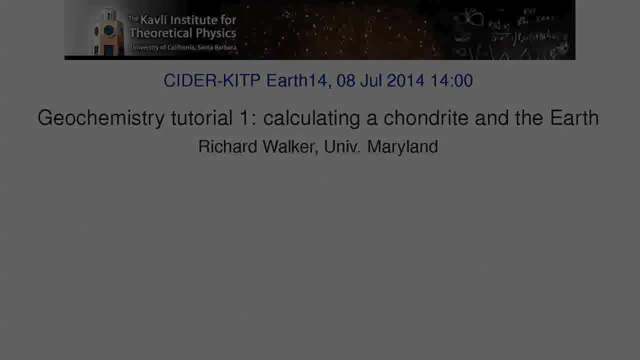 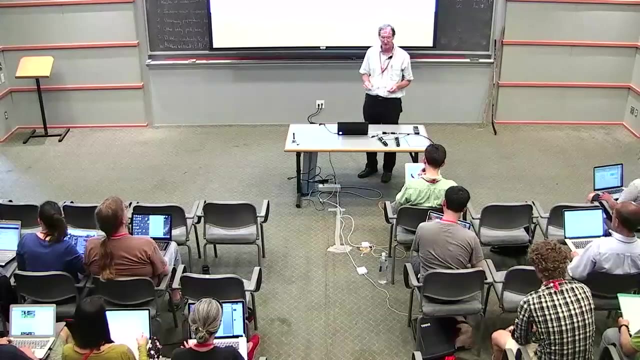 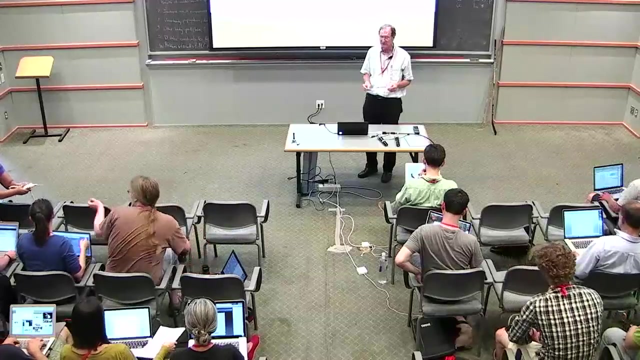 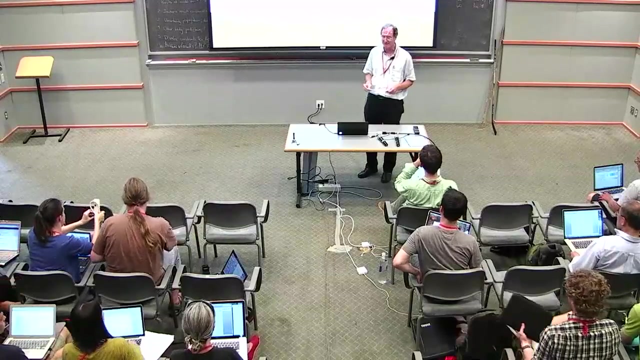 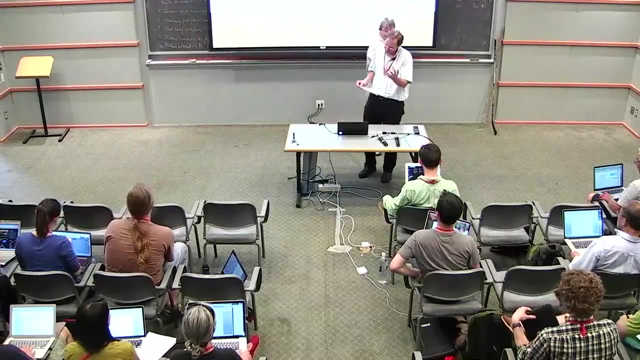 Okay, So first tutorial. I've never been to a CIDR tutorial, so I have no idea how this works, but we'll find out together. First thing to know is: the tutorial is not located on the virtual machine. You don't need a power cord, You only need a little bit of energy and your computer to do what we're going to do today. 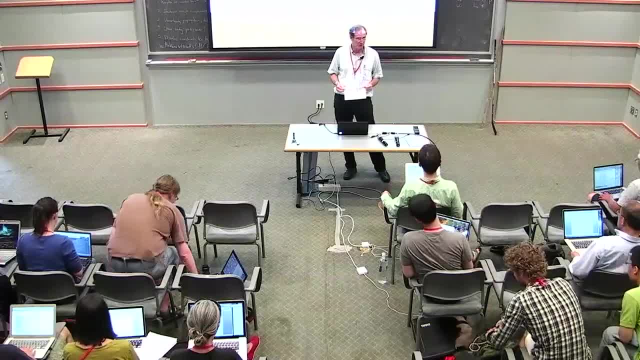 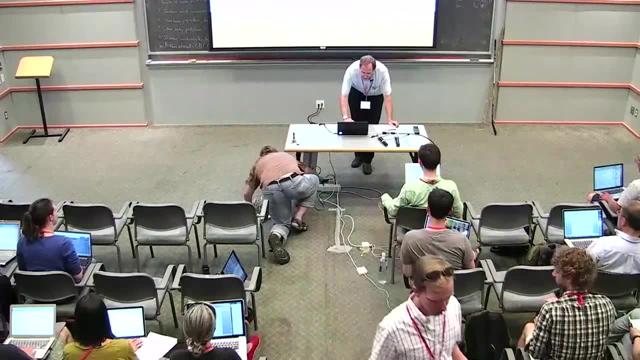 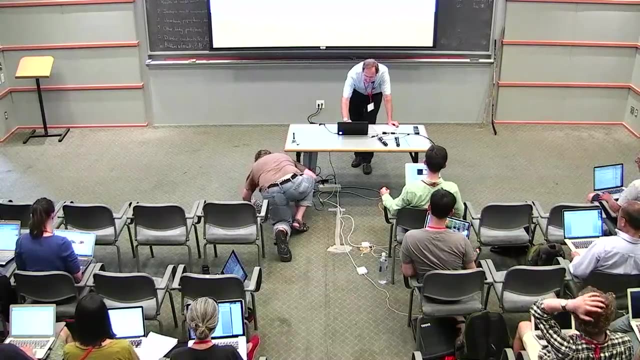 So this is not your first virtual machine tutorial. This will be simple. So how do you find what you need? What you need to do is go to the wiki page, which I will do for you. That's this one. Go to summer program. 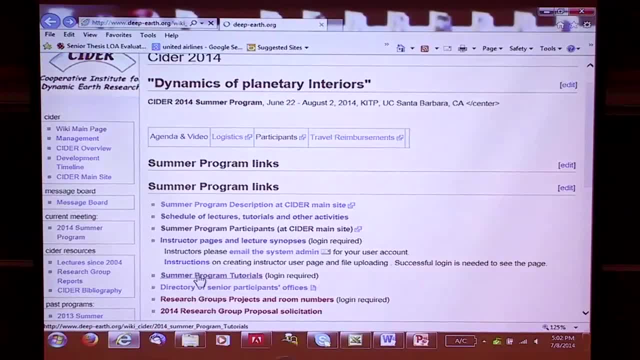 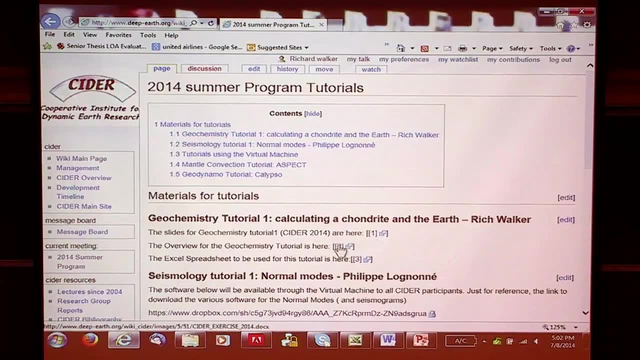 Tutorials: Click on that And under tutorial one you will see one, two and three And if you want the slides, you can click on one If you want a short word file that describes what we're going to do and some of the questions we're going to try to answer. 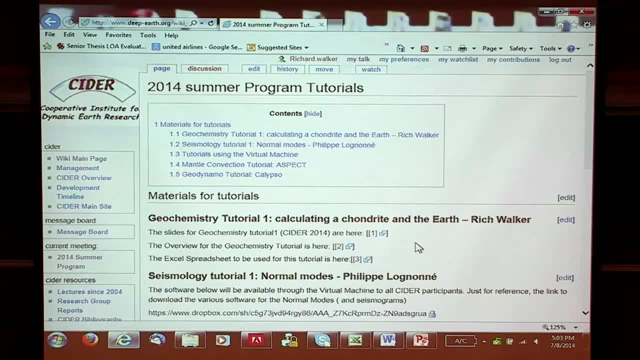 that's on two, but you don't actually even need that. What we're going to spend most of our time on is number three, which is an Excel spreadsheet. A simple Excel, a very simple Excel spreadsheet. How many of you have ever done anything with Excel? 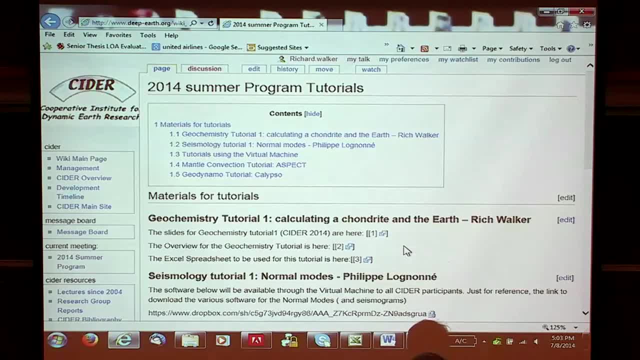 It's not as bad as you said. You said no one was going to know how to work with Excel. Okay, that's good. So does everybody know how to find the files? Tutorial 2014.. Actually, how do you get there? 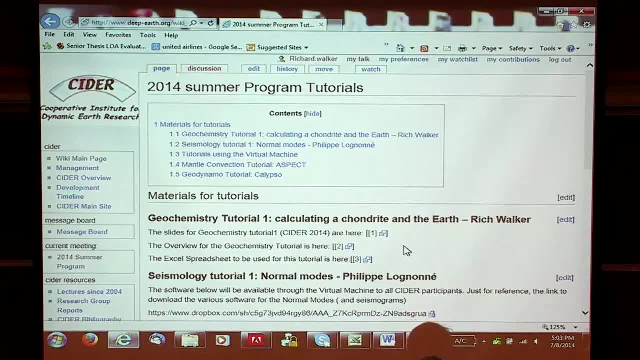 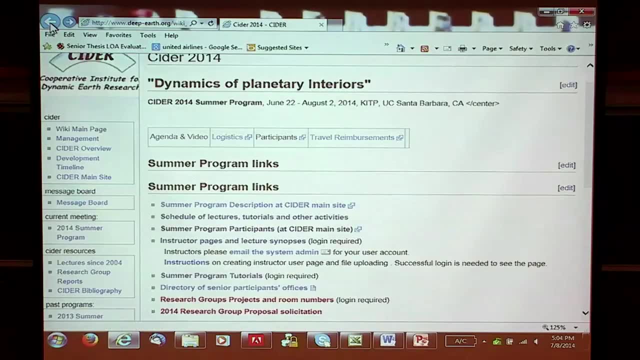 Oh man, All hope is already lost Because the wiki is ordered really bizarrely, Sorry. Yeah. Yeah, you can log in with that. The login is up there And if Luis is here, this should not crash the system. 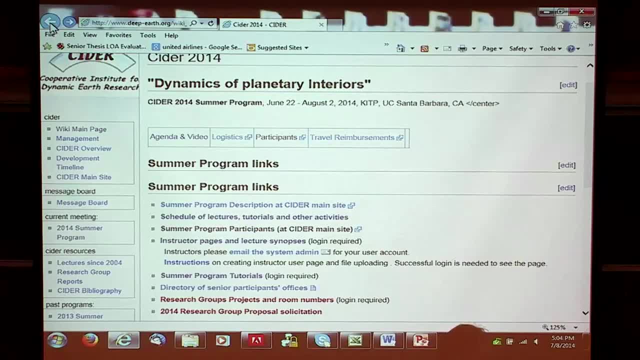 If everyone tries to download, this should not crash the system. We're going to have to do this all at one time because it's not a very big file. Okay, Are we good Questions? No, You have a problem with everything, though. 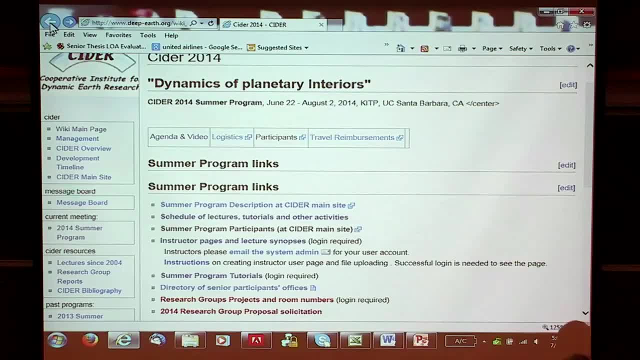 Come on If you want. it's like a treasure trove of files. You can have all three if you want, Okay, Okay, Treasure trove, Treasure trove. All right, We're again. I've never been involved in a CIDR tutorial. 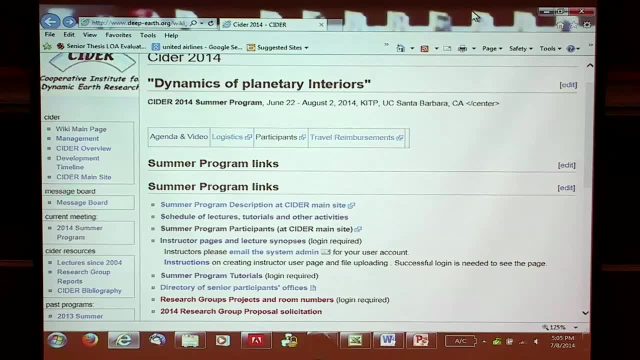 I've been told that it sometimes is good to break the students plus postdocs into groups and ignore the instructors. so we will do that. And I've also been told, and I know from experience, that scientists do not self-organize very well. 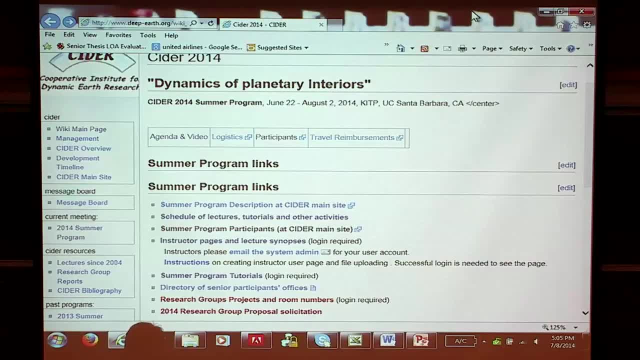 So we're going to go to the third grade. This is the third grade phys ed method and I'm going to request that every student or postdoc in here count off One, two, three, four, five, Start over here somewhere. 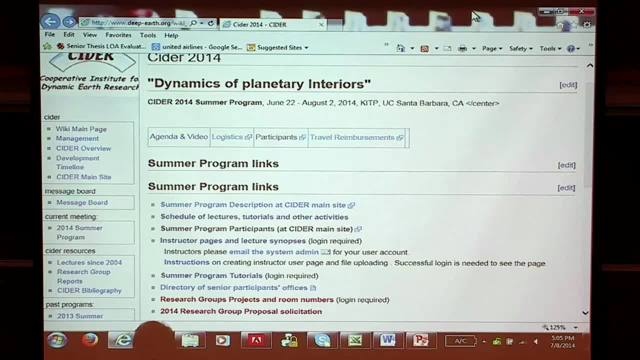 Senior people forget it. No, you can glom on to whatever looks like the best group, But if you're a student or postdoc, please count off One, two And remember your number. And remember your number One. Come on, come on, we haven't got all day. 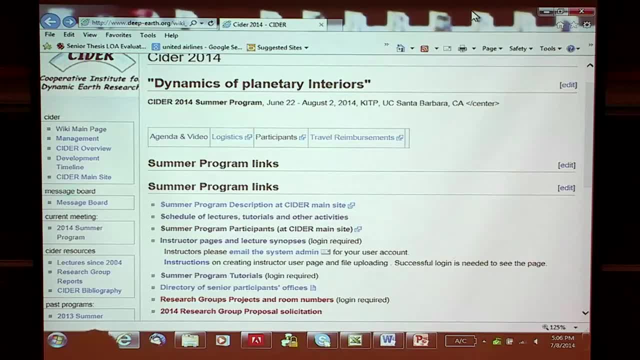 Bruce killed it. he died, but Bruce, What happened? This is too complicated an exercise. This is even worse than I thought. All right, start here. 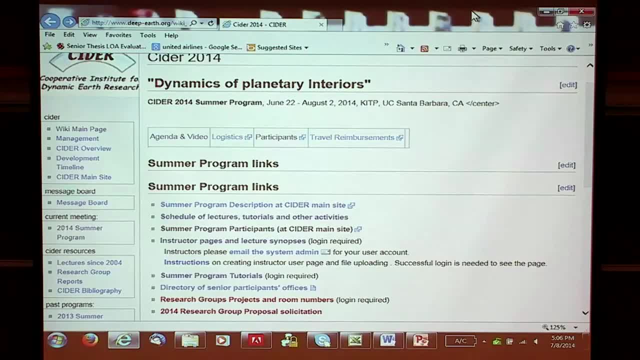 One, two, three, four, five, Five, one, Five. Do I have a one? One, two, three, four, five, glom two. 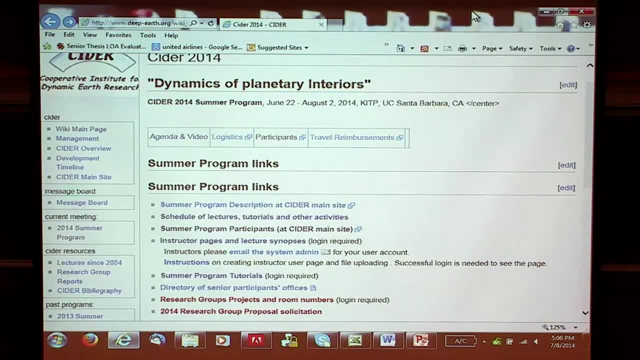 If he wants to be a student, he can. Are we there? Okay, are we good? Okay, good. Did you not get one? 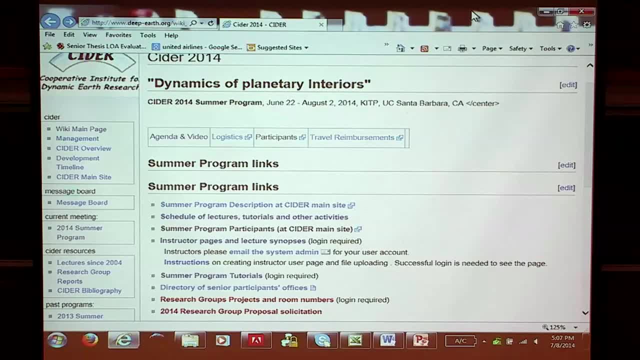 Pick a number, Okay, and you're now locked into that group for the next four weeks. No, Okay. so what I'm going to do is hopefully give you a brief overview of today's topic, And today's topic as it turns out. 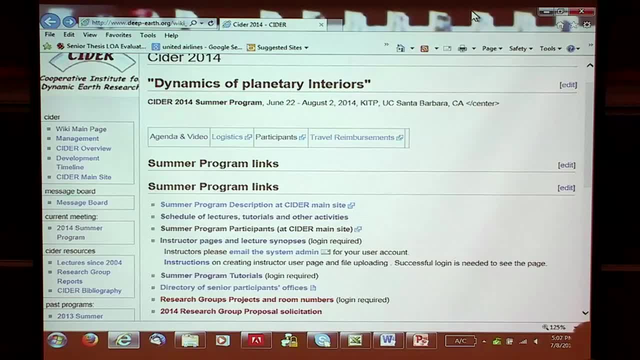 is nothing like what was written on the website. It is, but it's similar. It's building a chondritic planet and then segregating so-called siderophile elements into the core and mantle and learning what that may tell us about how the Earth put itself together. 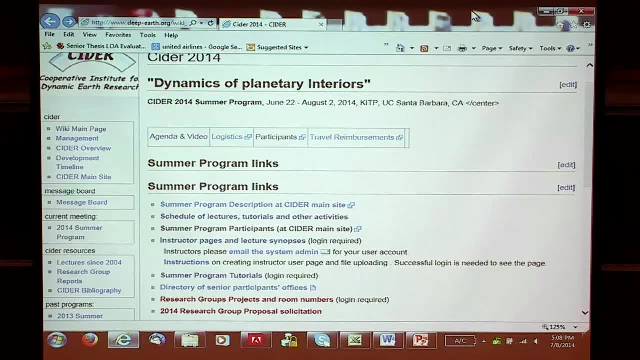 So we're going to be looking at measured concentrations of some elements, We're going to be using some real distribution coefficients And we're going to do a very, very simple model of core segregation that is kind of consistent with what some people believe. 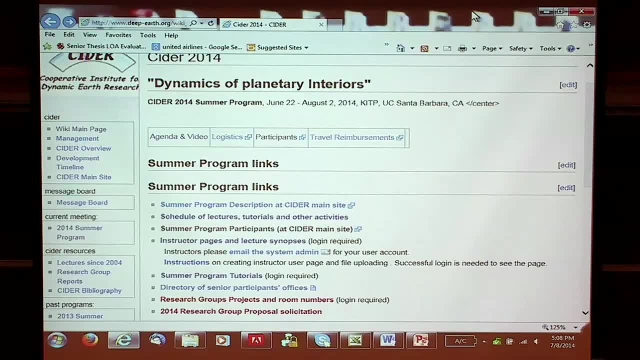 And we'll see what we get And we'll look and try to assess what the strongest constraints on the process are and whether or not any of the inputs that we put into the spreadsheet actually yield a viable model. And I'll forewarn you: 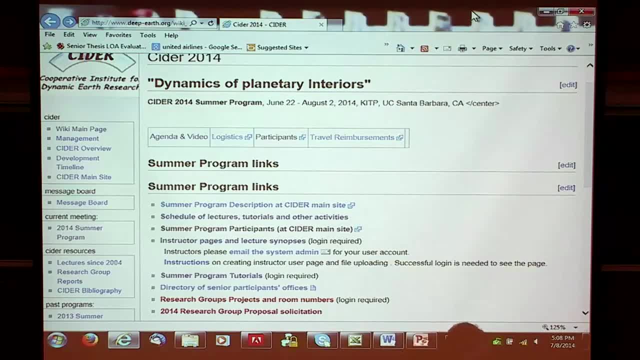 actually none of the conditions that I'm going to give you the data for are actually going to work perfectly. I'm really, believe it or not, not trying to set up a straw man and convince you that this can't possibly work, because at the end of this exercise, 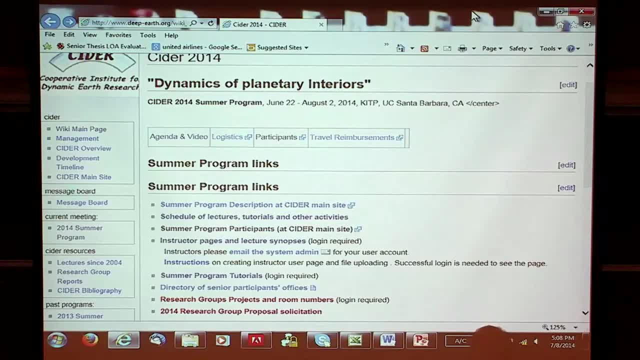 we want to consider all the things we don't know and still need to be done with regard to models like this. So we're not going to be entirely satisfied at the end of this tutorial, but the final question that I have written on the board is: 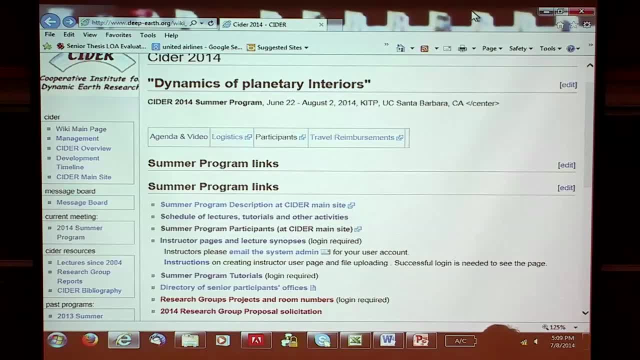 where would you go from here if you were an experimentalist and you wanted to proceed further on this issue? Ved, My question is that when I try to download your files, it says zero KB of question mark. you do not have permission to access the requested resource. 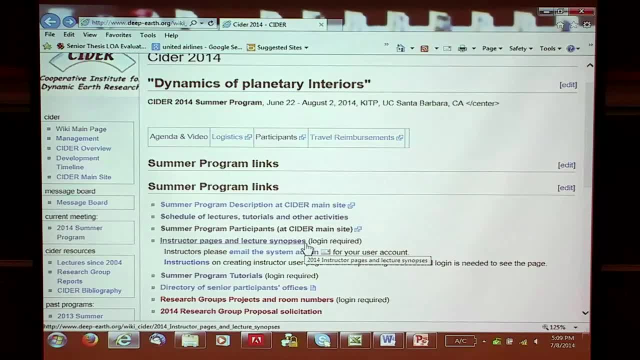 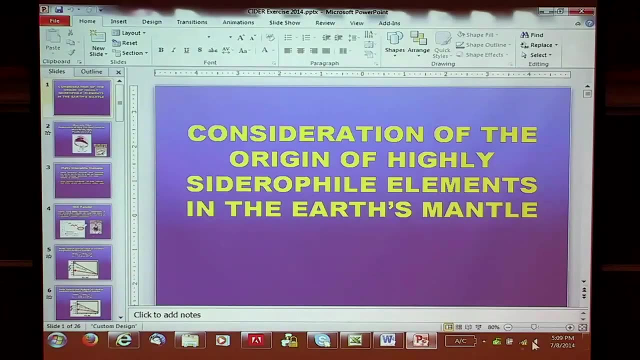 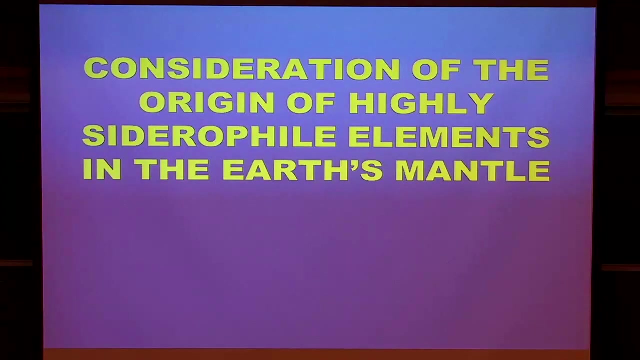 Did anybody else have this problem, or is it just? It's really designed to block you? Okay, So the bottom line: too bad, Get with a group that knows what it's doing, okay, Okay. So the topic: consideration of the origin. 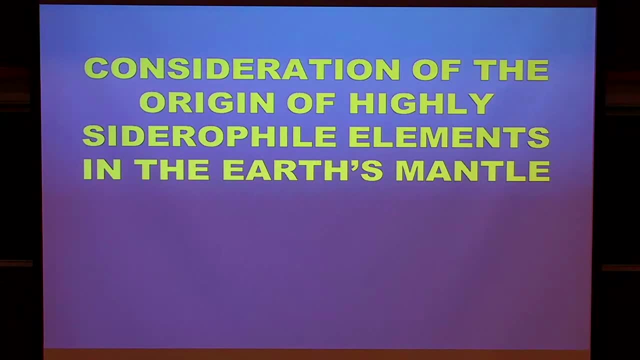 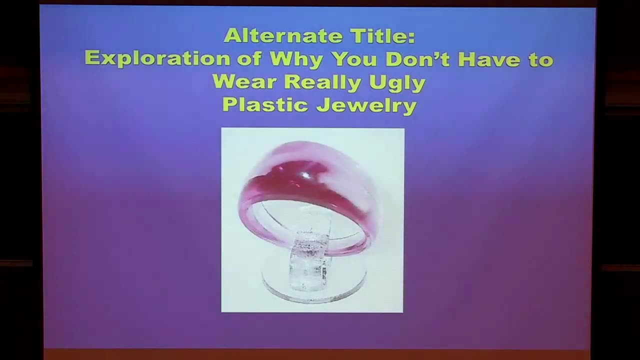 of highly siderophile elements in Earth's mantle, and I have an alternate title which is more visceral, and that is exploration of why you don't have to wear hideously ugly plastic jewelry and can instead wear shiny gold. You can wear gold if you want to. 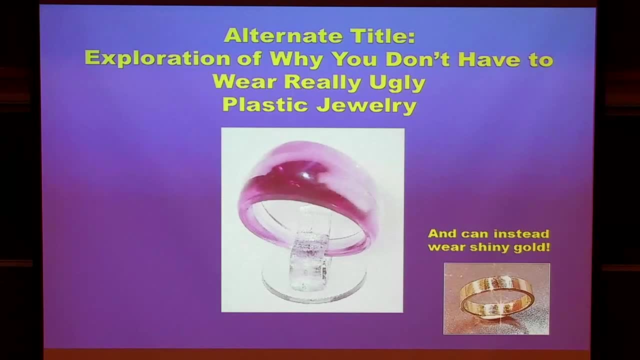 And I say this with a little bit of a trite nature, but really, if the Earth didn't perform the way that it did with regard to this suite of elements, you could very well be living in a society that doesn't have much in the line of highly siderophile elements. 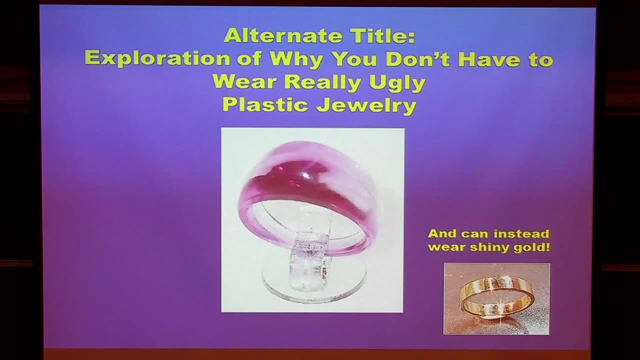 Gold you could envision could be easily a thousand times less prevalent here in the crust where we can mine it, than it actually is, And if that were the case, humans probably wouldn't be wearing gold jewelry, and they may not be as technically advanced. 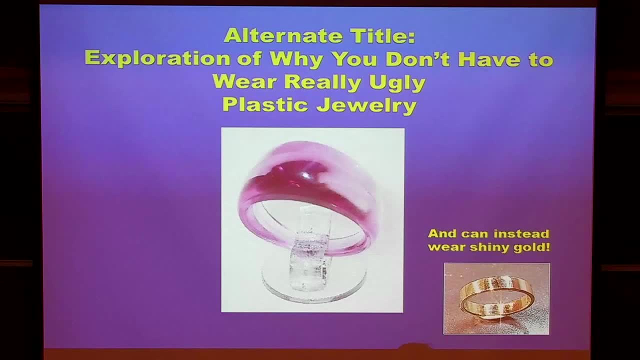 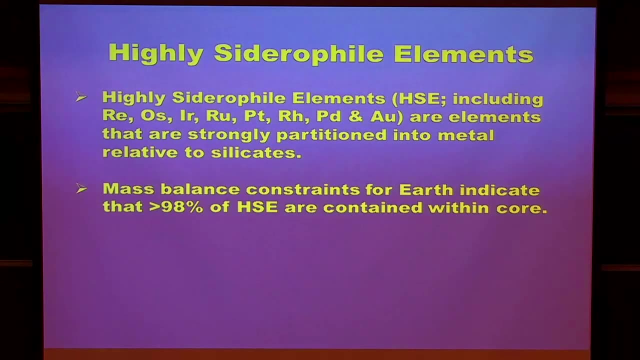 as we think we are. So just a little bit of practicality to this. Okay, So I'm going to be talking about highly siderophile elements. This is a little bit of a chicken and the egg type question. I'm going to also talk a bit about this on Saturday. 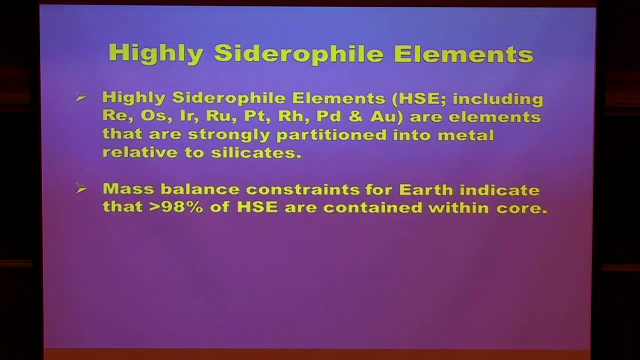 So this might have worked a little bit better after the primary lecture, but this will aid us on Saturday as well, So let's get started. The highly siderophile elements, which I may say HSE- sorry- include this suite of elements. 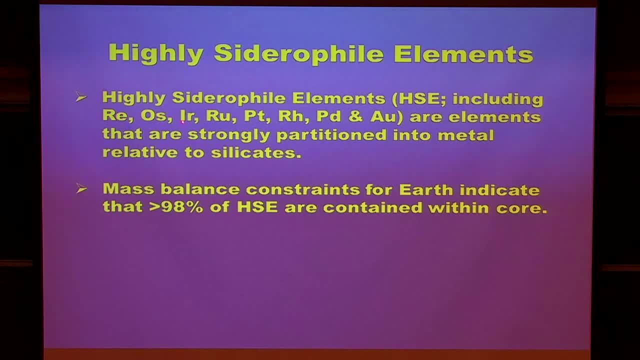 Let's just go through them: Rhenium, osmium, iridium, ruthenium, platinum, rhodium, palladium and gold. You've certainly heard of some of those. You may not have heard of some other ones. 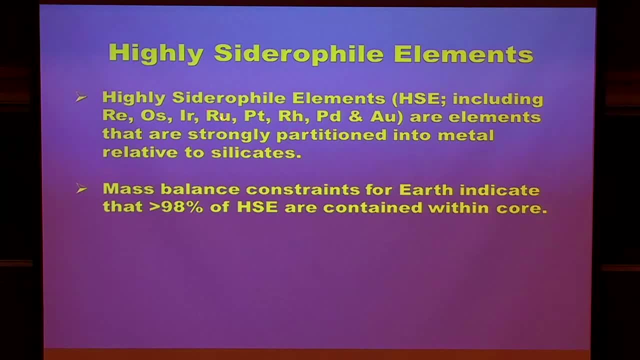 This is rhodium. This is ruthenium. He's not very good with element abbreviations, But we can work through that. And the term highly siderophile means these are elements that are really really strongly partitioned into metal. So where are these elements located in this planet? 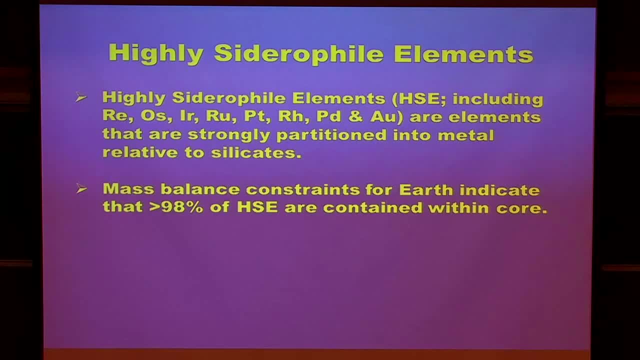 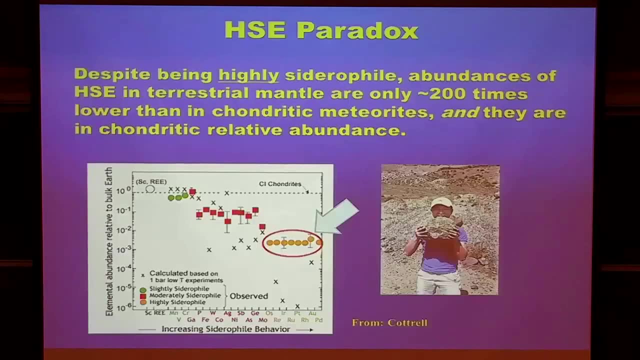 By and large, about 98% of the Earth's highly siderophile elements are sitting in the core right now. Okay, So this is the paradox, the problem that's involved with highly siderophile elements. This is a beautiful diagram that Liz Cottrell created. 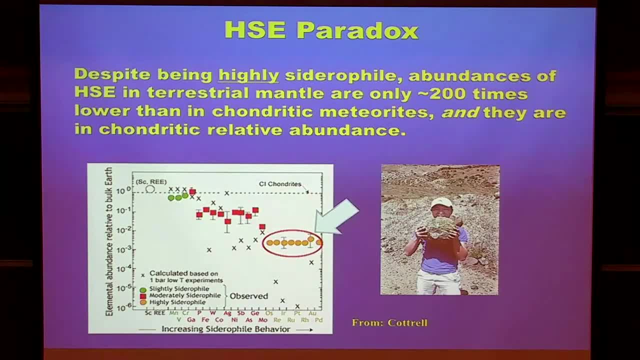 I liked it because it's got so much color in it compared to other published figures. But there's lots of figures like this, Just to be clear. yes, okay, This is a plot of a bunch of elements that increase in their siderophile element behavior. 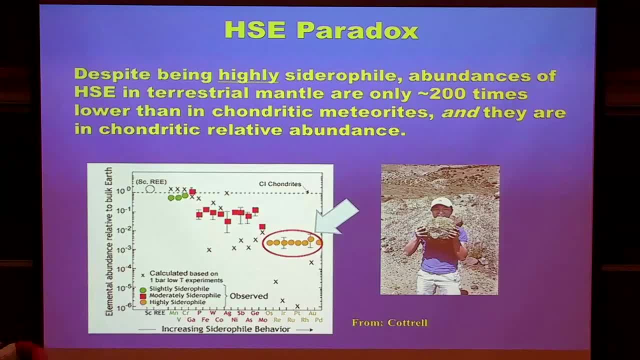 from left to right And it's a multi-log plot, And their abundances in the mantle are ratioed here or compared here with C1 chondrites, which we'll also treat as bulk Earth here, And so the red symbols we'll talk more about on Saturday. 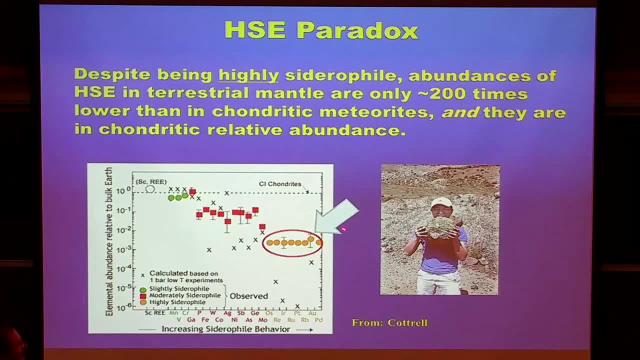 They are the so-called moderately siderophile elements, And it's the orange ones that we're considering here today. And the thing to note about them, they are about 200 times lower abundance than they are than a typical chondritic meteorite. 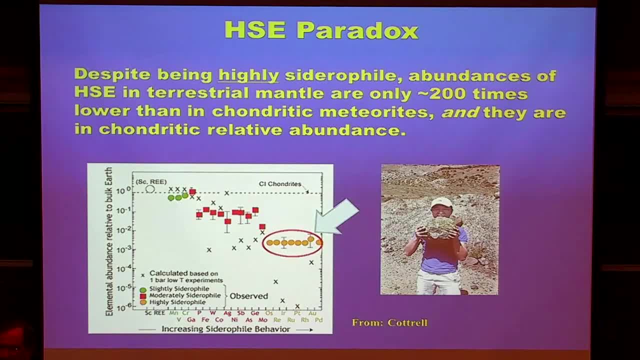 And that sounds like they are in low abundance, And they are Typical. concentration of a highly siderophile element in the mantle is low part per billion or nanogram per gram concentration range. Interesting thing about them, though, is if you go into an experimental lab. 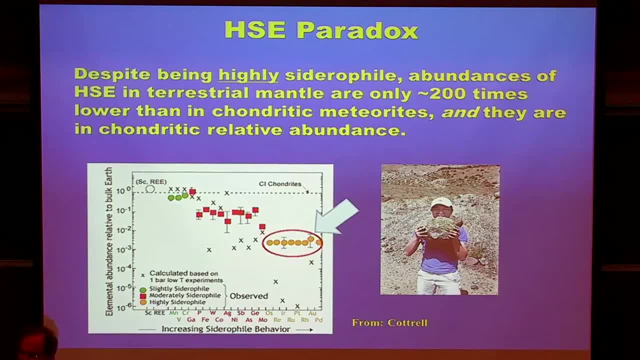 and you throw some metal into some silicate and you examine the partitioning of one of these trace elements between the metal and the silicate under, let's say, one-atmosphere conditions, as people were doing 50, 60 years ago. 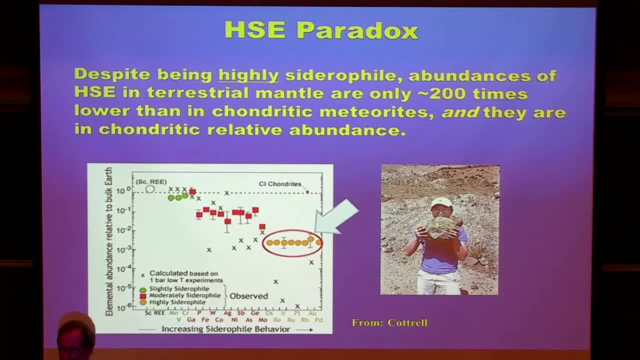 you would find very, very, very low concentrations in the silicate portion of the experiment. the silicate And these Xs in figures like this always represent what the concentration would be if partitioning was like we see under low-pressure conditions. And so the paradox, the problem here. 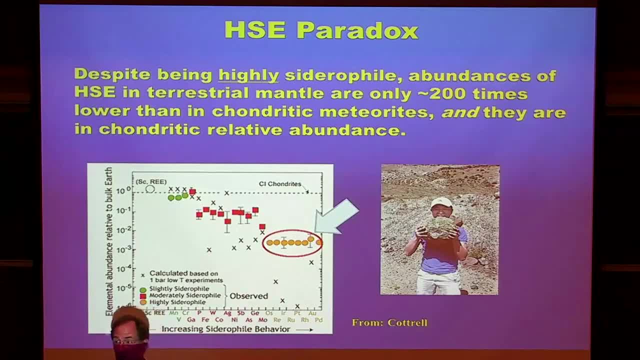 is that the abundances of the highly siderophile element by and large are much higher than we would expect from low-pressure, relatively low-temperature metal-silicate partitioning. Okay, And this has been known since the 1950s and 1960s. 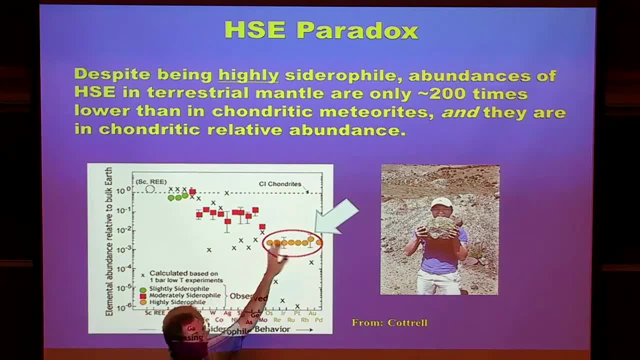 Now, how do we know the abundances? Well, this is a planet that, as you know, allows us to physically access bits of the mantle- And yes, this is not Liz, but this is a guy holding a big peridotite zenolith. 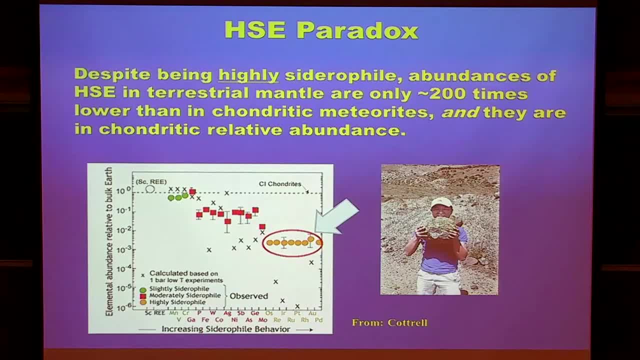 from the North China Craton, And so we can go to rocks like that and we can grind them up and we can analyze them. And you know what? Bill White gave a talk yesterday discussing the bulk composition of the Earth and some of the controversies. 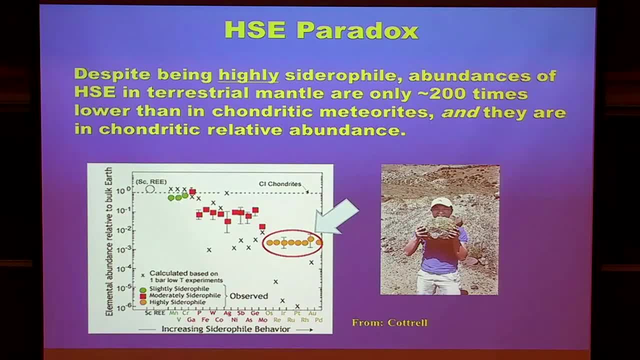 in terms of the major element composition of the bulk Earth, There's really not a whole lot of controversy about these abundances. Now, if we got together a group of geochemists that are really only interested in highly siderophile elements, there would be a lot of nitpicking. 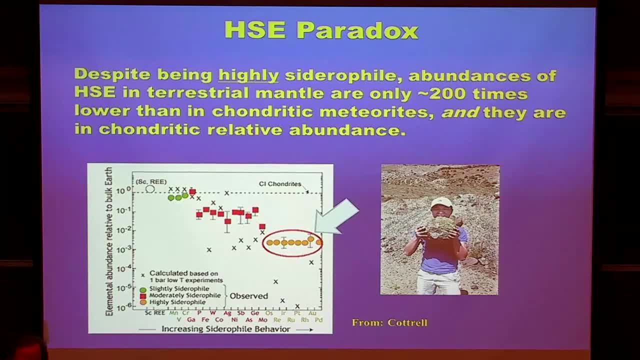 about the absolute abundances in the mantle, But by and large nobody- Do you agree with this, Liz? Nobody really argues these approximate abundances. So this is a set of elements for which we're pretty confident. we know the abundances in at least the upper mantle. 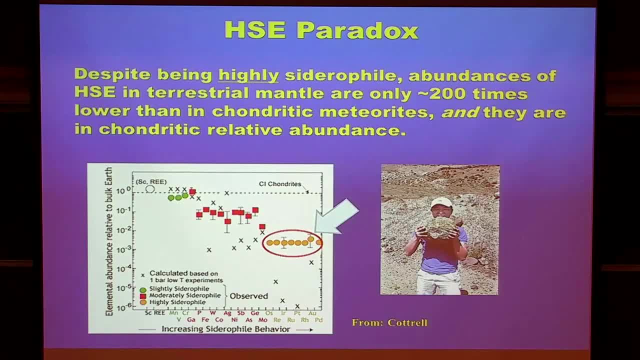 And if the upper mantle is reasonably well mixed with the lower mantle, we're good to go. I should also point out, in contrast to some of the isotope systems that Bill was talking about yesterday, Bill White was talking about, these are elements that don't like to go into continental crust. 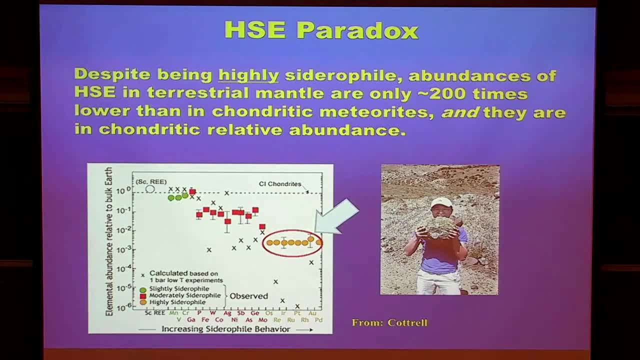 and therefore we don't even have to worry much about the effects of continental crustal production. So mass balance, these elements are pretty well understood. Ah, there's one other thing that this figure shows, and that is they all plot along kind of a horizontal line. 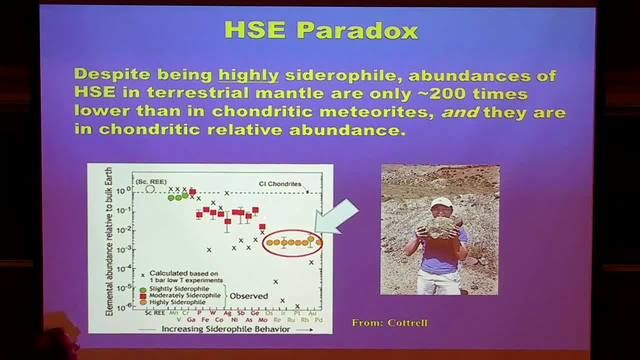 which you notice is kind of the case, but not totally the case for moderately siderophile elements. So that has to be explained by whatever process generated their abundances in the mantle. That's my question. It looks so suspicious. Also, why do some of them have error bars in other elements? 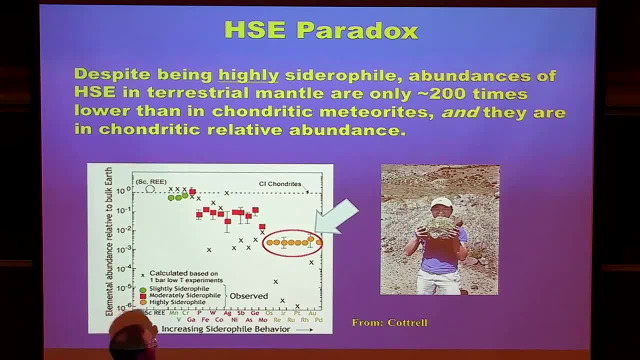 And what are the error bars representing? The error bars represent uncertainties in projections to a bulk-silicate Earth composition, which I can get into, but you probably really don't want me getting into that. These are tightened up since Liz generated that figure. 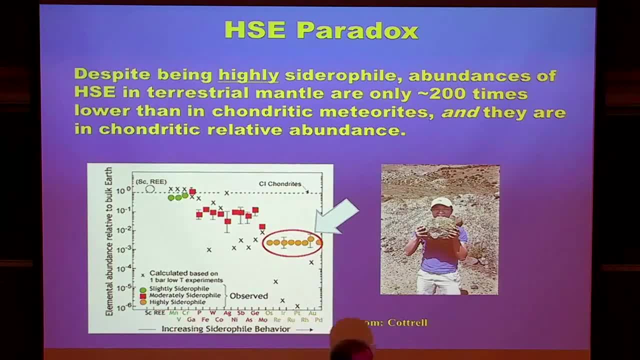 so I think we know them better than you. Even the size of the dot on there, that's a long scale, so the size of the dot gives you a good factor of two. Yeah, in the spreadsheet that you can download, as I'll go to in a minute or two, 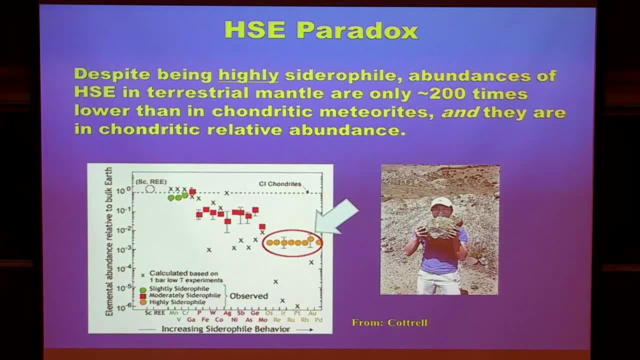 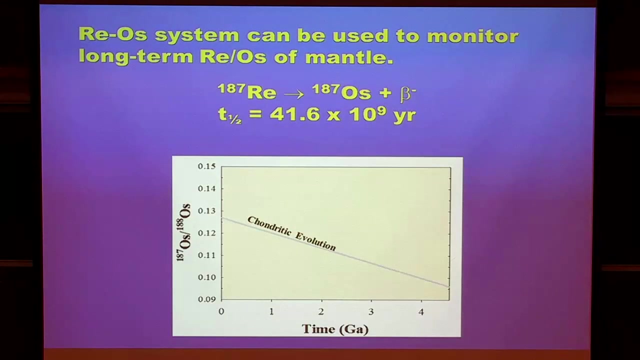 you'll see a bulk-silicate Earth composition which, again, there would be some minor nitpicking within the geochemical community, but by and large it hasn't changed. It's not going to change Now, embedded within this suite of elements. 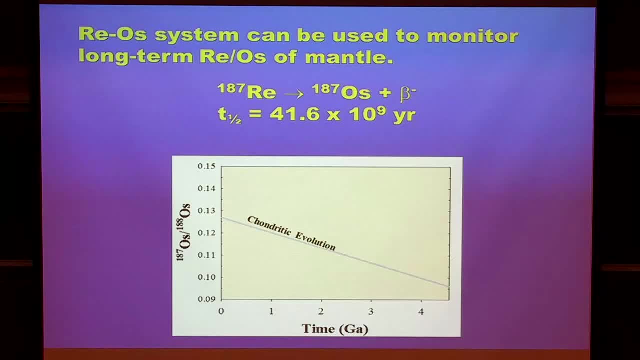 are two radiogenic isotope systems- and we're going to work with those a bit today- And one is one of my favorites, which is based on the decay of rhenium-187 to osmium-187.. Both of these elements are highly suitable. 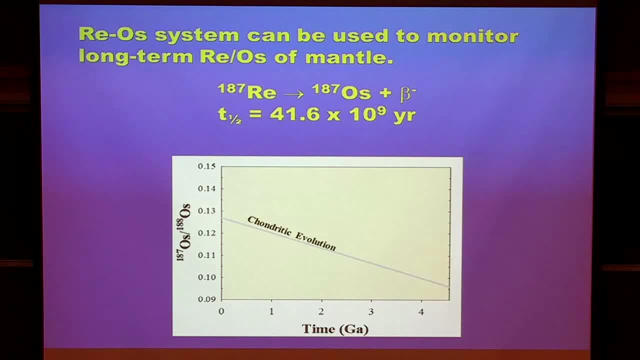 as siderophile elements. so they were among the orange symbols there And this is how we believe the mantle has evolved. There is finite uncertainty in chondritic evolution. We can talk about that later on, but by and large, what we're going to look at- 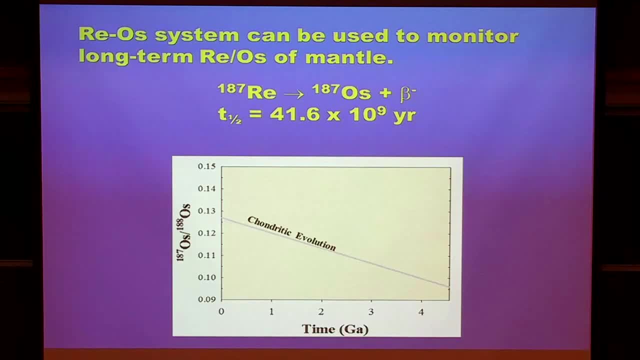 in our calculations later on. if this were to actually work, There we go. You know, if we fractionate, vary the rhenium-osmium ratio within the mantle by even a small amount, long, long ago, when these elements were placed into the mantle. 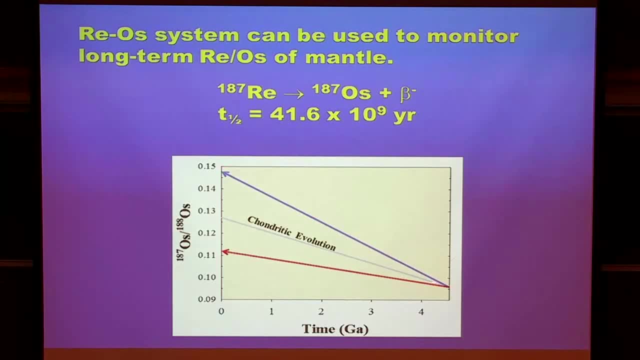 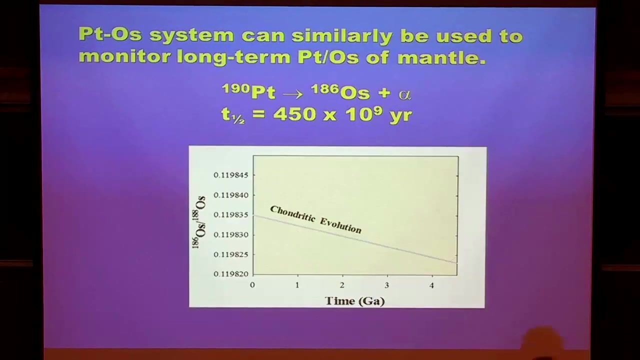 we might get evolution along a trajectory like this or like this, And we will see differences, therefore, in the modern-day isotopic composition that we project from the models that we're going to run today. Okay, We have one other system, which is a nightmare system in some ways. 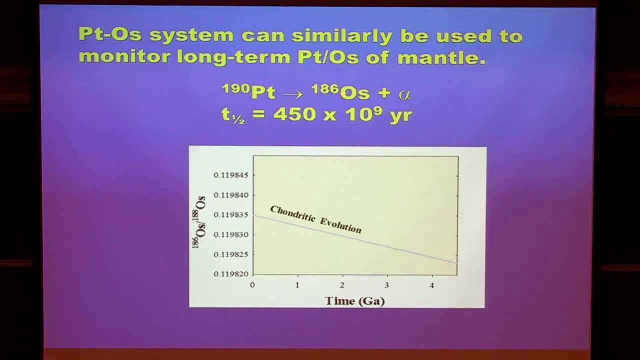 It's platinum-190 decays to osmium-186.. It's an alpha decay system. It has a- Oh, I didn't say it before, but the rhenium-187 has a half-life of about 42 billion years. 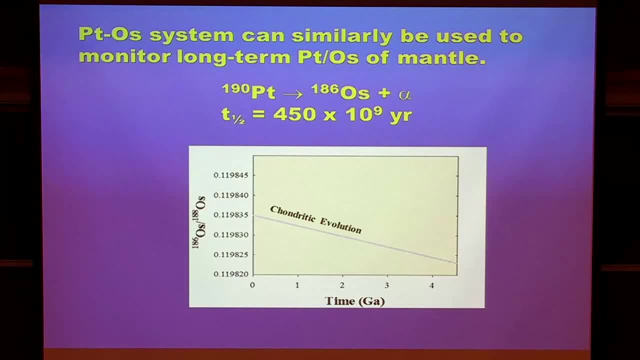 This system has a half-life of 450 billion years, and the parent isotope is a very minor isotope, And so this is a isotope system that is exceedingly sluggish It. You can see. we've got several more significant figures here. 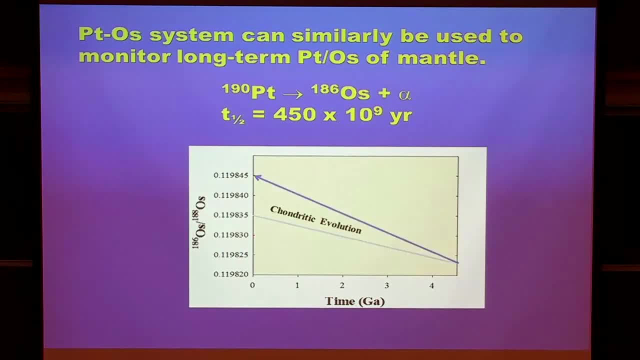 and we can do the same thing and see if the ratio in the mantle is actually higher than chondritic, it might evolve up that way. If it's lower than chondritic, it might evolve off that way, And so we'll do that. 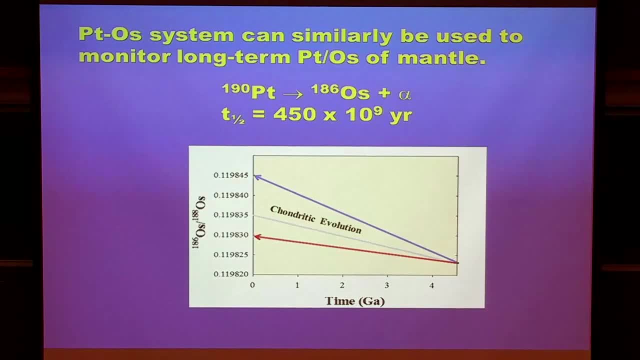 And the good news is in the spreadsheet I did all the calculations for you, So you only have to think about the results. You don't have to deal with the Excel spreadsheet other than putting a few numbers in in case you're getting worried. 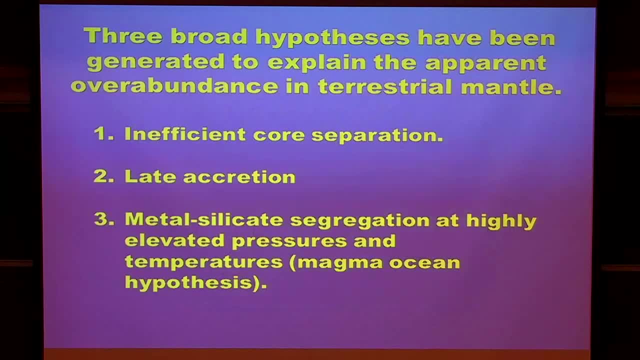 Are you getting worried? No, I still haven't downloaded it. Oh, dear, dear, dear. Okay. Well, while Ved continues to work, I can give it to you on a disk, Anyway. so how did these elements get into the mantle? 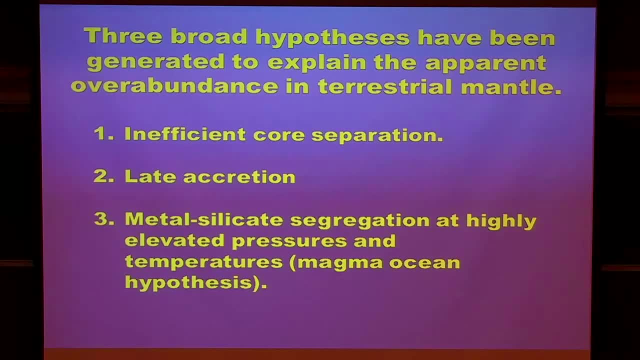 That is the question that we want to address in part today. Over the years there have been three broad hypotheses tendered to explain the abundances of the highly siderophile elements. why those orange symbols plot where they do on that diagram? And one of them has been termed: 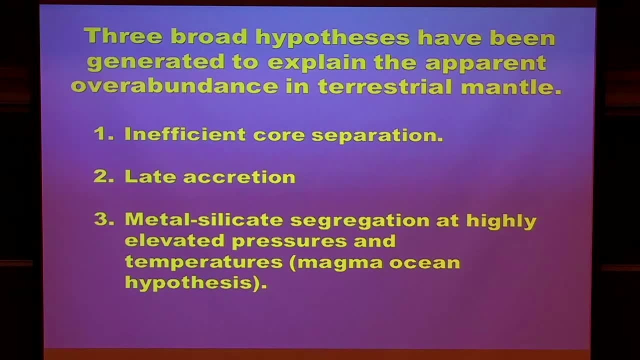 inefficient core separation, which I'll show you what it is in just a second. but it's just what it sounds like: Segregate a core but leave some of the metal behind. Number two, a process called late accretion. 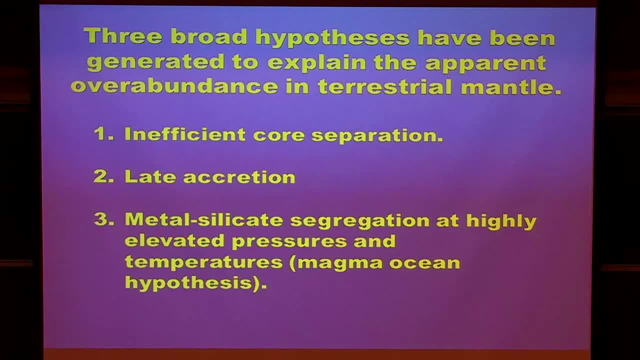 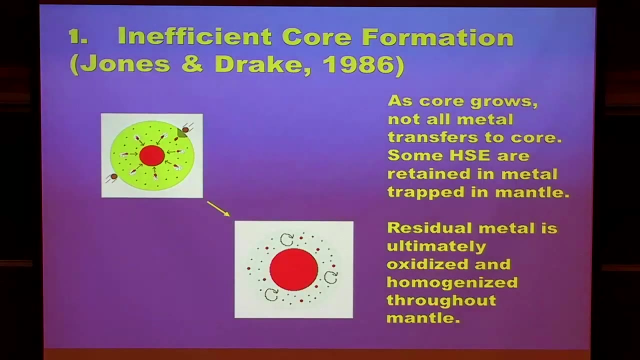 And number three. what we're going to be considering today is metal silicate segregation at highly elevated pressures and temperatures. Some people call it magma ocean hypothesis. Okay, So the idea of inefficient core formation is: you're building a planet, you're adding stuff, perhaps 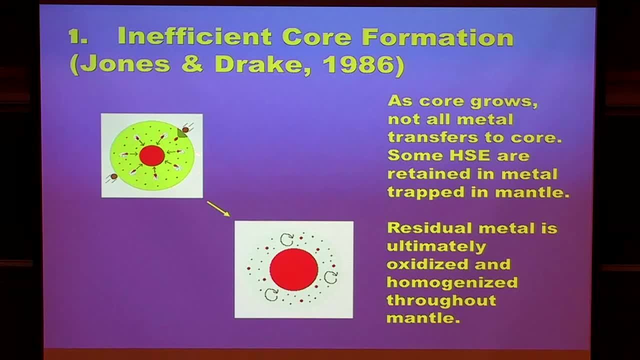 to a partially differentiated body. Some of the metal which is shown here as little rings, little red droplets, may stick around in the mantle. That doesn't look too good here, but ultimately you end segregation of metal from the mantle and you've left some portion of metal behind. 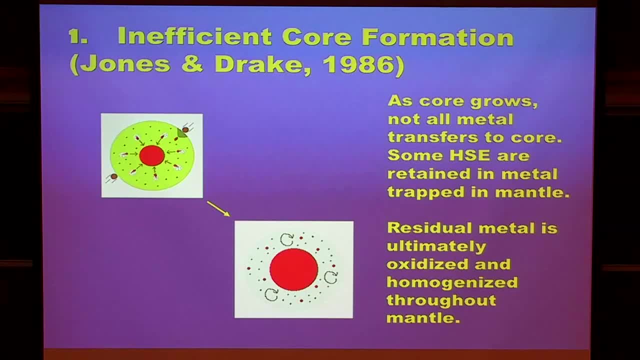 and ultimately for it to end up looking like the mantle today. you've got to oxidize part of it and make the metal go away. Any problems with that idea? This idea was kind of generated maybe 30 to 40 years ago. It was before people were thinking. 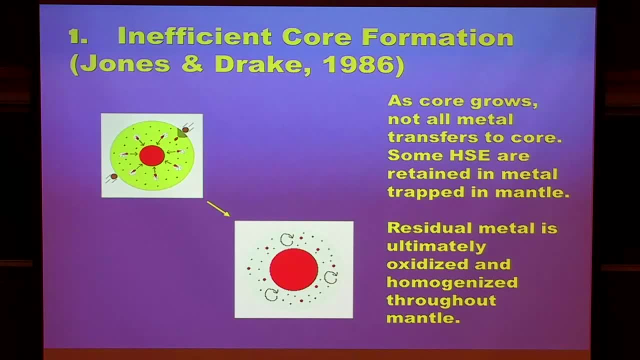 much in terms of magma oceans. This is a model that I think still has some utility, but it's hard to envision much metal sticking around in a planet that is periodically experiencing magma oceans. So not much has been done with inefficient core formation in about three decades. 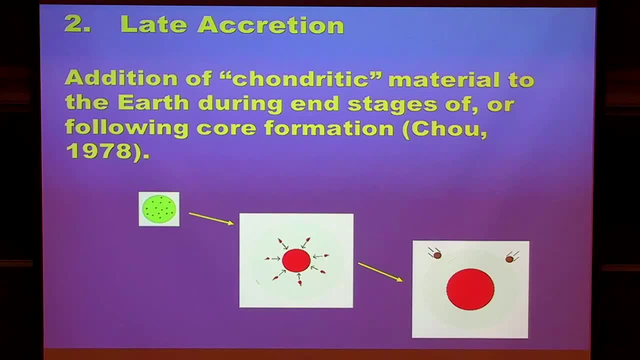 The second idea, which I'll talk more about on Saturday and is my favorite candidate, but it's by no means proven- is late accretion, And that's a concept where you form the earth, you segregate the core. At some point, core segregation ends. 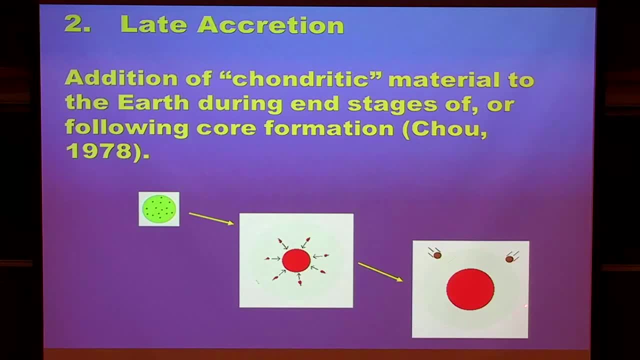 These just didn't come out very well in projection here. And then you add some chondritic material to the silicate portion of the earth, buffering up the concentrations of these elements and defining the mantle then as having chondritic relative abundance of magma. 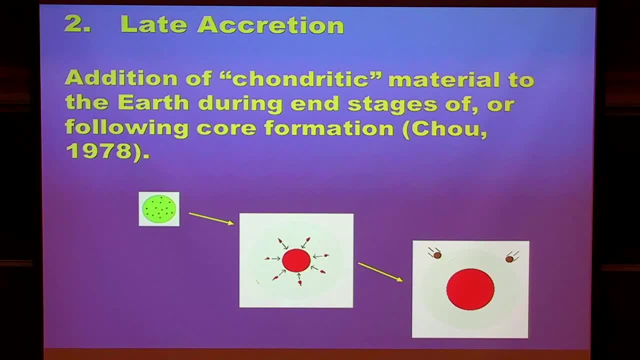 So that's one of the differences of these elements. The idea is, if you're impacting differentiated bodies, none of the metal from those get into the core and they have the same problem that the inefficient core segregation model has, which is you have to ultimately oxidize. 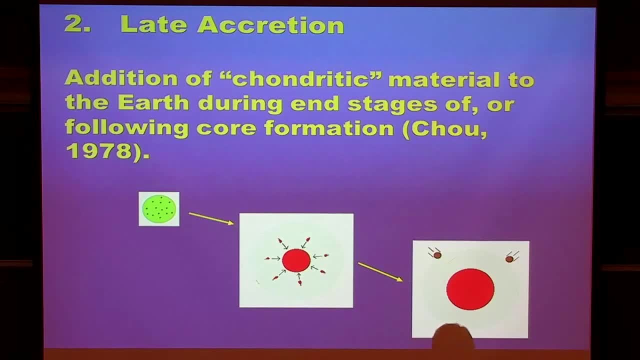 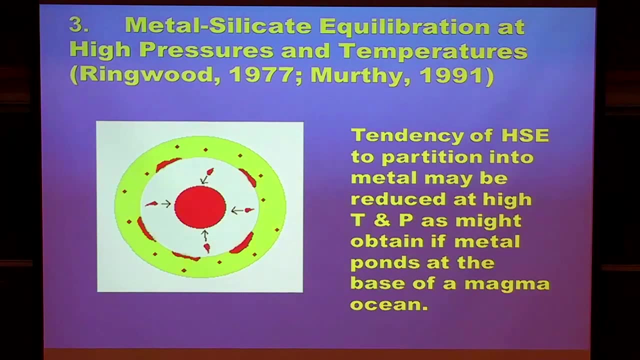 the metal, to have it go away, Because we don't find metal in the mantle today, right, Good, okay. And what we're going to consider today is a lively topic of conversation in the community, and that is metal-silicate equilibration. 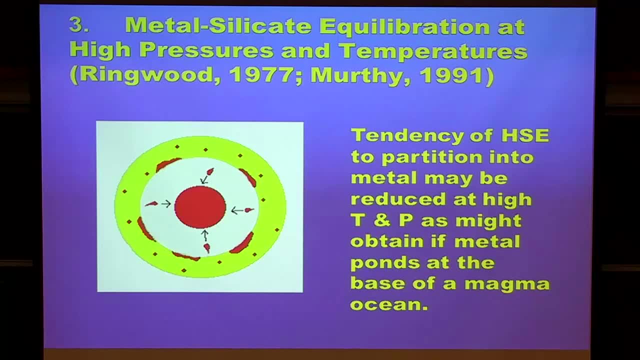 at high pressures and temperatures. I'm not going to say much about it today, but I think it's relatively safe to say that the community that works on these issues generally agrees that the moderately siderophile elements, the red elements in the earlier slide. 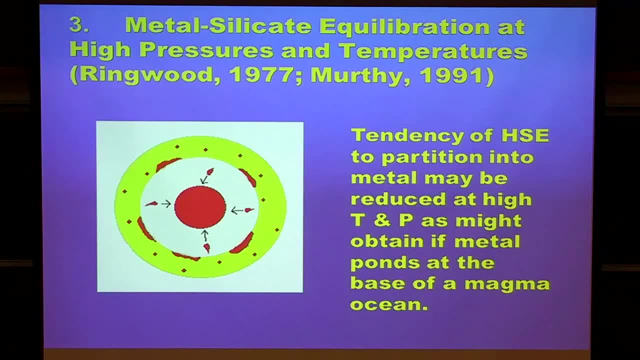 were probably set by a process like this, And Bill mentioned this as well yesterday. So the idea is you have a body that is segregating a core, but you may have a molten exterior, a magma ocean, and you might have pooling of metal. 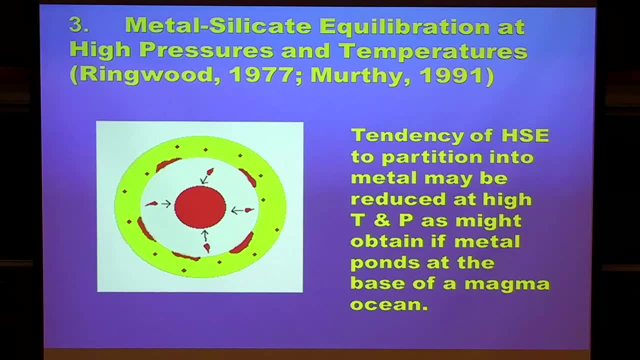 at the bottom of the magma ocean And the idea is, at these depths you're doing the equilibration between the metal and the silicate and that's what defines the final abundance of these elements in the silicate portion of the planet. 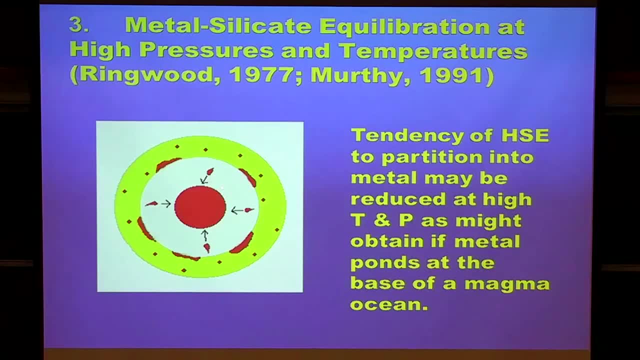 The metal ultimately drops diopyrically through a solidified lower mantle into the core. Okay, So again to reiterate: people generally agree they have different models, but geochemical world that works on this generally agrees that the moderately siderophile elements were established. 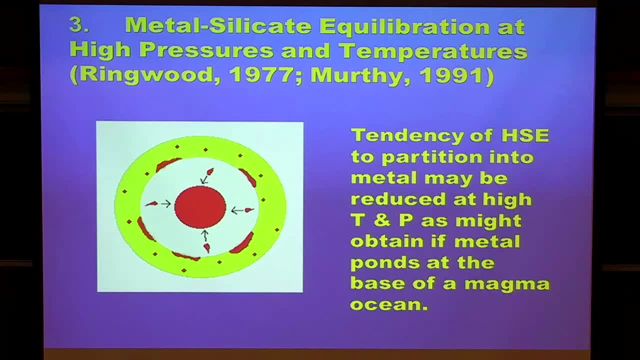 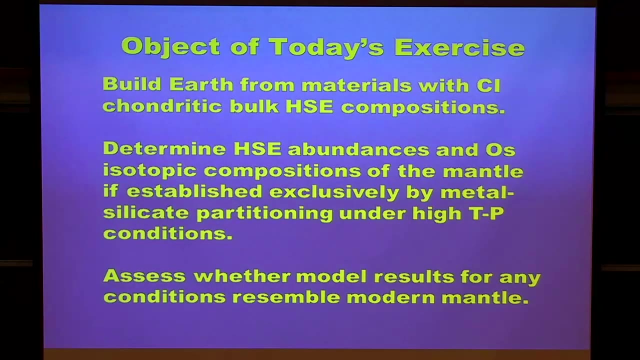 by this process. So it's not probably as simple as this. The Earth perhaps went through multiple magma ocean stages, but some average pressure and temperature was probably established which ruled the partitioning. Okay, so what we're doing today? we're going to build Earth from materials. 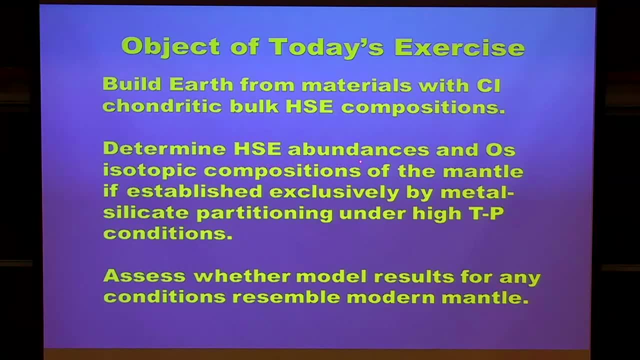 with C1 chondritic bulk composition. We're going to determine HSE abundances and osmium isotopic compositions of the mantle if they were established exclusively by metal silicate partitioning with high pressures and temperatures. Okay, We're also going to do a little bit. 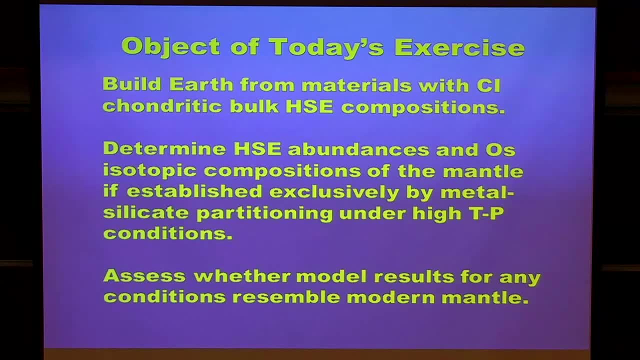 of varying of another factor, oxygen fugacity. but that just stems from the source of the distribution coefficient data that we'll be using, And so we're going to assess whether the model results for any conditions. resemble the modern mantle Again, I tell you. 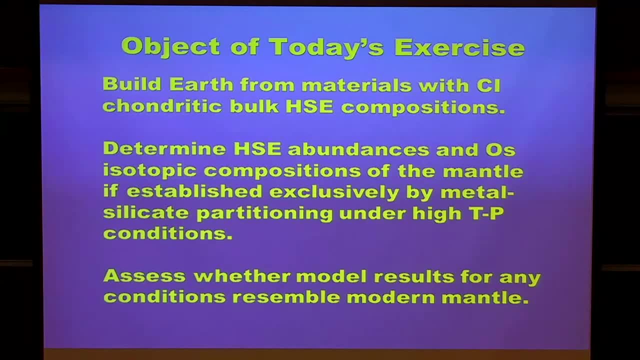 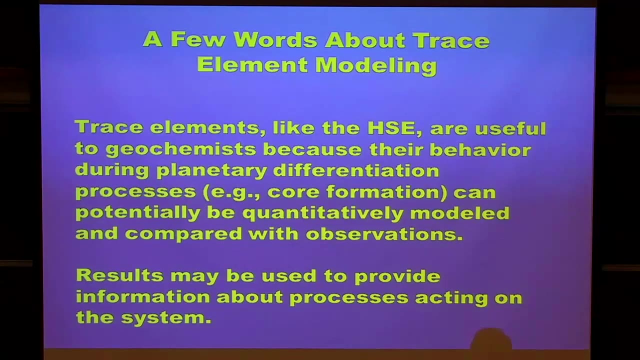 none of them are going to be perfect. Most of them don't come close, but it'll allow you to see what would have to change in order for this type of model to work. Okay, Okay, Bill White yesterday actually did most of the work here. 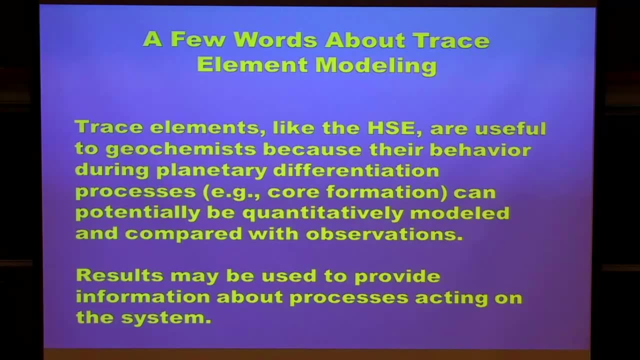 so a few words about trace element modeling. in the system we're about to deal with, The highly siderophile elements are to be treated as trace elements, and in many geological scenarios we can use measured distribution coefficients in order to quantitatively predict how these elements should partition. 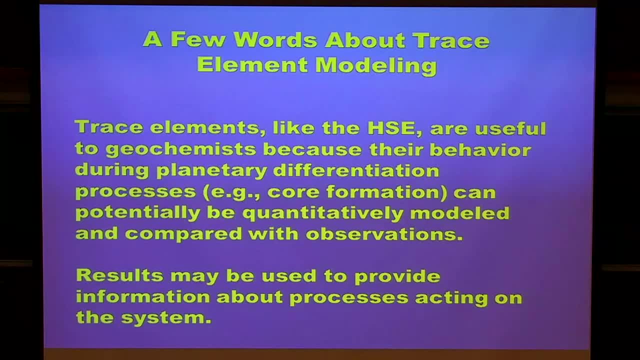 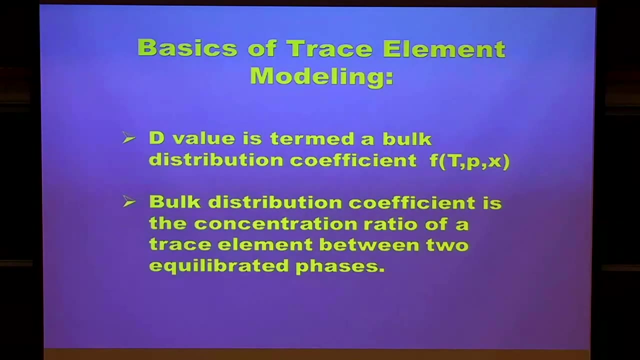 between different phases. In this case, our interest is in looking at the partitioning of this suite of trace elements between a molten silicate earth and metallic core material. Okay, And again, yesterday this term was defined a capital D. We're not going to go into differential equations here. 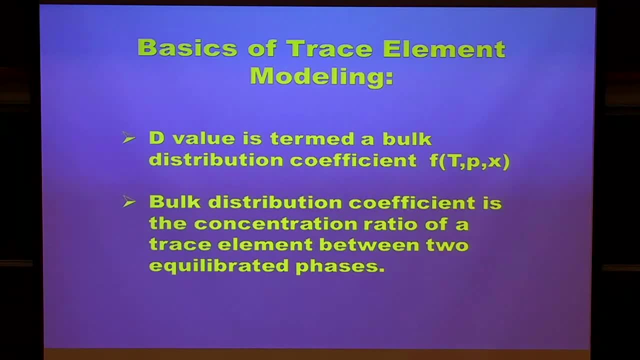 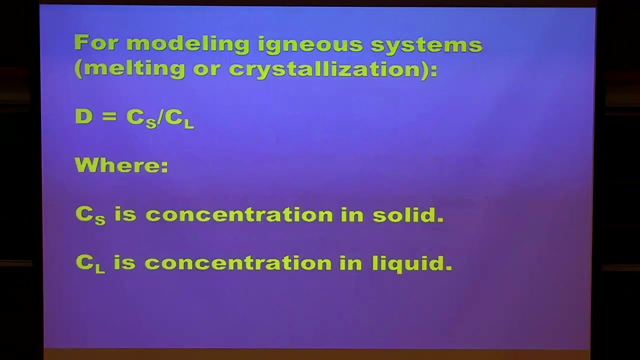 We have very simple equations: D is bulk distribution coefficient, and it is just simply a concentration ratio between two phases. In this case, the two phases again are metal and silicate, liquid metal and liquid silicate, And so here's the relation. 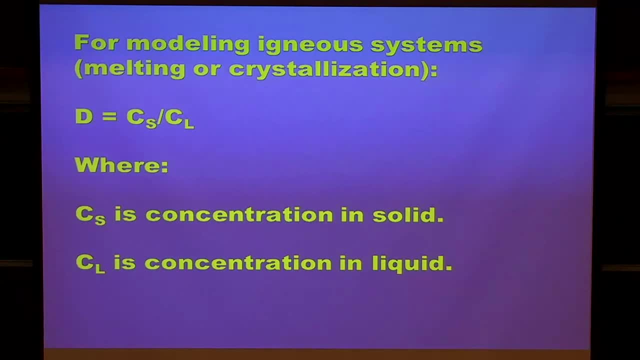 That's not too bad, right, Okay? And for this case, what you're normally treated to in a textbook would normally be presented like Bill presented it yesterday, where we have C sub S is the concentration in the solid and C sub L is the concentration in the liquid. 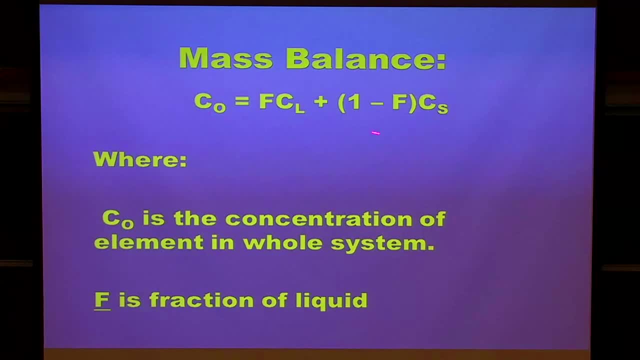 And then you go into a mass balance calculation or equation like this which Bill showed you yesterday: The C sub O, in this case, is the concentration in the starting system. What would that be for our planet? It would be the bulk composition of the planet. 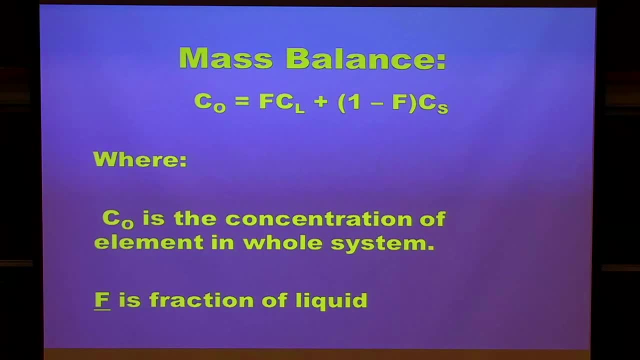 So it's our chondritic composition And in this case, in the equation F, will represent the mass proportion of the silicate Earth. which is what? Come on, What is the mass proportion of the mantle in this planet? Oh, I'm going to go home. 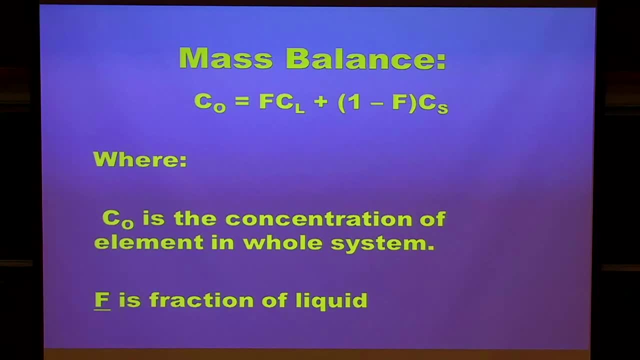 It's about? What's the inverse? What's the mass proportion of the core? I can do that. I'm not going to go forward until we get an answer. Okay, I'll tell you: It's about 33% of the Earth by mass. 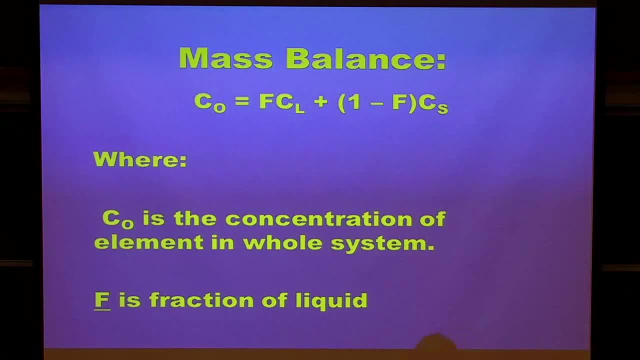 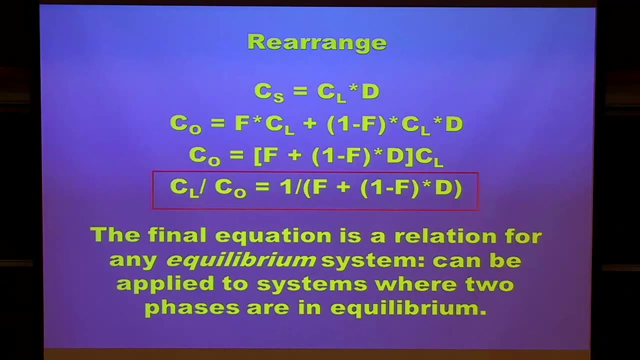 is the core and 67% by mass is the mantle. If you learn nothing else at CIDR 2014,, that's a good one to know. okay, All right Again. Bill went through this yesterday, so I don't have to do it again. 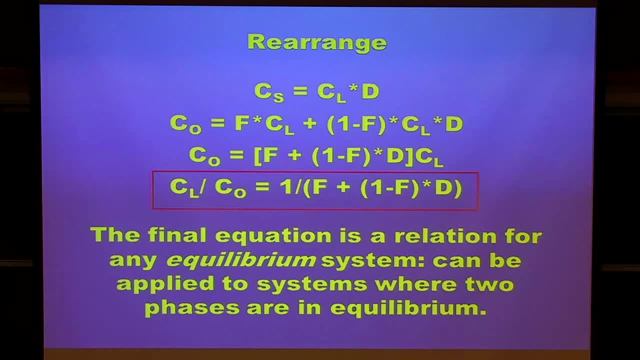 This is actually the equation that's going to go in one of the Excel spreadsheet cells that we deal with. The only question, And again, this is a useful equation for a system that is in equilibrium. Now, geochemists use lots of different equations. 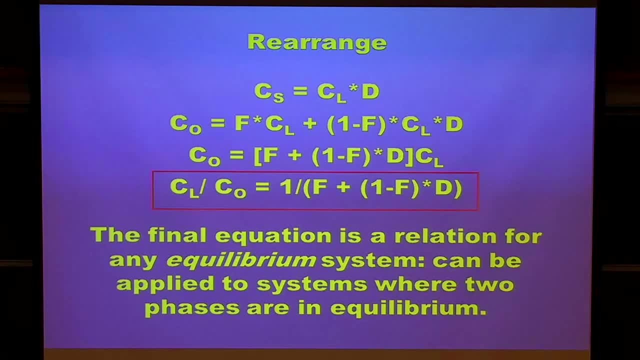 to model trace elements. This is a really, really simple one. It's probably not really applicable to this problem, but you know what? It's also probably not going to give us a result that would vary all that much from a much more sophisticated approach. 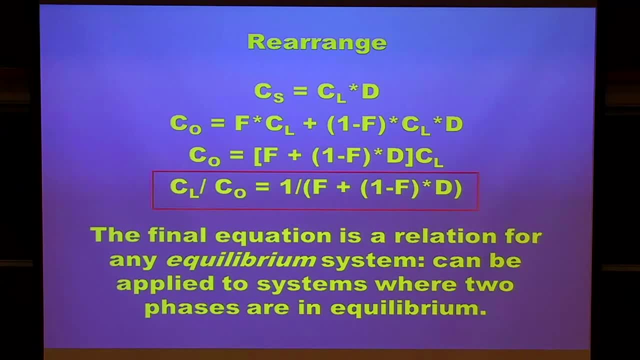 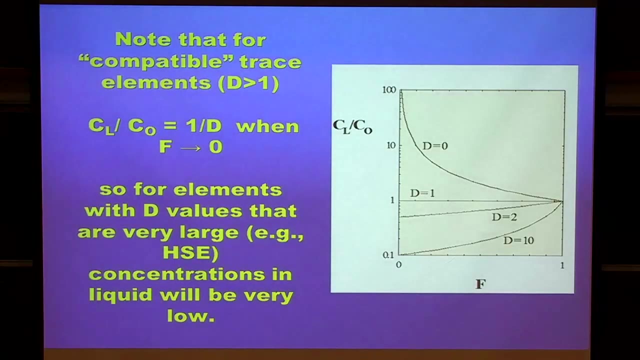 So we're going to go with this. This is something you can look in the cell. You'll see these terms and be very easy to understand where they came from. Okay, And again, this is the type of figure that you normally see in a geochemistry textbook. 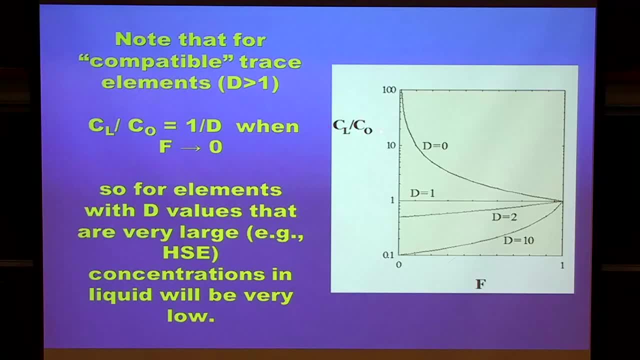 So this is concentration in the liquid ratio to the concentration in the starting system for incompatible and compatible trace elements. Are our highly siderophile elements considered to be compatible or incompatible? Well, that depends what you define as being the CS or the CL here in the equation that we're going to use. 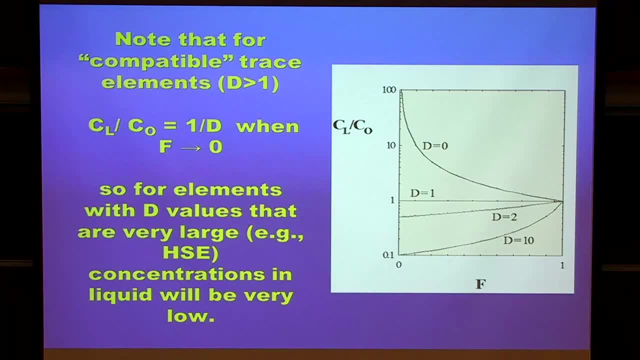 We're going to be looking at metal-silicate partitioning, and so the distribution coefficients that we will be applying are very large by and large, and therefore these are elements that, in the system we'll be considering, are highly compatible. So here's a D value of 10.. 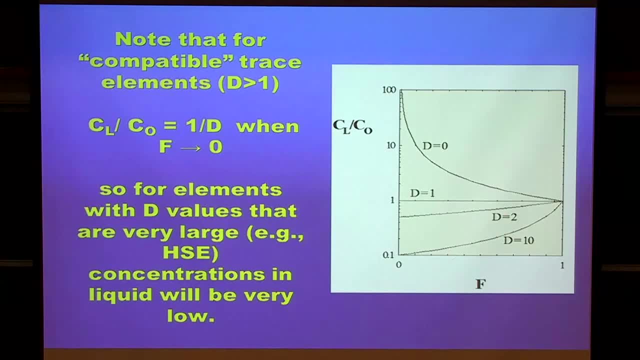 In some cases we'll be dealing with D values of 10 to the 7.. So you can see this relationship here: as you approach a very small proportion of mantle, you approach a concentration ratio of 1 over D, but you'll see that even for an F of 0.67,. 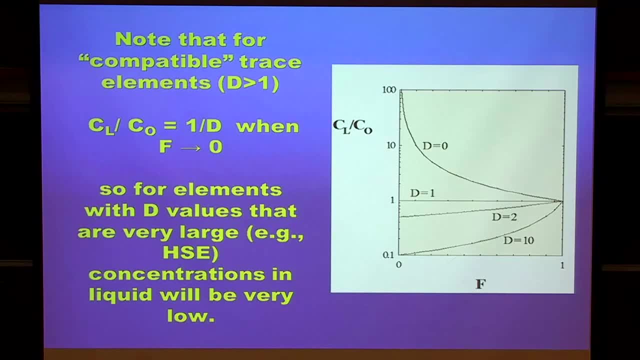 we're going to see very low concentrations, and that's consistent with what we see in the mantle. We do have low concentrations of highly siderophile elements in the mantle. Okay, so that's the theoretical background. Now a few other words before we get on with this. 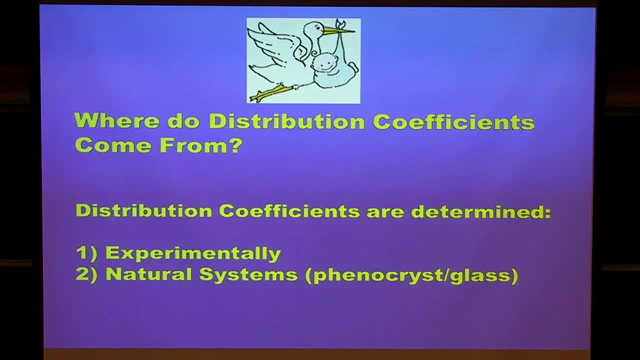 Where do distribution coefficients come from? Unfortunately, they are not handed down to us on golden tablets from heaven, and that's really unfortunate. They really come to us in fundamentally one of two ways: Natural systems- we can look at in some silicate systems. 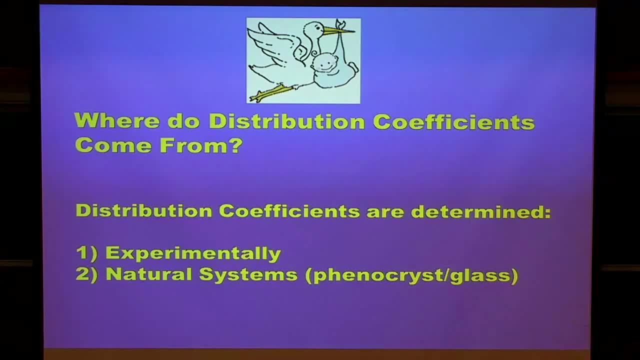 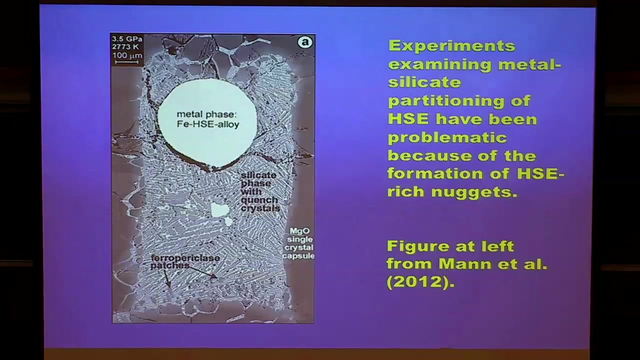 phenocryst glass ratios. In some meteorites we can look at metal-silicate ratios, But this is the way most of the ones that we will look at come from, and that is experimentally. And just a few words about experiments. 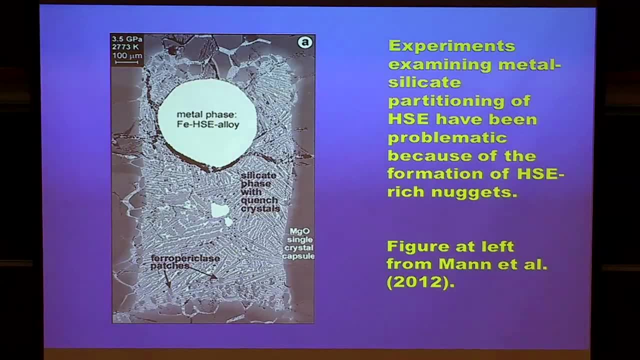 This is what an experiment looks like when you complete it and you saw it open and you look at it- and we have one of the experts on this subject, Liz Cottrell, right here- And what these guys did. Mann et al. 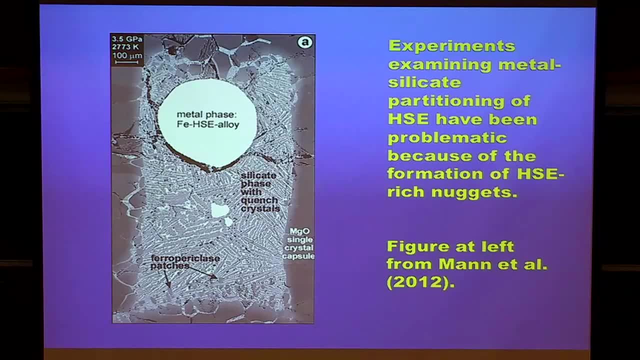 which is the paper that we're going to be drawing our data from. they put some metal and they put some silicate into a MGO single crystal capsule and they pumped the system up to varying pressures and temperatures and let it equilibrate. 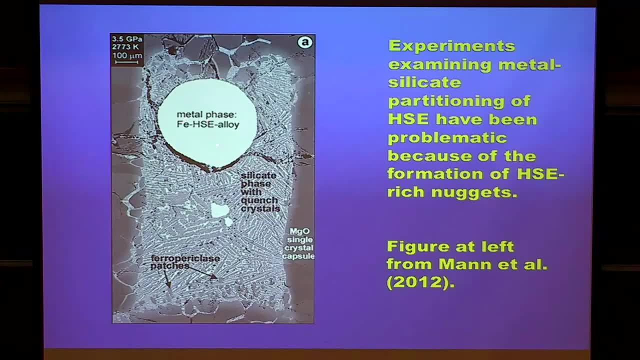 and then they quenched it and then they analyzed the metal and the silicate for the concentrations of the highly siderophile elements in it. And since a d-value is a concentration ratio, you just get a d-value from that. Sounds really simple. 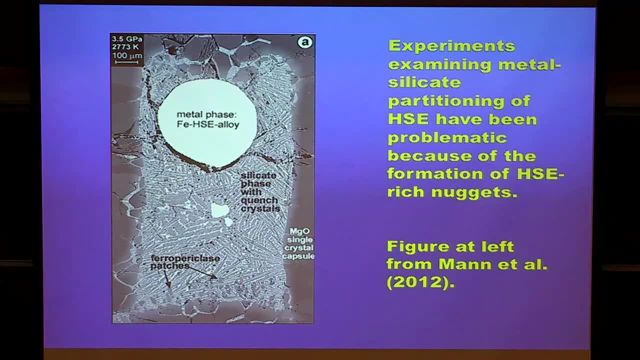 is it really simple? Yeah, So. so measuring their abundances in metal is easy, Uh-huh Right, And we won't talk about it here. but a real big issue that has plagued people that do these types of experiments is you oftentimes. 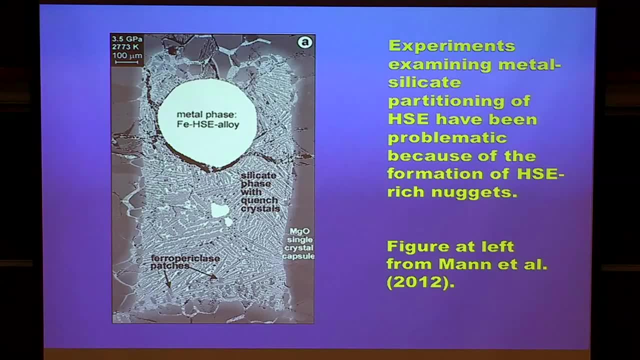 at the end of the experiment, when it's quenched, you find little tiny micro-nuggets of the highly siderophile elements in the silicate. And the question is well, how do you know if it's a silicate or not a silicate? 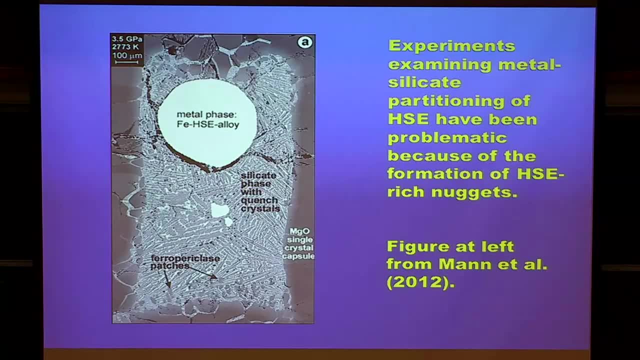 And the answer is: well, if it's a silicate, then it's a silicate. And the question is: do you include those in your concentration measurement of the silicate? meaning they exhaled from the silicate melt at the time it was quenched. 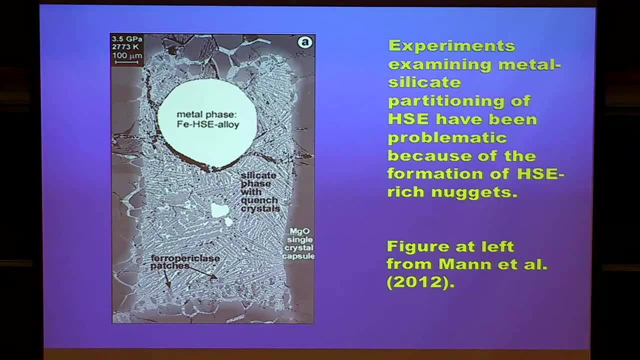 or were those just little bits of metal floating around in the silicate during the experiment, in which case you wouldn't want to include them? So it's a complex issue which I don't do, and any questions you might have should be directed at Liz. 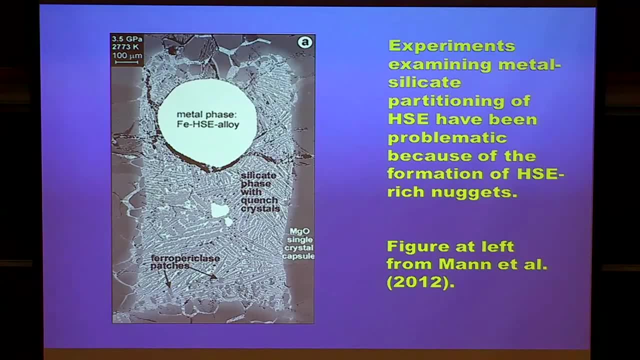 but go ahead, you can try. I just have a quick question: How long Here here? Oh, Quantitatively, how large are the uncertainties on these partition coefficients, Like, how much wiggle room do they give you? We're gonna look. 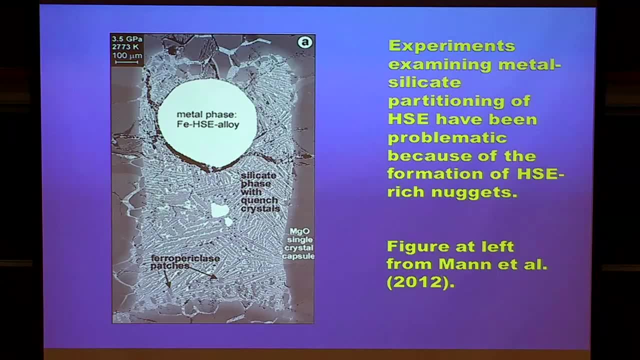 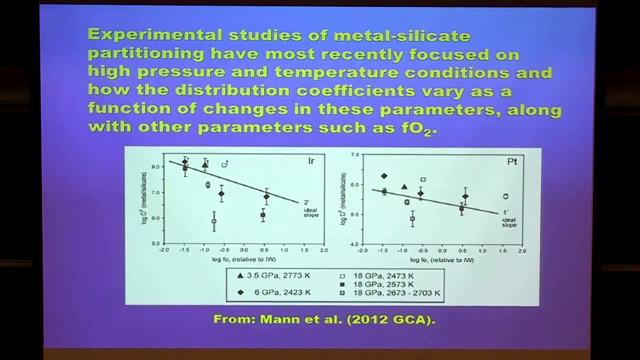 We're gonna see that You're gonna get to insert different numbers into the spreadsheet. Okay, So you will soon have a feel for that, a very good feel for that. Okay So what else is varied Pressure temperature, This paper? 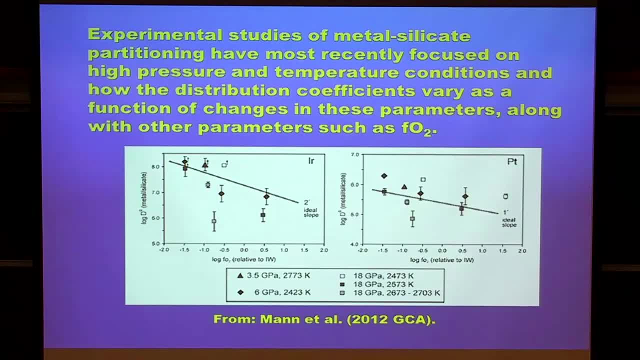 they varied oxygen fugacity, and so the three variables that are present in the data that we'll be working with are pressure temperature and oxygen fugacity. Liz, are they all unrelated? Can you just dial up any pressure temperature, oxygen fugacity you want? 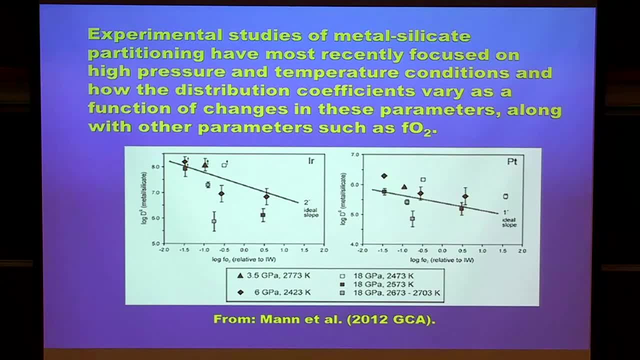 in three words or less. In these data sets pressure and temperature are often involved, because the higher you go in pressure and in thermic, the higher temperature you need to go to melt and silicate. So in large data sets that go over many, 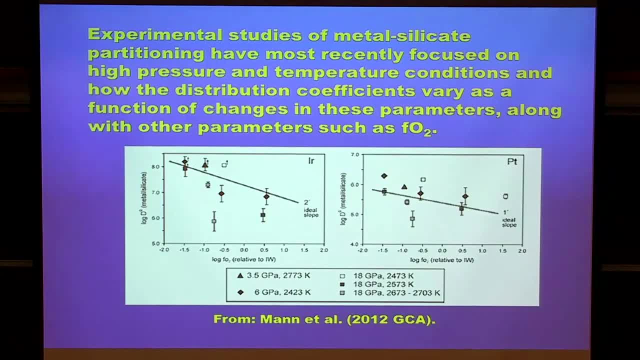 you know, through pressure steps and transitions and water flow, you know you can see that the pressure and temperature are often involved, because the higher you go in pressure and in thermic you'll see that pressure and temperature are difficult to disentangle. 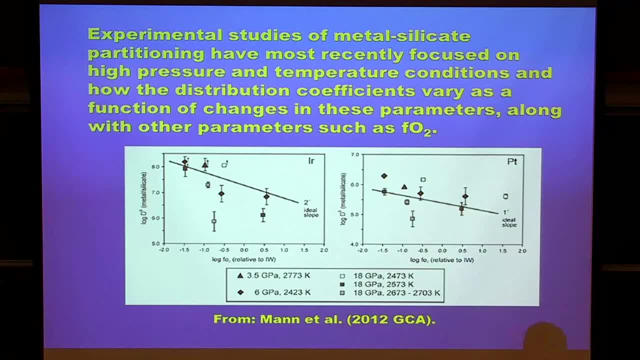 with independent variables. Oxygen fugacity is more of a let's measure what we got after the fact then. I would not say that in any high pressure experiment oxygen fugacity is controlled. It is. we try to assess it after the fact. 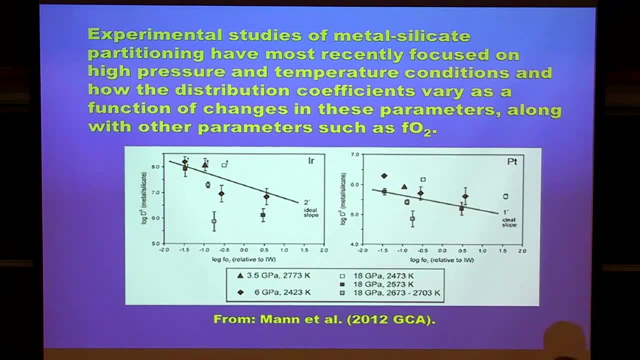 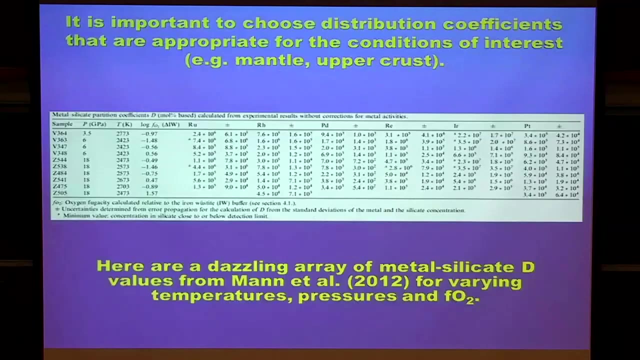 One atmosphere experiment, the oxygen fugacity, is controlled and known with great certainty. A leaf experiment is controlled, and known with great certainty. Leaf experiments are large and there was no control. It was only kind of detective work after the fact. Okay, you asked about. 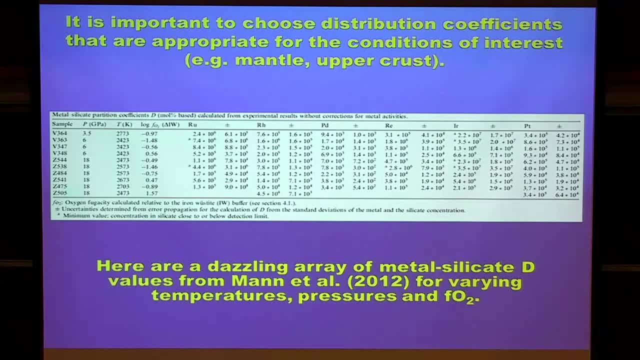 uncertainties. This is the actual table from the paper that we're working with. Why are we working with this 2012 paper? Well, it's useful because this group did a bunch of measurements of different highly siderophile elements all in the same set of experiments. 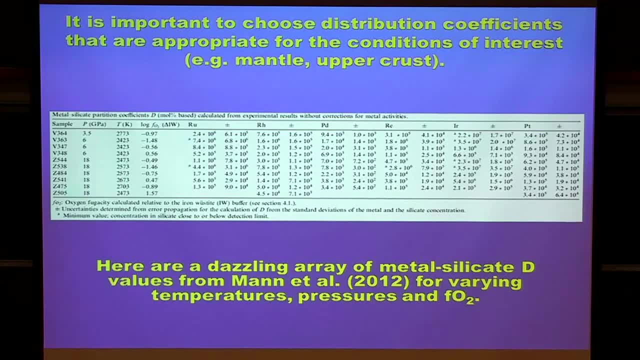 and so we have data for a bunch of different elements again processed under the same conditions. You will see little plus or minuses. So these are the uncertainties associated with it. These data I have put into the second page of the Excel spreadsheet. 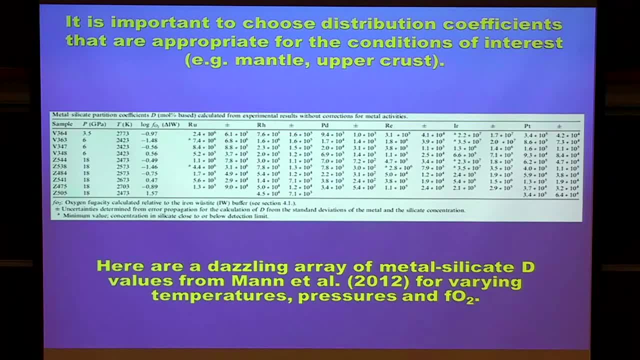 and these are the things that you're going to vary in your groups to see what their effect is on concentration. Yes, Liz, Are you going to talk at all about this? No, I'm just going to continue with these and see what happens. 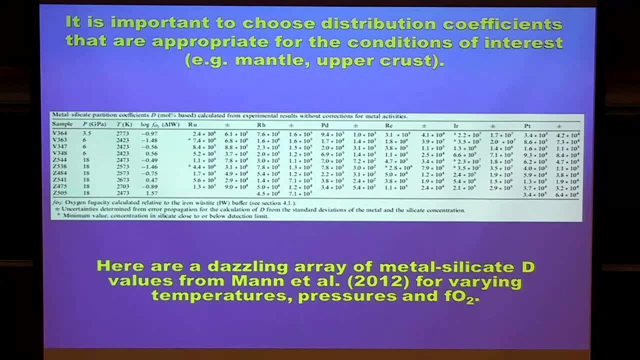 Okay, so I call this a dazzling array of metal silicate D values. We are just going to apply them directly. I will notice here, or I will have you notice they go. here's the different pressures: 3.5 gigapascals. 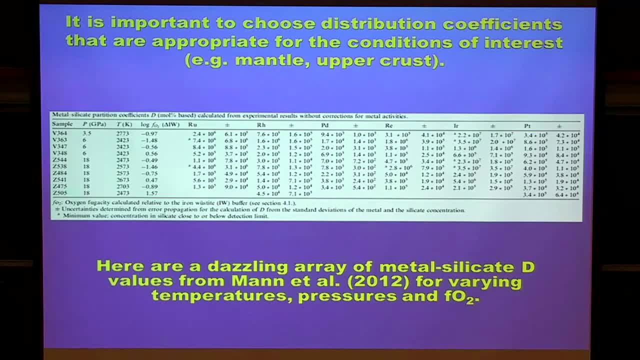 up to 18 gigapascals. We're going to go to 40 and 60 gigapascals related up to them, and that's something that's worth keeping in mind. Why don't they just simply do these experiments at 40,? 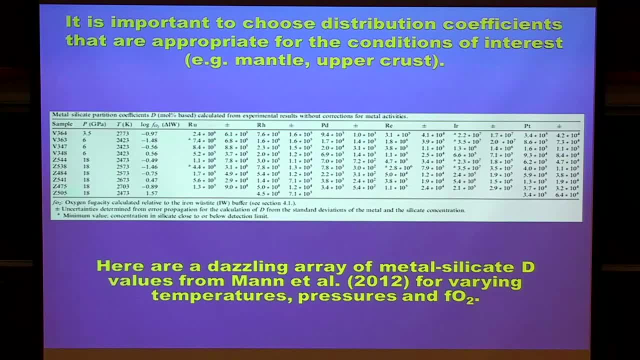 as I'm sure we'll hear something about that here- to very high pressures and temperatures. but they produce very, very small experimental charges and we need a lot of atoms to make measurements, especially if you have a really high distribution coefficient. So 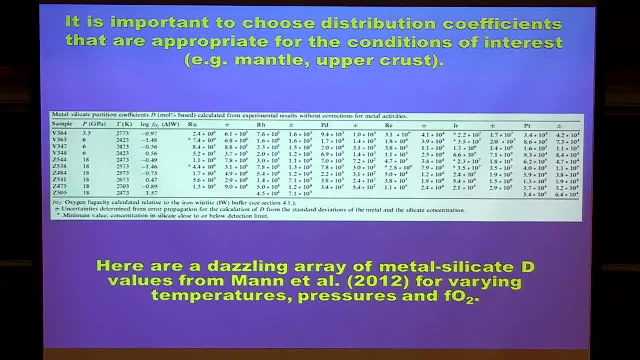 this is really hard work, and so a point that I want to point out is that the measurements are not from the heavens above. they are for specific conditions, for specific compositions. they did the measurements in certain ways. it by no means is the only way. 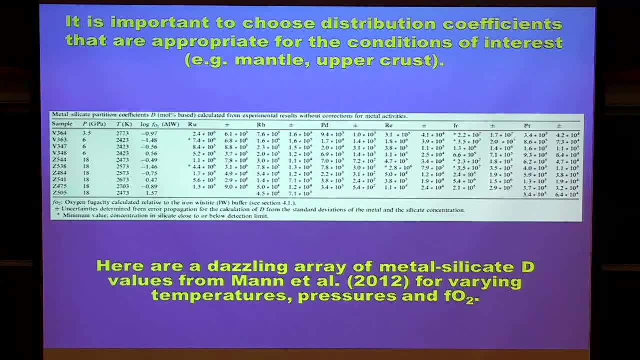 you could do this? Yes, What do you say? Well, I'm asking for a comment. These are quite large, Yeah, and those are probably. I mean, those are probably just. I hate to tell you, but those are probably just their. 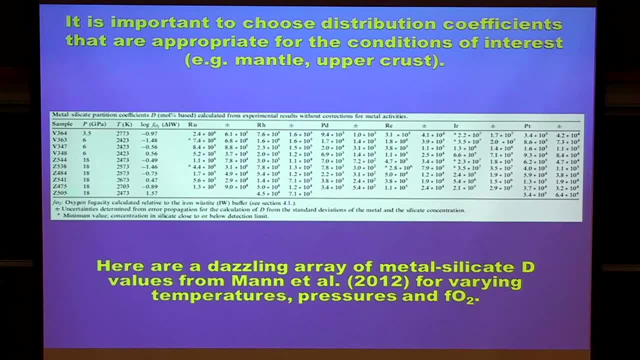 measurements. Taking these coefficient and applying them to the earth requires an activity composition correction, and that is the whole. These are just probably just the measurements that you can do. There was another question. What I don't understand is if you look at these: 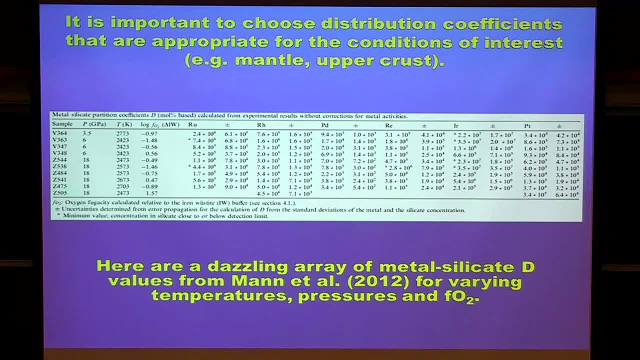 and maybe this is the point of the tutorial, but if you look at these coefficients for the different elements at the same conditions, they're all the same. No, it's the same row. Well, these are different elements. Yes, all the. 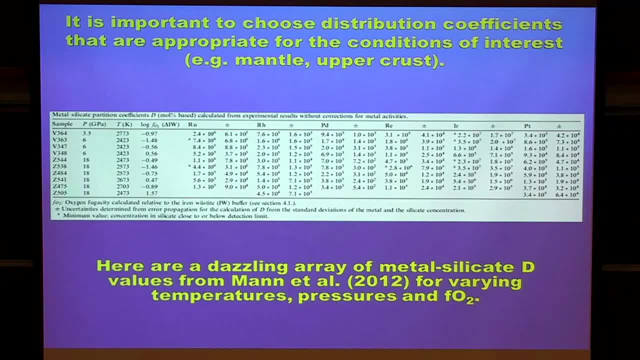 elements are different, But when you look at that line, they're all the same. That's what we're going to model. We're going to try to duplicate that. You're just so close, Okay, Anyway, so we're going back. 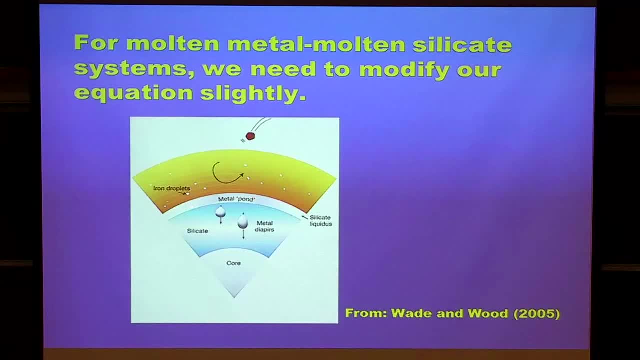 to this. This is a figure from Wade and Wood, a 2005 paper that everyone likes to use. So again, just to reiterate, we're going to be looking at partitioning between metal and silicate, as you might envision want to. 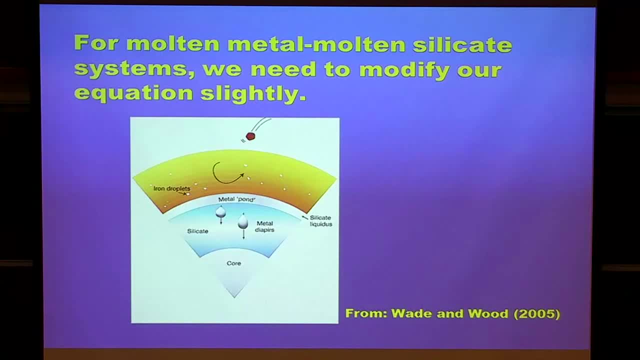 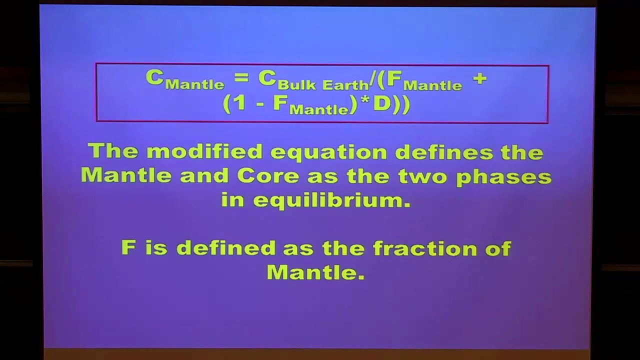 model the partitioning as a function of Earth growth, And I'll show you a figure on Saturday where people have done that. That's something that Wade and Wood have actually done, But by and large, this is what we're about to model. 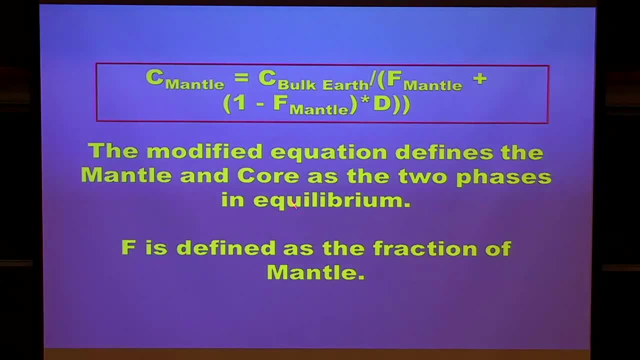 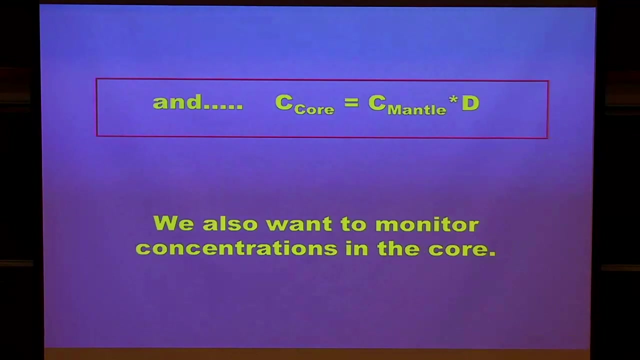 Okay, So we're not doing CSCL, We're doing C, and this is ultimately what is in the cell that calculates the concentration of the highly siderophile elements that result from trace element modeling in the mantle. And how would you calculate the core concentration? 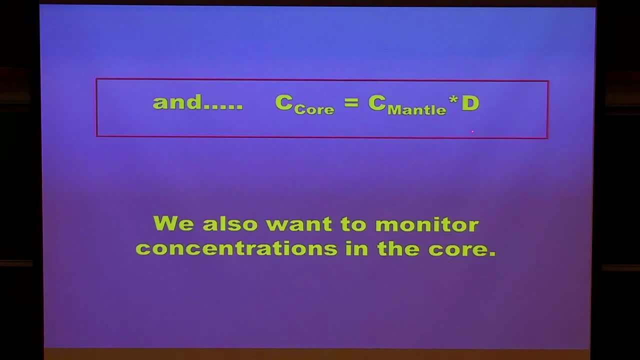 Well, if this is truly equilibrium, gee, we're going to calculate the corresponding core. One of the things that you'll want to notice is: is anything happening to the core? We're changing partition coefficients. How does that affect the core? 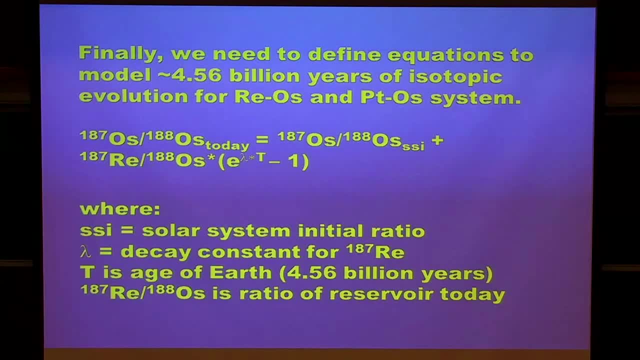 Does it affect the core at all? Of course it affects it some, but we'll see. Okay, One of the things we want to do is, once we have created a mantle 4.5 some billion years ago with the highly siderophile, 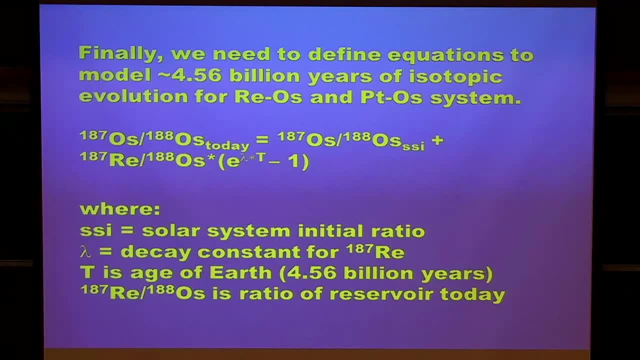 element abundances that we calculate what are the implications for isotopic evolution for the next 4.5 billion years? And it's a relatively simple problem. We're going to talk about the composition of the mantle in the mantle. Again, geochemists. 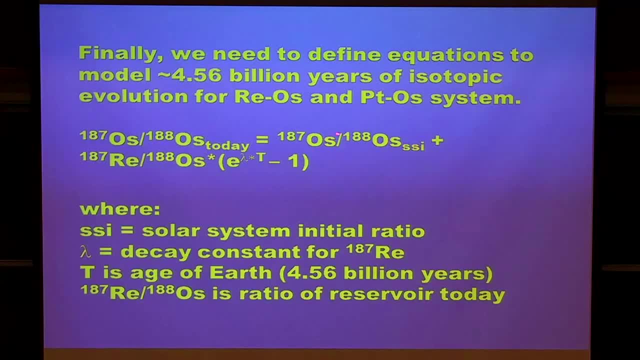 nitpick about what the osmium isotopic composition- 187 isotopic composition of the mantle is today, but not a whole lot. not enough to talk about Man et al. the paper that I'm taking the distribution coefficients from did not 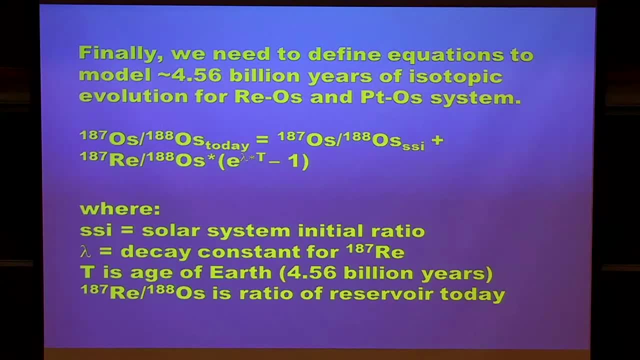 include osmium in their experiments. Why did they do that, Liz? Yes, It's a hell of an element. We don't care about toxicity, but No, I know. but instead we're going to use a. 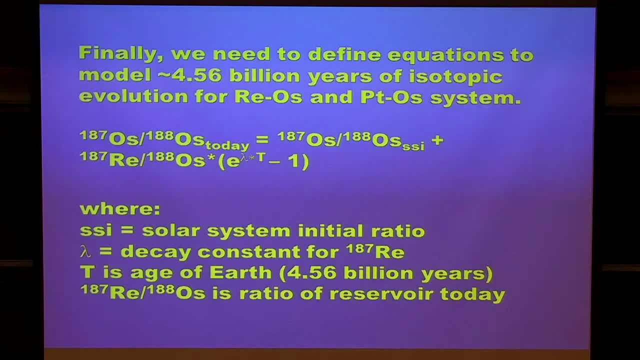 near geochemical twin, and that is iridium. So you'll notice on the spreadsheet that I'm just using the same distribution coefficient for osmium as they measured for iridium. One of the criticisms of this type of modeling, then, would be: 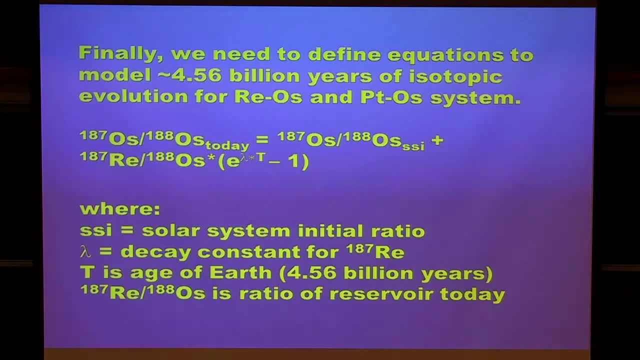 we don't. actually I can't answer that in three words or less. Everybody runs things under different conditions so it's not that easy to make a comparison, but I don't think they're wildly different. This is just a fun exercise, folks. 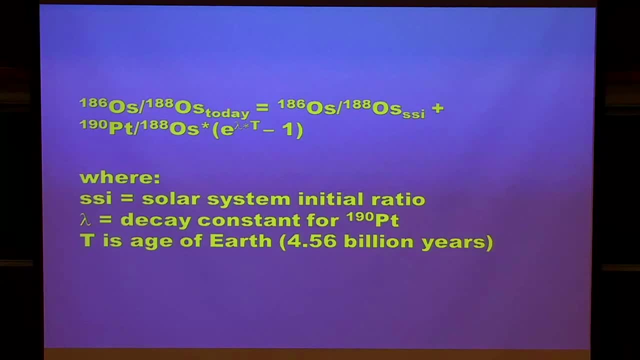 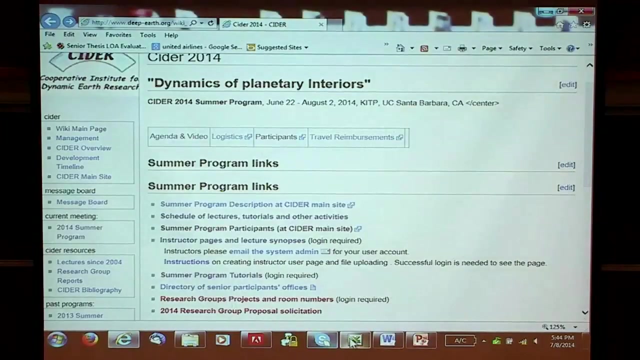 And then finally, osmium-186, same thing. We measure platinum and we measure osmium and see how this system evolves to the present. So that's all I have to say. I just want to show you the spreadsheet and give you a really quick overview of it. 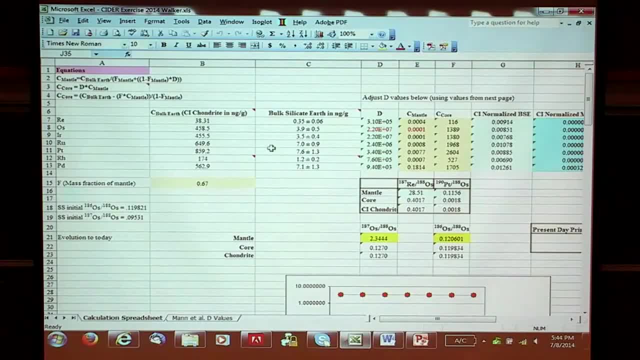 So this is what it looks like. Hopefully you have something like this on your computer. Just as a quick aside, these are the bulk Earth values we get from C1 chondrites. C1 chondrites Actually aren't a particularly good fit to the Earth. 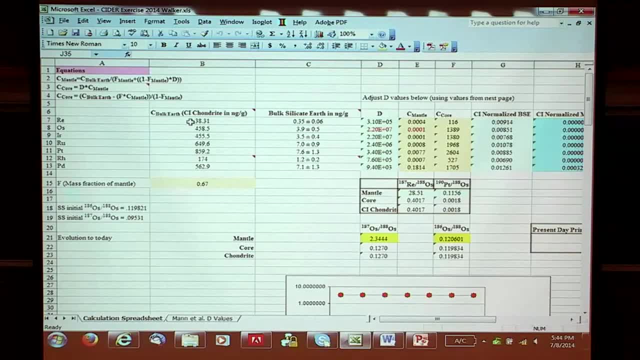 from a highly siderophile element standpoint. We can discuss why that is later on. Bulk silicate Earth or primitive mantle concentrations are shown here with their estimated uncertainties. This column labeled D value. this is what you want to vary. It's very simple. 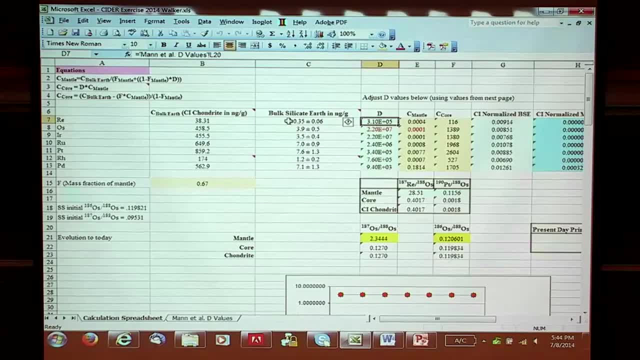 If you look at the box, it refers to the next page of D values. All you need to do is change that final digit or final two digits in this box to change the distribution coefficient to the set of conditions that you'll be assigned. 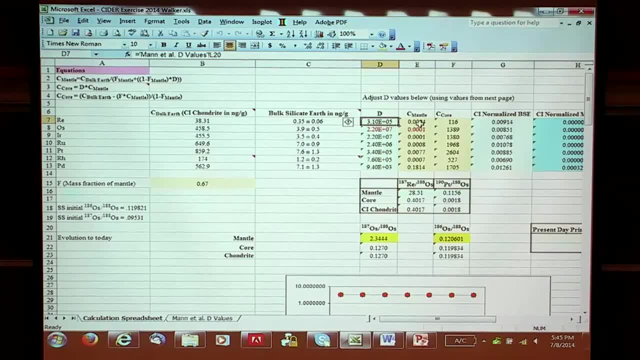 The spreadsheet will calculate concentrations for you in nanograms per gram in the resulting mantle and in the resulting core. So pay attention and see if anything changes as you change distribution coefficients. Geochemists like to normalize things, as we learned yesterday. 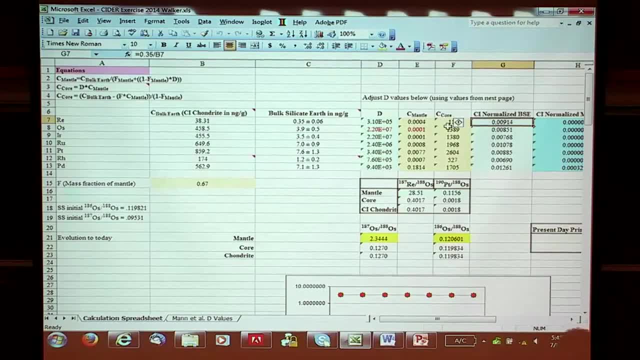 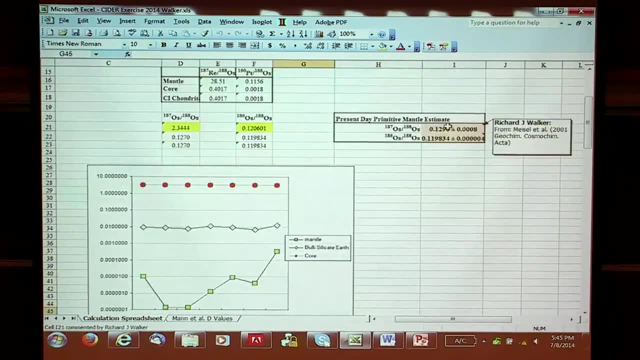 So we're going to normalize the results, The results to chondritic, and that's what these three columns are, And down here I've even got it plotted for you. Isn't that nice? It is. So you can. you can, you can. yes. 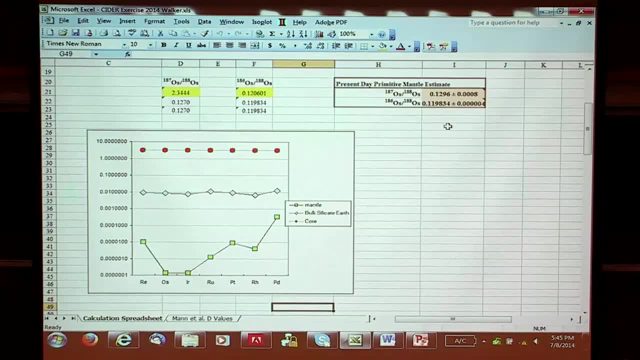 I had to get my wife to get me to show me how to do that. I don't actually know how to do that. Yes, I was wondering if you could talk just a little bit about the what we looked at, the FO2 numbers. 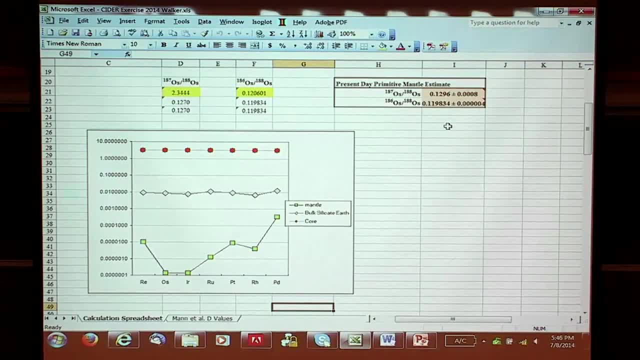 What we should- just a reminder of which we should take as a monofilament for the surface and the Core formation is often modeled. but that's one of the questions that we one of the reasons why we've done these studies. 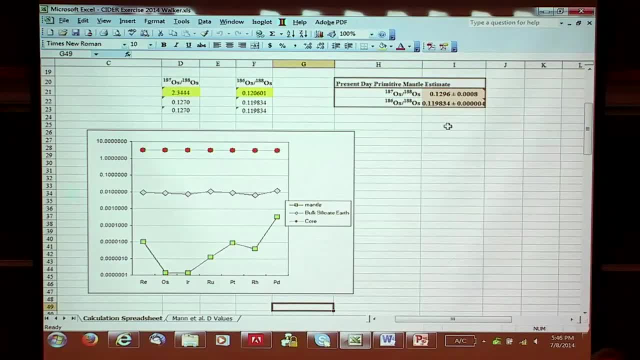 is to figure out the likely op. sorry, I don't have it. Oh sorry, This will work. One of the reasons for doing these experiments is to do this kind of modeling to determine the likely oxygen fugacities. But you can see, this is very relevant for core formation. But based on the iron content of the mantle, we typically think of core formation as having occurred at iron woosite minus 2,, if that means anything to you. So two orders of magnitude below the equilibrium between iron metal and woosite FeO at any given P and T. 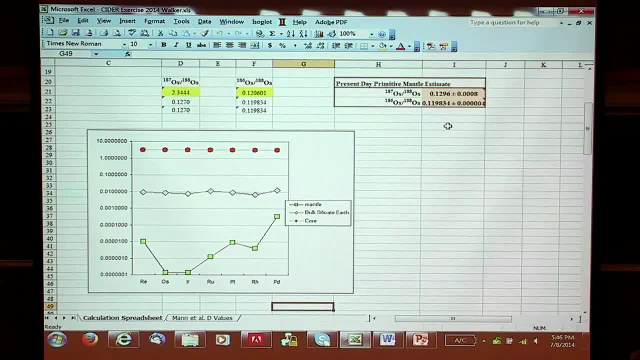 So we don't have any that are actually this low on our list, and we have some ranging from minus or minus 1.5.. But just assuming that you know that this is what we think is the probability. So do you want to step back? 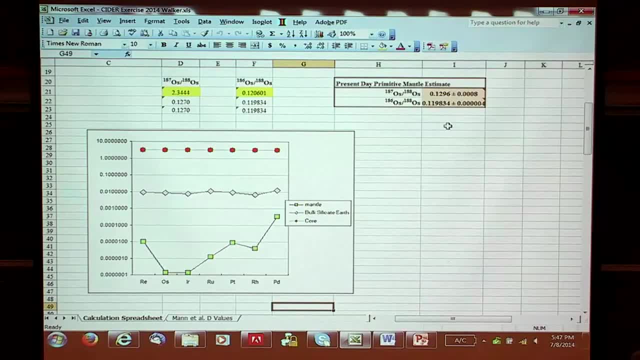 Okay, thank you. Great. So we have two orders of magnitude below the equilibrium that were, at any given, P and T, so that we're able to type and we don't think of any that are actually this low Male Speaker 2 because, right, because they're trying to. 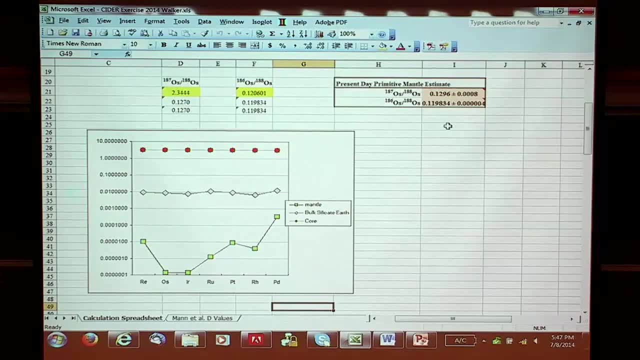 probably avoid the micro nugget issue, which is an experimental problem plague, and because, like I said, it's difficult to control the oxygen fugacity, and so that's just how the experiments came out and why one experiment comes out one. 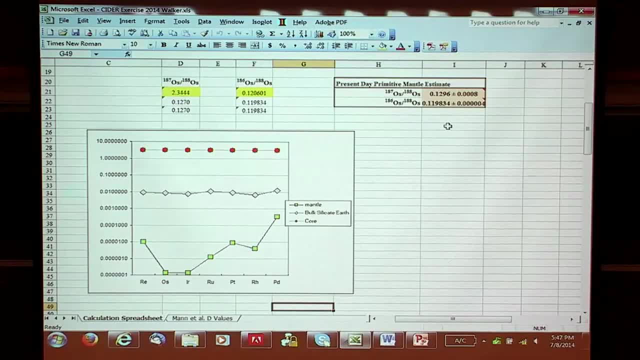 way and another comes out. another is not always easily understood, Michael. I don't think anyone defines oxygen fugacity. What Should I just mic myself up? Yeah, you can sure. So I'm going to do that on Friday, but oxygen fugacity can. 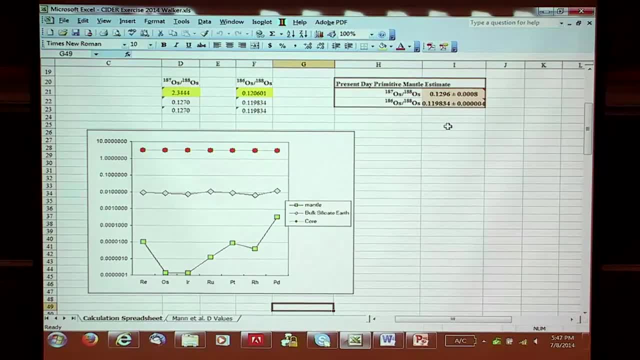 be thought of. the oxygen fugacity in this room is .21.. It's the oxygen partial pressure. in an ideal gas, partial pressure and oxygen, Partial pressure and fugacity would be the same, would be equal, in an ideal gas, an ideal solution of ideal gases. but we 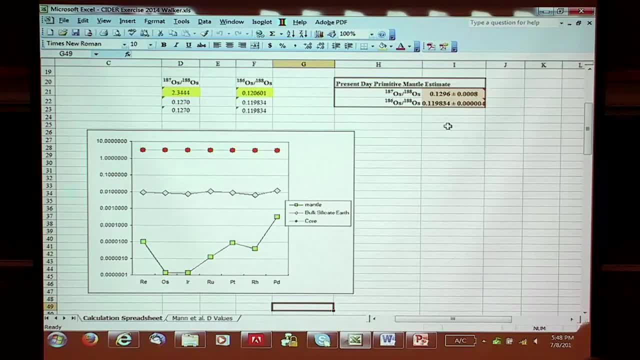 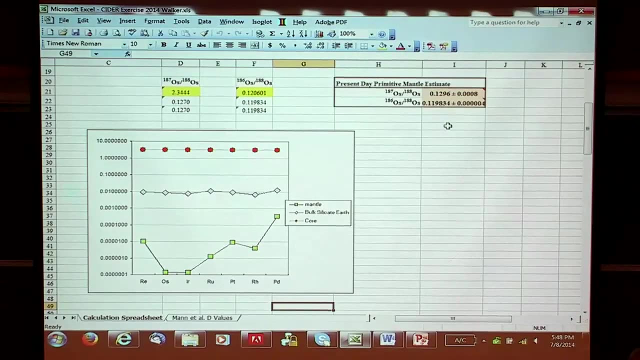 don't have that, so we add the fugacity to indicate, to account for non-ideality. so fugacity stands for like fudge factor, if you will. and so rock is certainly not an ideal gas. and so, since rocks are not ideal gases, it's oxygen fugacity. but 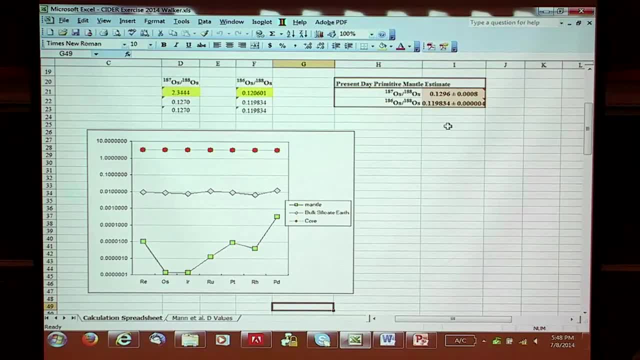 you can think of it in thermodynamic terms. it's the activity or the chemical potential of oxygen in the system, which is just what partial pressure is. so that's oxygen fugacity. Partial pressure is the way to think of it. Yeah, the activity, it's the activity. 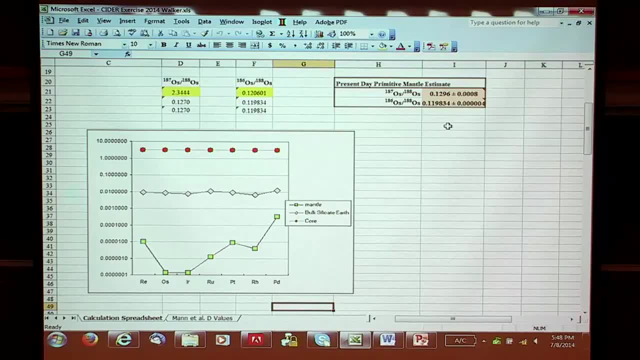 It's not like there's oxygen that's hanging out the way you're around, right? It's not free oxygen, Right, And so it's the availability of oxygen to participate in chemical reactions. You can actually have a lot of oxygen in the system, but you 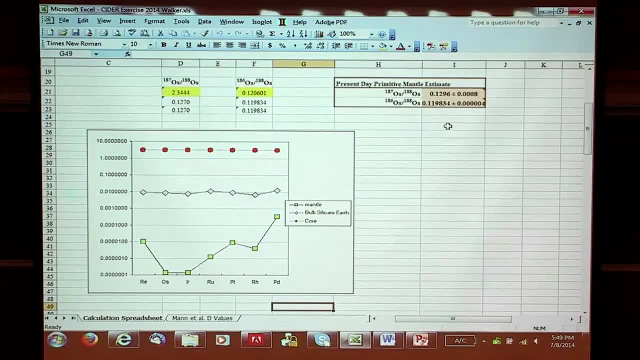 can't have oxygen. the mantle is 44% oxygen, but relatively reducing relative to the surface environment, because the oxygen is not free to participate in chemical reactions and oxidize other species. Okay, we need to move on, but quick, Yeah, just for clarity, this, these experiments were done with. 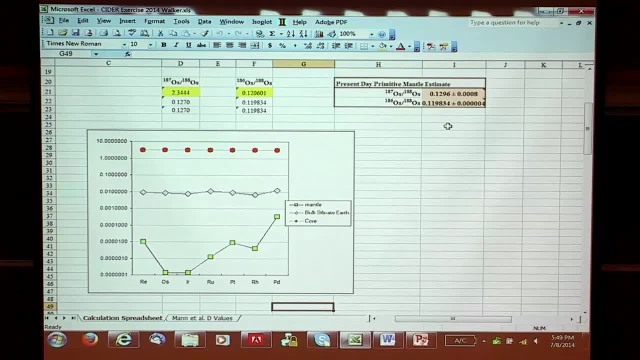 pure iron, right. So they were not done with a sulfur- Impossible. But they weren't done with any sulfur or iron or silicon, which could. You're getting to the final end state question that we want to think about, which is: 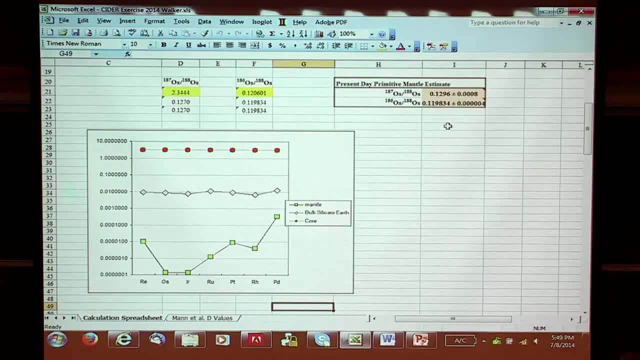 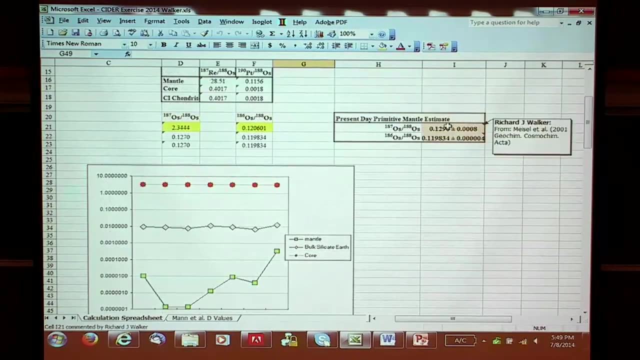 The metal surely has all of those dissolved in it though, because it's in equilibrium with a silicate melt. No, but for you said. silicon, for example, oxygen carbon are all unavoidable in the metal. It doesn't matter if they meant to, if they end up in the 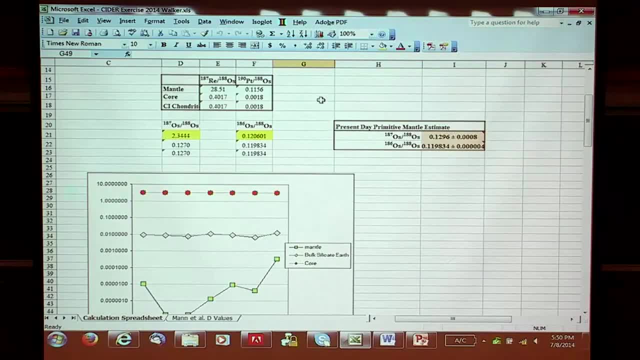 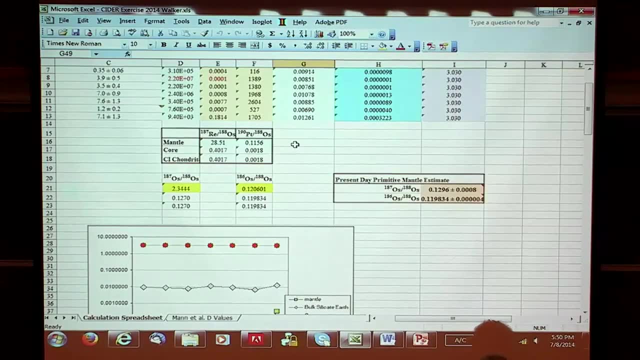 silicon, right, If they added it deliberately or not, Yeah, but you might be Right. No, right, they're not done in graphite, but silicon will be in there for sure. Okay, just keep thinking. This is, this is a simple calculation we're doing. 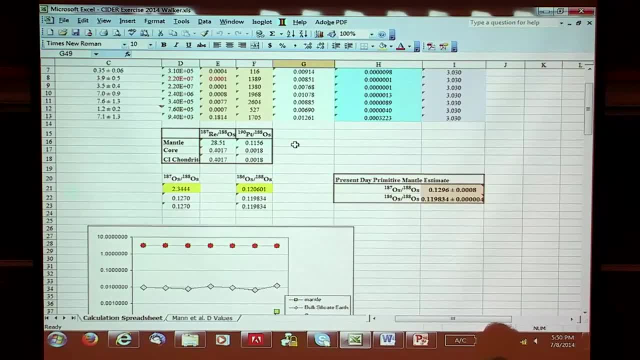 So the last thing I want to say before turning you loose- sorry this has taken so long- is isotopic evolution. This is done for you. So we take the rhenium-osmium and platinum-osmium ratios that result from the partitioning calculations. 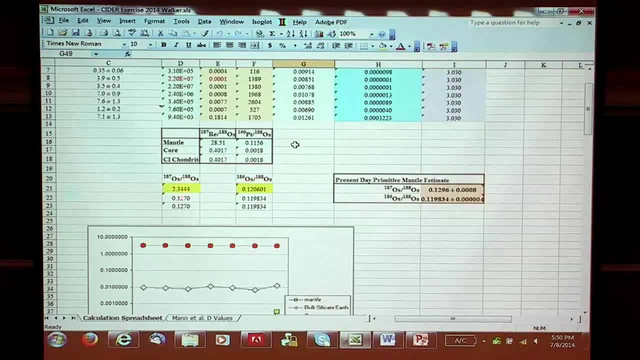 They get plugged into these two yellow cells. Actually, they get the results, get plugged into all six of these cells, but these yellow cells represent the isotopic composition of the mantle after 4.6 billion years of evolution with that ratio. What does that mean? 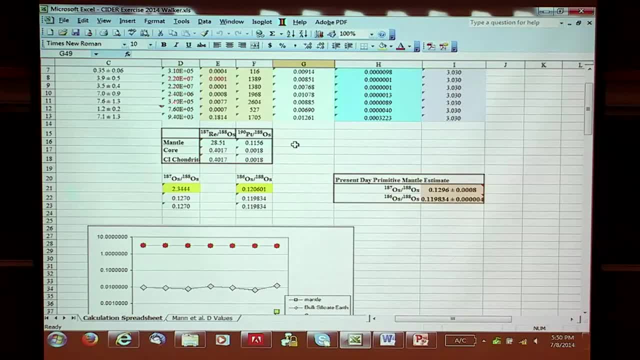 Well, in this case- and I think in this case- I have the lowest pressure experiment embedded in the D values for the spreadsheet I'm showing you here. This would give us a present-day osmium isotopic Composition of 2.34,, which means nothing to you. 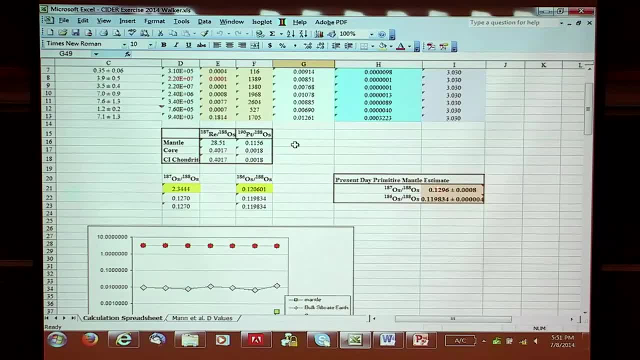 But you can compare that with our bulk silicate Earth or primitive mantle estimate for today, which is about 0.13.. Does that sound similar? It does not. So this, this result is wildly different. Here's osmium 186.. 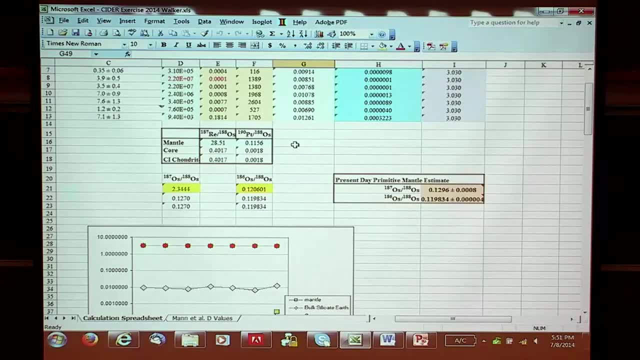 You have to look at a few more significant figures to grasp the meaning of this. This is 0.12060.. The present-day measured value of the mantle is 0.119834.. Notice the uncertainty in this is pretty far over to the right. 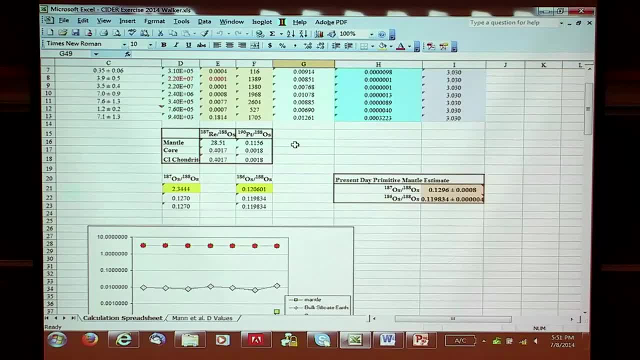 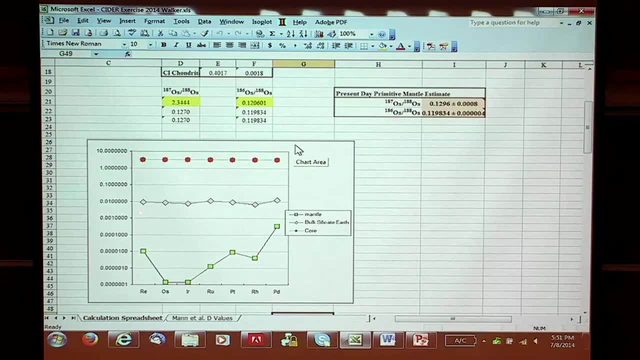 So this is a failed model as it is, And you can. you can see that down here in the figure. What you want to do is this is the bulk Earth. That's not going to change Whatever you change in the spreadsheet the green represents. 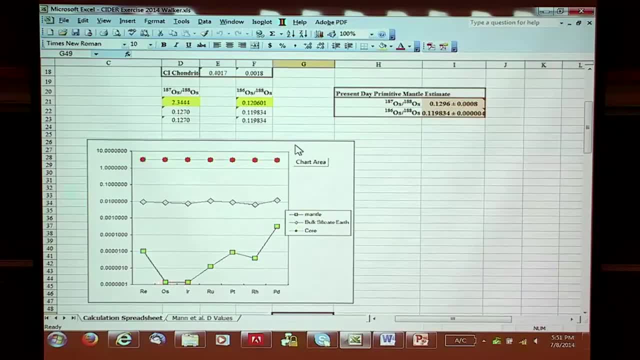 the resulting mantle. You can see the osmium and iridium are the same because we're using the same distribution coefficients. This is the core. So the abundances that we generated by this low-pressure experiment are way, way, way below where the the mantle is today. 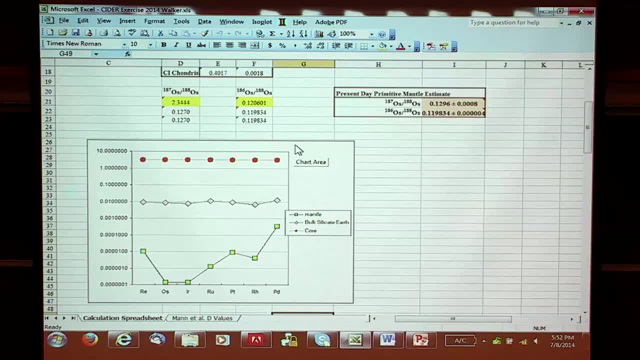 And also, as we just saw, the isotopic compositions are very different. Okay, so it's not going to take you long to put the different distribution, your groups- not you specifically, but somebody's going to have to do this- put different distribution coefficients in the. do we have a way of blocking this? 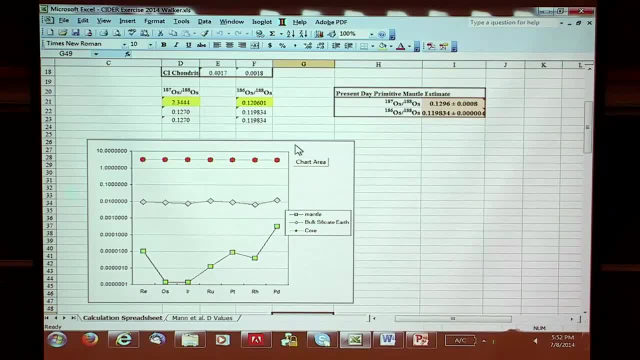 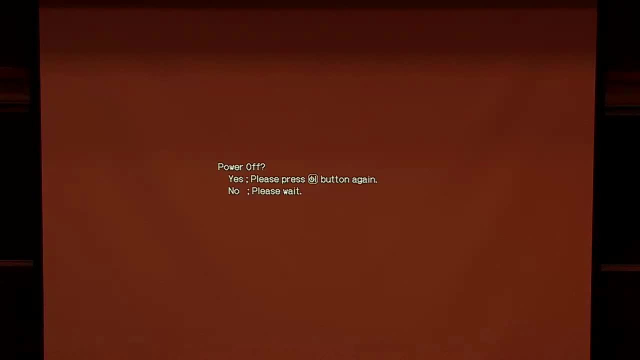 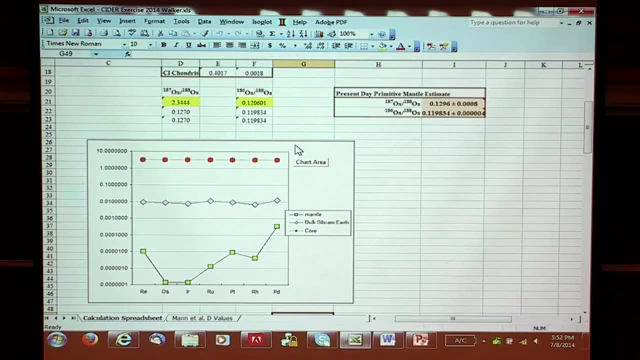 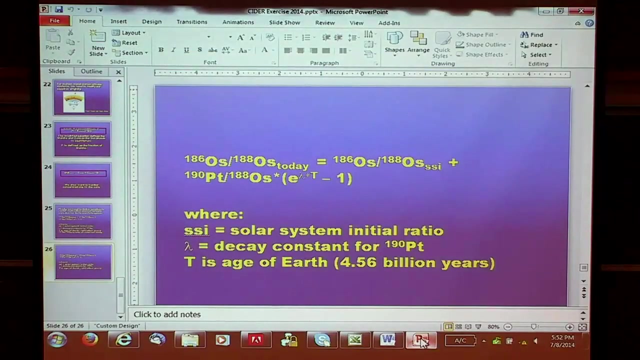 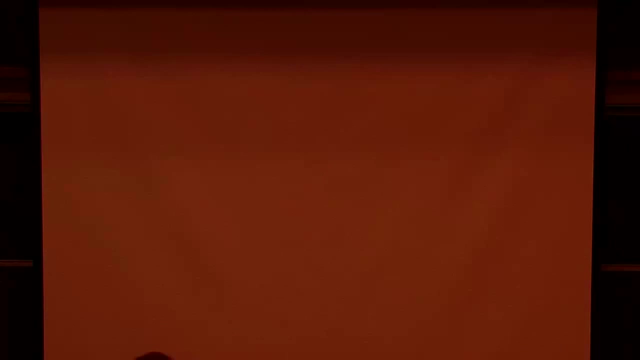 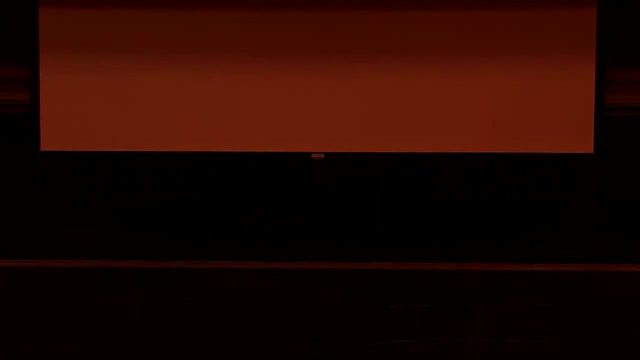 off without turning it off. huh, standby, does that do it? oh no, I don't hit B really. is that going to solve it? oh, very good. so here's the questions you really want to think about. as you do this, we'll divide up into our groups. ah, here are your groups: the groups one, two, three, four, five. these represent the different conditions. 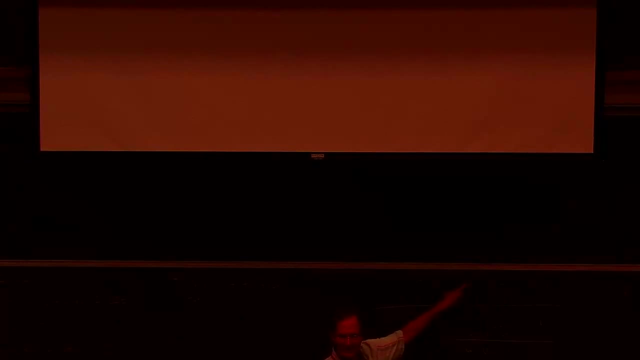 on that second page of this. sorry, i could have written bigger on the second page of the spreadsheet. they represent different lines, so i have the line number. so you really just need to change the final two digits in the d column in order to embed the correct distribution coefficients. 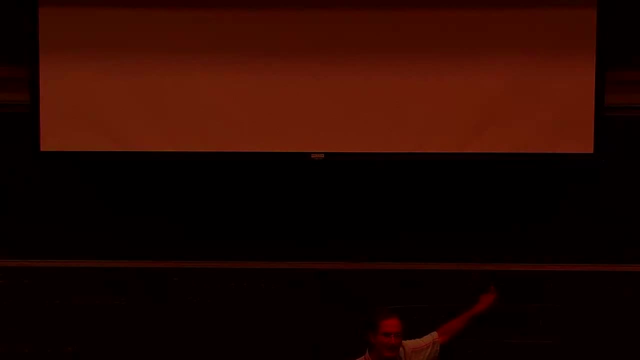 so this is not the interesting part of the exercise. so just each. each of these groups should do at least three, but you're welcome to do as many as you want. look at what pops out the other end, so you'll get the highly siderophile patterns. look at the isotopic composition that result from that. 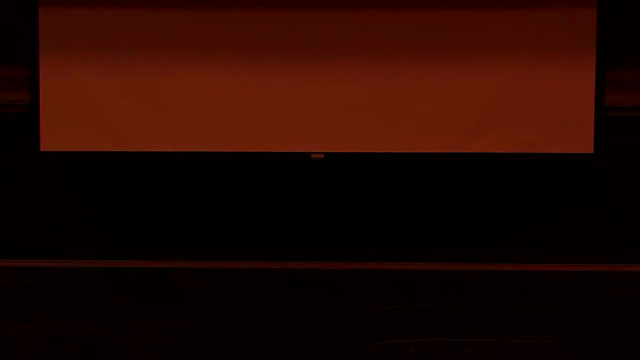 and then consider these questions, and i don't know if you want to do this for, but we'll come back, maybe after. we'll go until what 3: 30, go to the coffee break and come back for about 20 minutes to discuss something like that. so here they are: results of gosh. that's not grammatically correct, is it? 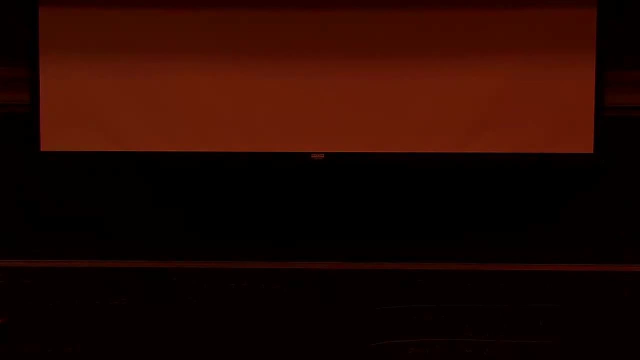 results of model with in comparison to bulk silicate earth. i've already told you the answer to that, which is: none of these are going to be particularly good. maps matches to it, but what's wrong with them? what are the particularly offensive elements? do any of the 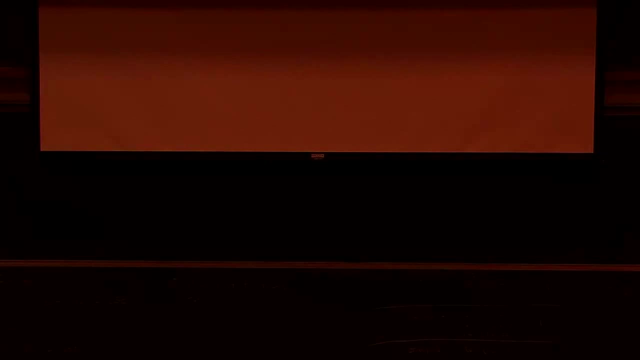 elements work. okay. number two: isotopic results. do any of the isotopic systems work? do any of the? do we get something approximating what the modern mantle is with any of the conditions that are incorporated into that second page of spreadsheets? well, this is a nice one. 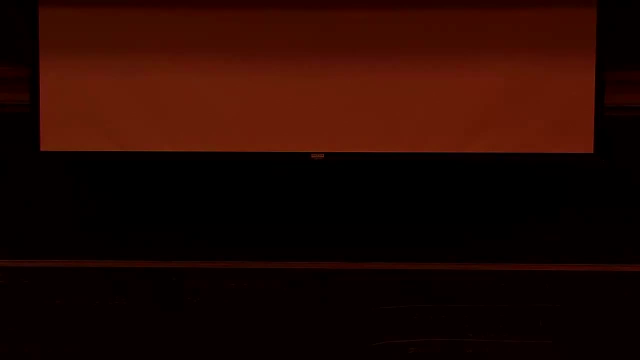 and this is where it gets a little more exciting. Uncertainty propagation: does it matter? People back here are a little bit concerned about very large error bars. Does it make a difference? if there is essentially an order of magnitude error bar, Try it. how would you go about doing that? Simplest way would just be: make the number as big as the error bar permits. make the number as small as the error bar permits and see what that does to the calculation. That's not the elegant way of doing error propagation, but it gets you pretty close to what you want. 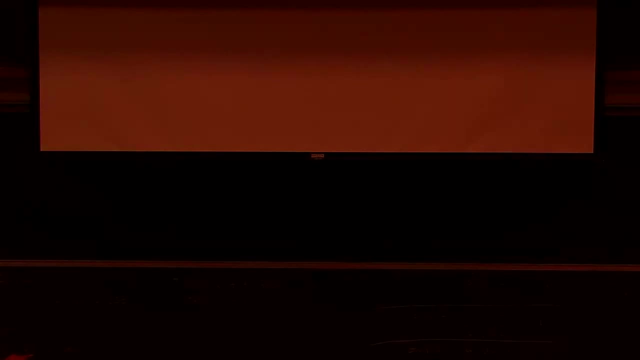 So again question is: does it matter Other body predictions? I don't know if we'll have time, if you have time, to go through this, but what are the predictions for other planetary bodies if they experience magma oceans? The Moon, Mercury, Mars have very different size cores. Moon about 2%, Mercury about 80%, Mars about 2%. If you had the same applicable distribution coefficients and you chose the right conditions, what would you expect to get in the mantles of Moon, Mars and Mercury D-value constraints? 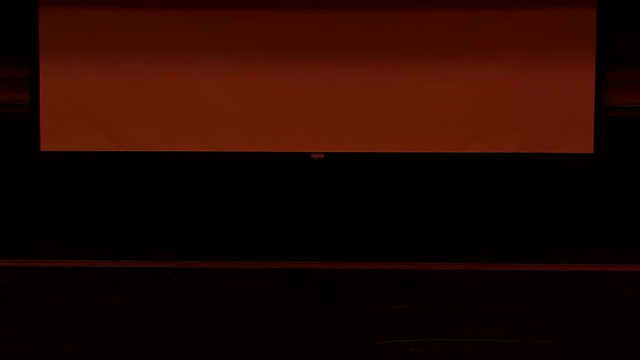 You can turn this around. You can say what kind of D-values would I need in order to generate the necessary isotopic compositions that we see, and how variable can they be in order to still be in the right conditions. So you can say what kind of D-values would I need. 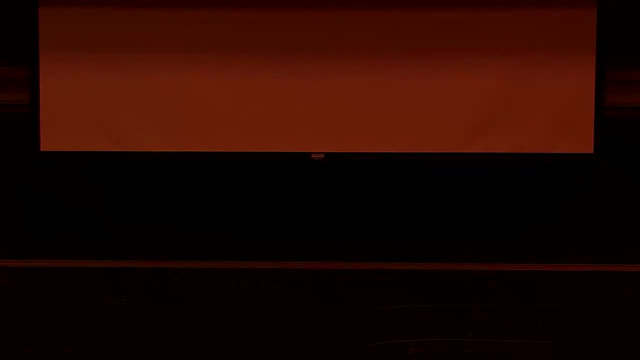 in order to still retain the isotopic compositions that we see. How would you approach that? You can just plug any numbers you want into the D-values until you get matches with the isotopic composition. See how much variability you can have in order to generate the isotopic compositions that we see today. 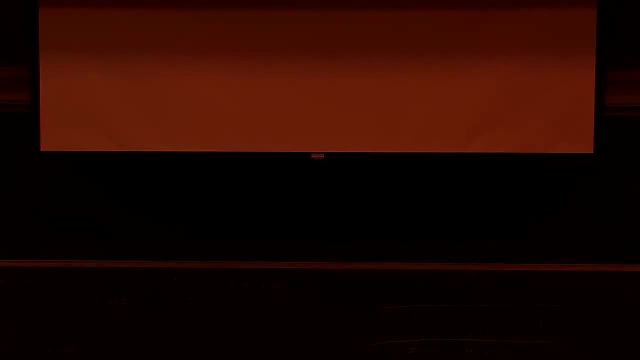 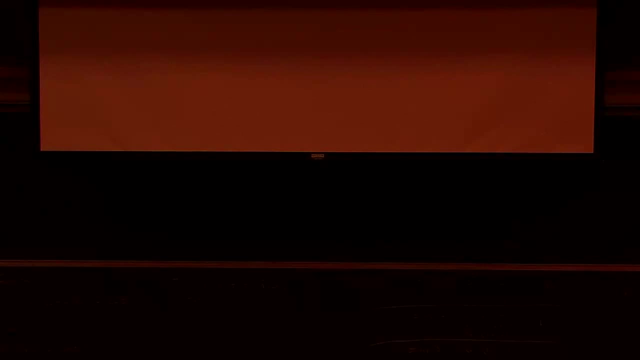 Liz did some experiments. When was your PhD published? So about 10 years ago. She did some phenomenal work on platinum, the element platinum- And she got, I think, pretty similar results to what we're seeing with the Mann et al results. 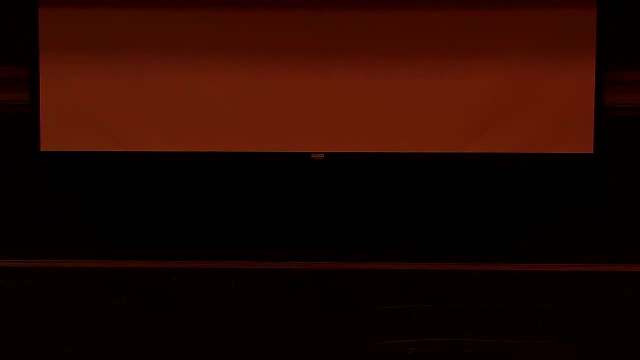 I don't think there's a dramatic difference. Does that create a problem for us? And by that, what if you can match the platinum consonants? What if you can match the magma and the magma concentration in the bulk silicate earth by magma ocean partitioning? 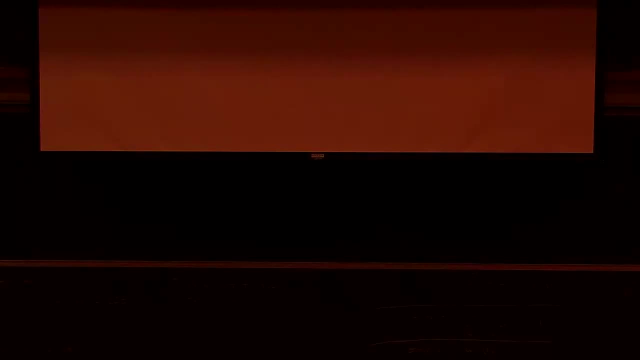 but an element like osmium you can't. Is there a way around that? I don't know. And then you can think about flaws in the assumptions. And then number seven is where best to focus future research. If you wanted to work on this problem, what would you do next? 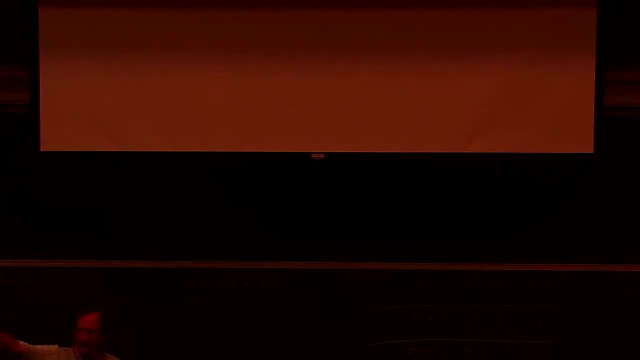 OK, So we have here somewhere group two, back there somewhere, group three there, group four over here and group five- if we get these lazy people out of the front row- could meet over here. We'll have Bill White and myself assist. 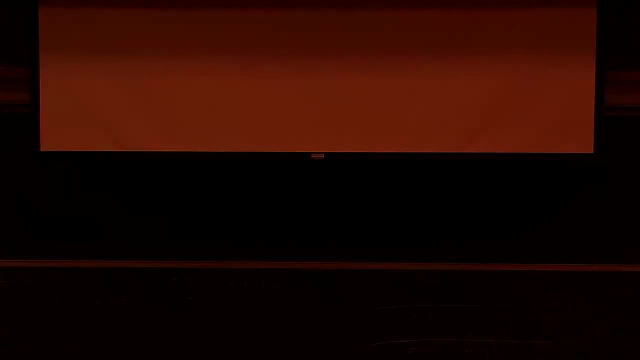 Correct. Yes, You look, troubled You look, But it doesn't look like any huge thing. You get a slight error. You can see that, Hey, Oh, I don't have that. Both Bill and I do, Really Yeah. 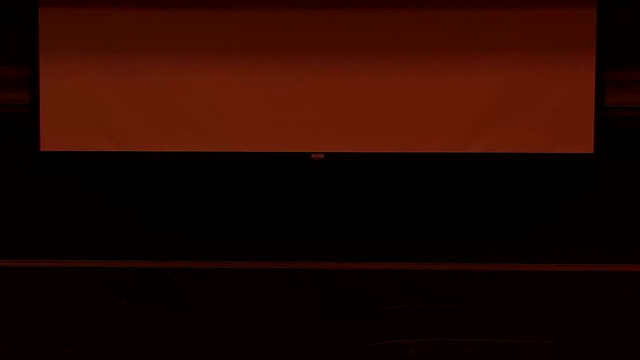 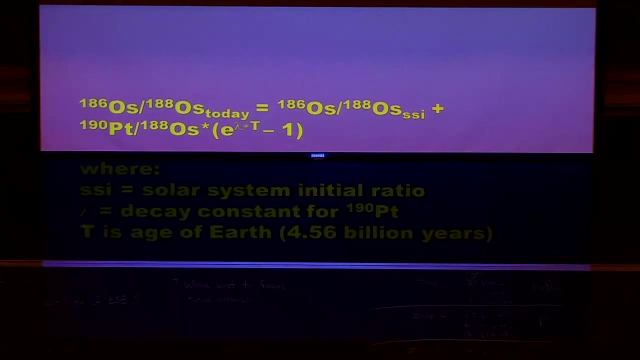 Everybody else does. So I mean the A is just tell people to get to the A, I'm sure, And that will work right. 2.8.. Oh, So in cell A25, or is that right? L25.. 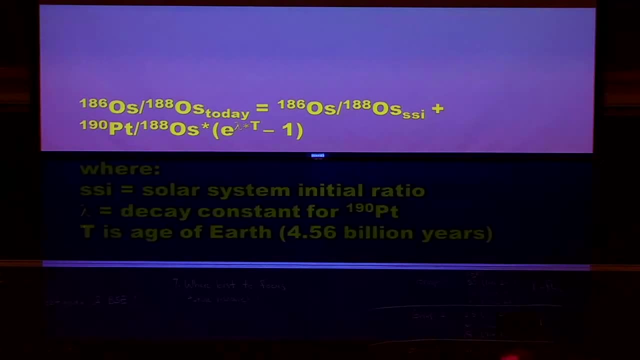 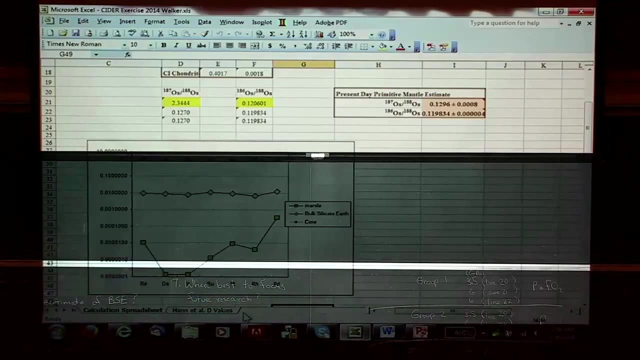 There's an A in front of the number. You should remove the A. I don't think I have that In the KVNR. we've got the skew up somewhere in there. Ah, there it is. You are correct. Sorry about that. 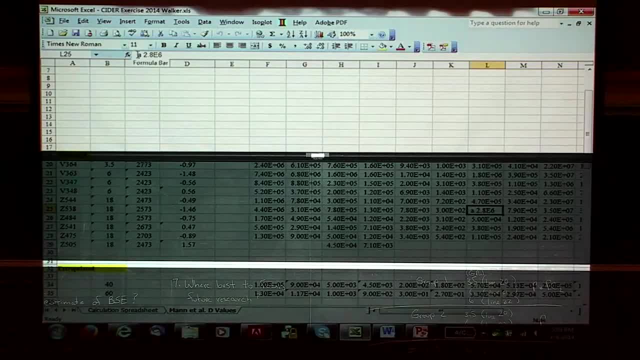 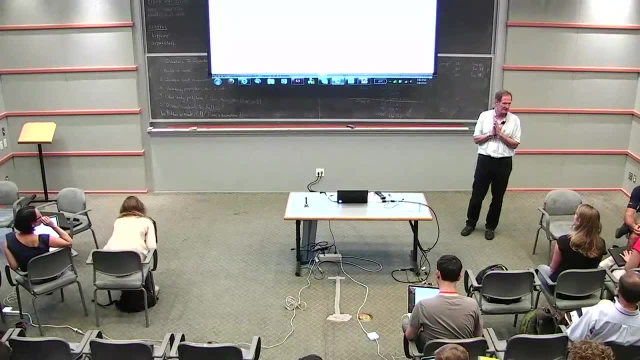 Also, you have an extra line on the platinum data set here. I don't understand that, Sorry. where Go to the platinum data set? Go to the far end. The highly siderophile element abundances in the mantle as a consequence of varying pressure. 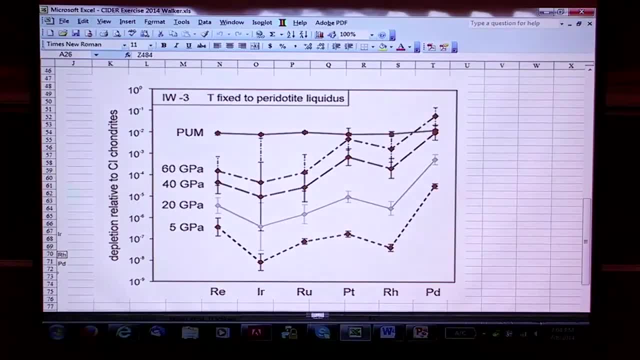 So I told you at the outset you would fail, but we hopefully learned something from our failure, And so now let's consider some of the questions. We just answered question one, So I don't think we need to discuss that further unless some group actually got results that worked. 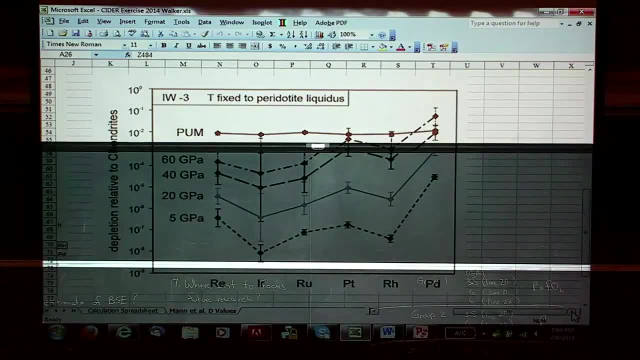 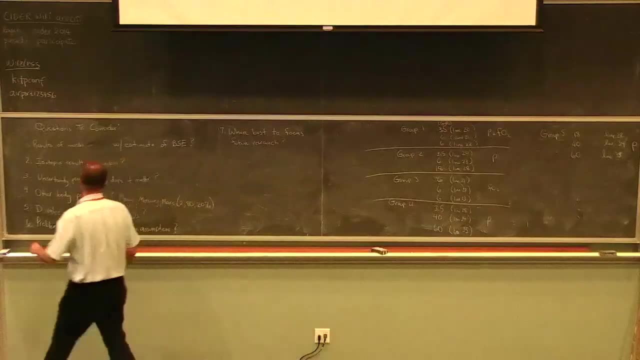 Did anybody? I didn't get a sense that anybody was Ved, did you? I guess we make up our coefficients. Yeah, you can make up coefficients. Okay, so we need to get on so that we're finished by 4.30.. 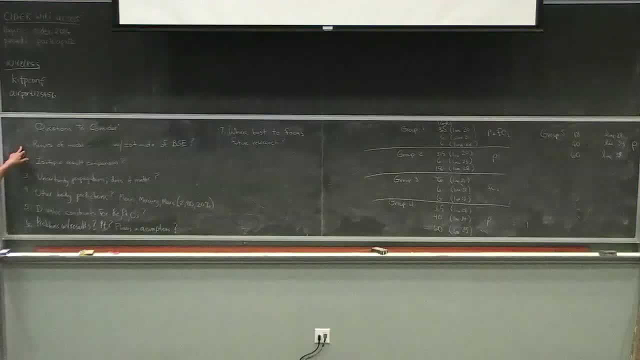 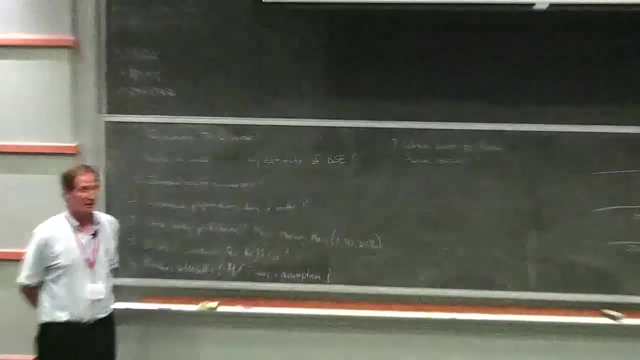 Okay. So none of these models, using these experimental results, produced a bulk silicate earth like we think we have. Okay, number two: Go ahead To be fair, as they go up in the pressure, they're approaching that value. 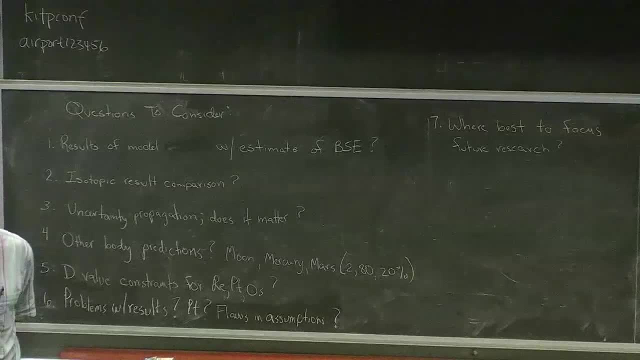 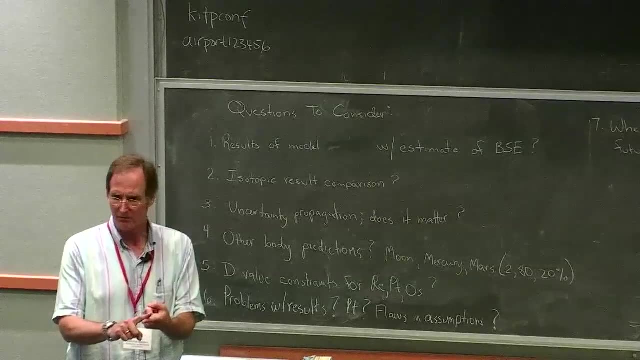 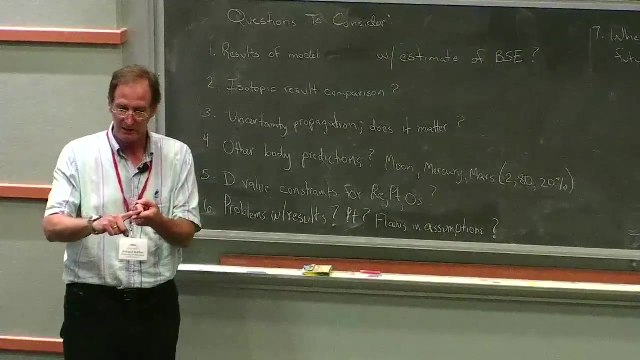 They are approaching. Yeah, Uh-huh, That's certainly true And again, I just want to keep emphasizing- every time I walk by a group, I emphasize- that the people that have worked on moderately siderophile elements are generally convinced that those elements were primarily established by magma ocean processes. 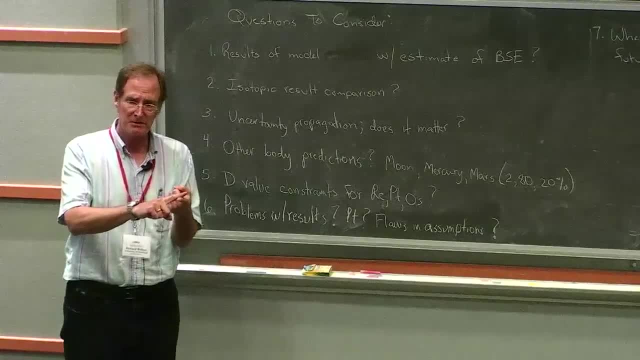 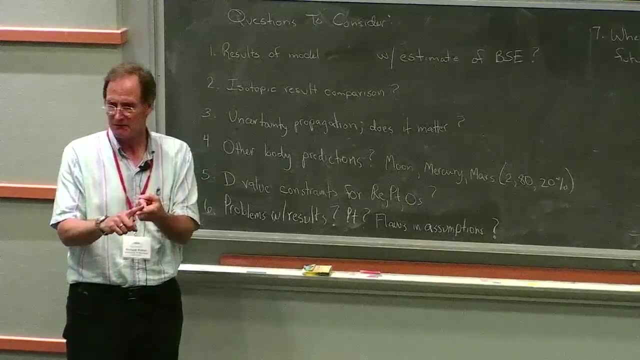 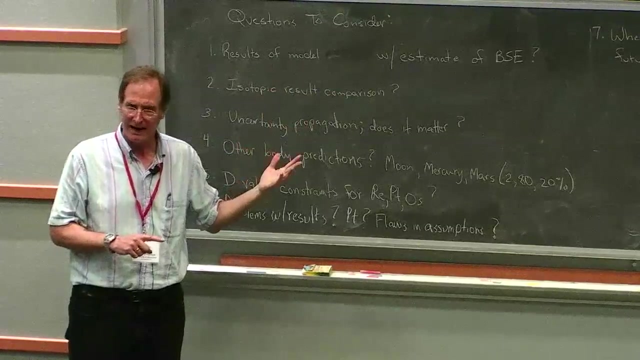 Most of those models are typically in 40 to 60 GPA range. So one of the questions to think about- and I don't think we have an answer to this here- is if it works for moderately siderophile elements- and it works for some of the elements we're seeing here, like palladium. how do we explain the other elements? 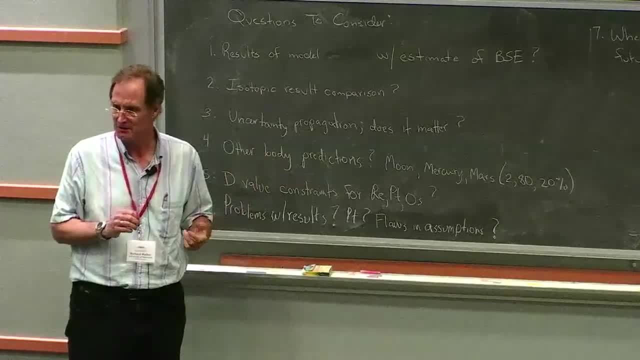 And that's a conundrum that I don't have an answer to. It's something that I worry about, But I don't have an answer to it. By definition, you didn't get the correct isotopic results using any of the conditions. 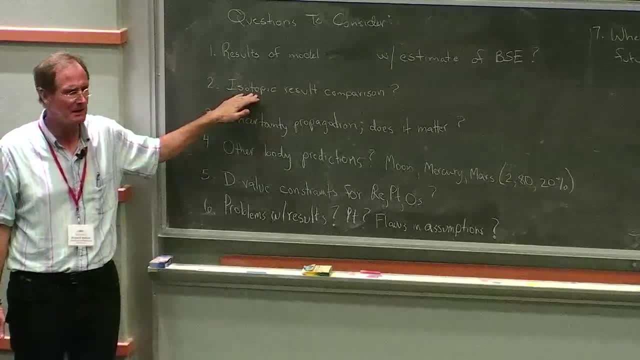 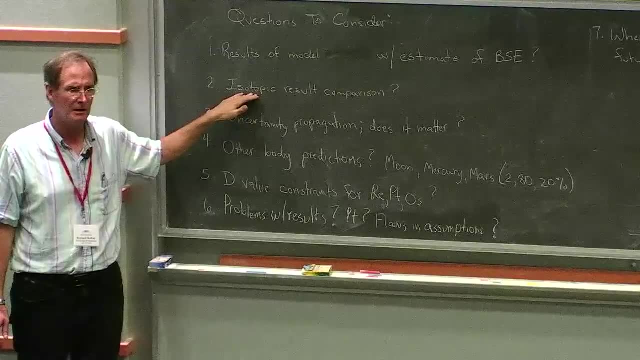 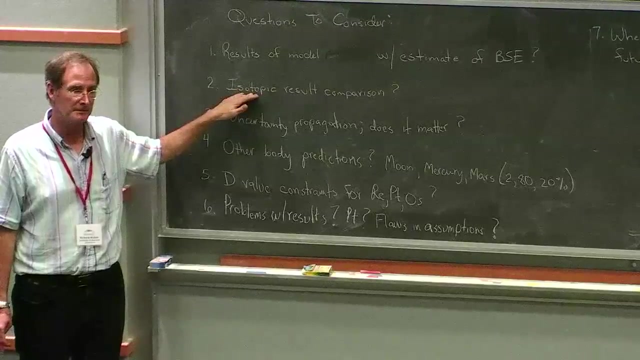 Did anybody get anywhere close to the observed isotopic compositions? Yeah, What conditions. There's quite a bunch of force distribution coefficients, That's okay. Force, I like that. Basically make it fit the measuring composition. Do you get the final mass of the system? 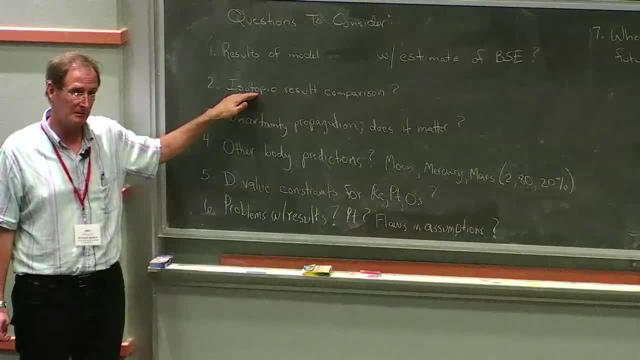 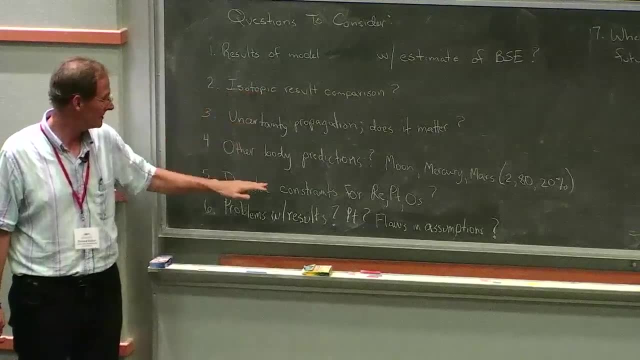 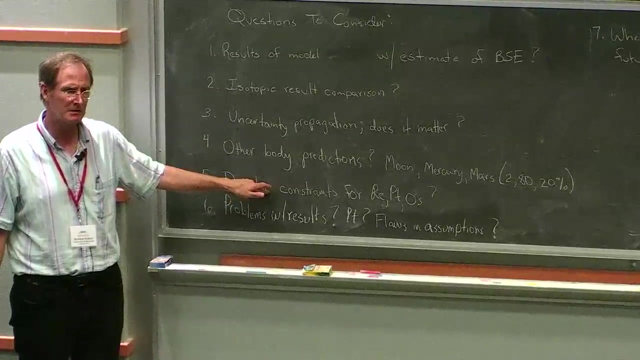 The error of what we've done from mantle, But the does not work so well So you have to actually get it by changing the parent-daughter ratio. So this is getting on to five. Did you do iterative calculations to see how much you had to vary bulk distribution coefficients to keep it within the range of bulk silicator? 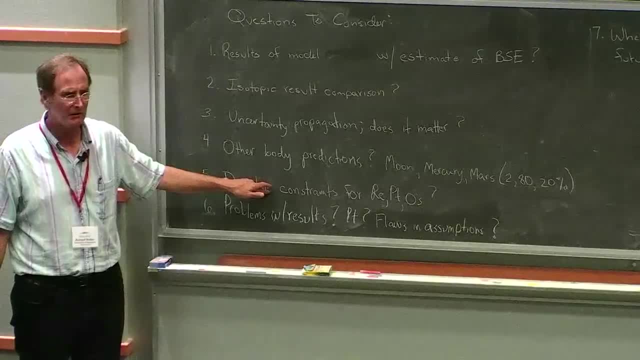 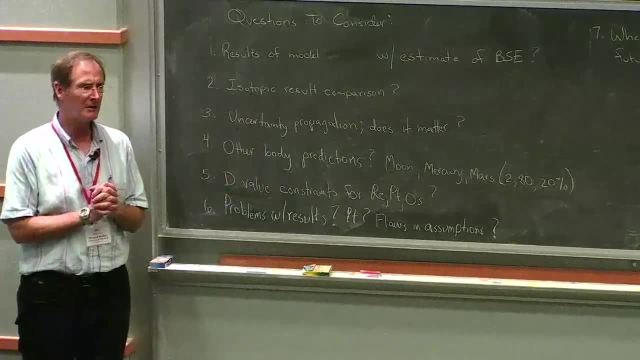 Did anybody do that? Well, that's something we can do on a rainy day if we have nothing better to do. Okay, What are the uncertainties? The Michael Manga question: He was worried about the big error bars, which are probably underestimates of error. 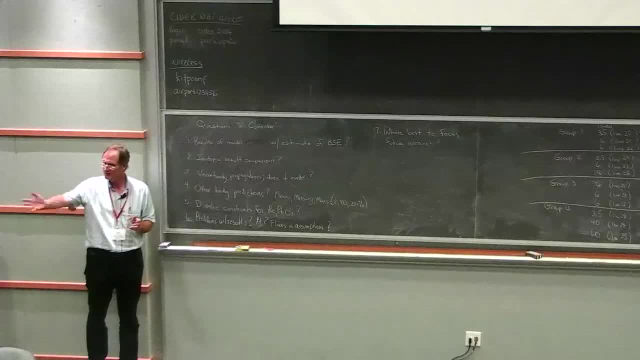 Did they have a major hole here? What's the conclusion? Group one: Yeah, they did. They did. So we tried plugging in the 2016 PA And then we sort of watched the uncertainties in there And some of the matches are pretty close. 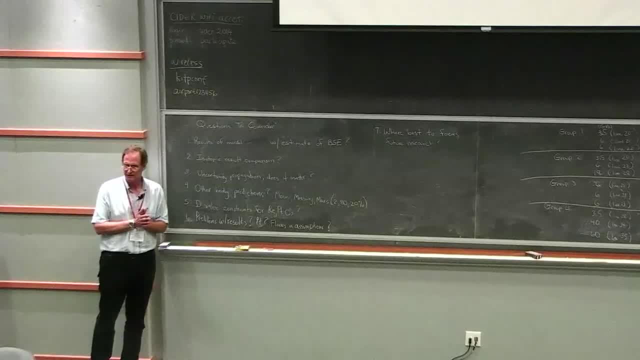 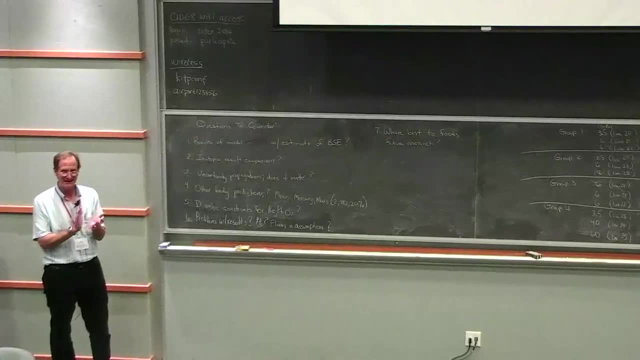 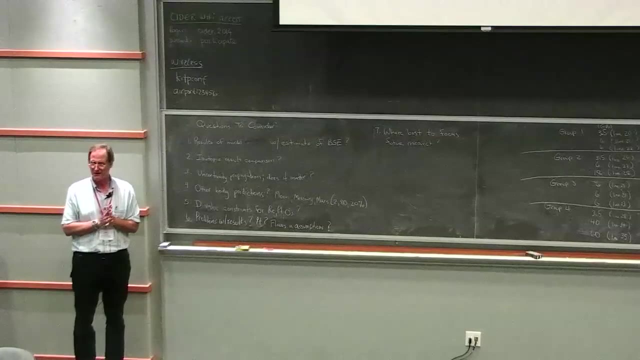 So you got pretty good results. That's not too bad. Hold that up. Everybody applaud. Wait a minute. You didn't say fudge factors, You just said errors. You expanded to the stated errors. right? You certainly didn't. 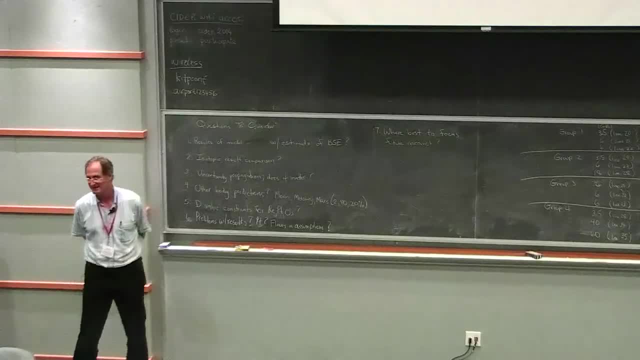 Oh no, Only for four of them. yeah, That's Okay. So group one is the group of cheaters. Now we know that. No, I'm just kidding. 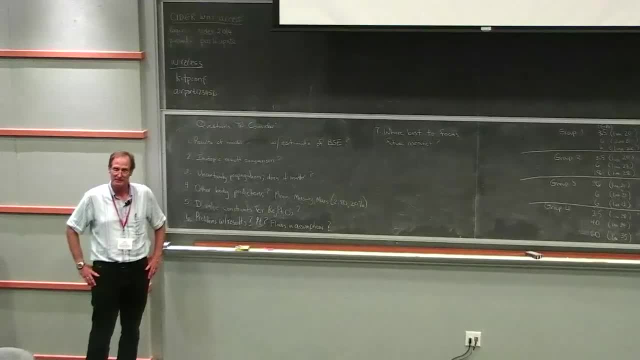 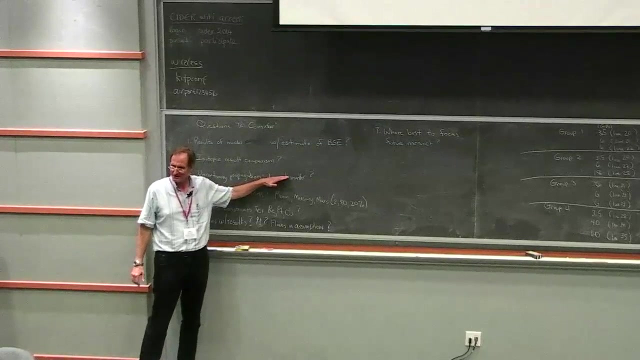 Yeah, okay, So the answer to this, I think, if you didn't fudge it, 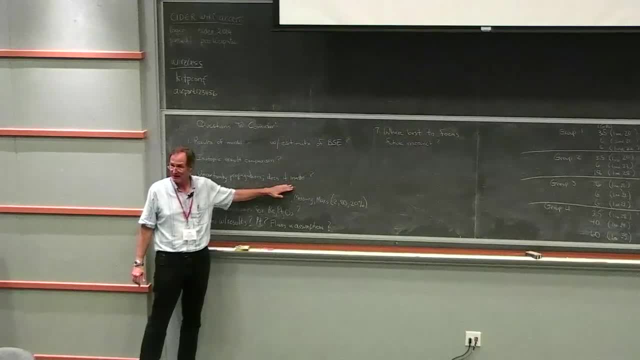 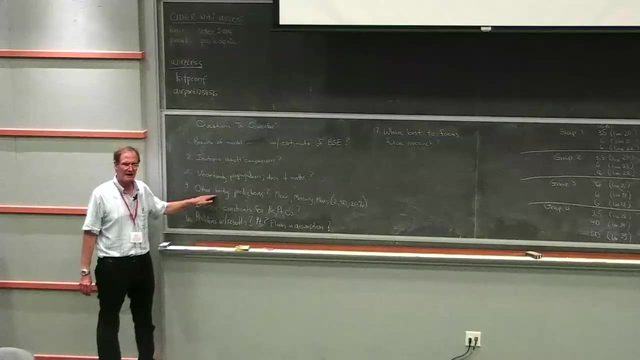 you might say it really does matter then, or it doesn't matter. A factor of 100, that's a pretty big fudge. A factor of 2 helps, Okay. Okay, did anybody group 2 back Back here? What exciting discoveries did you make? 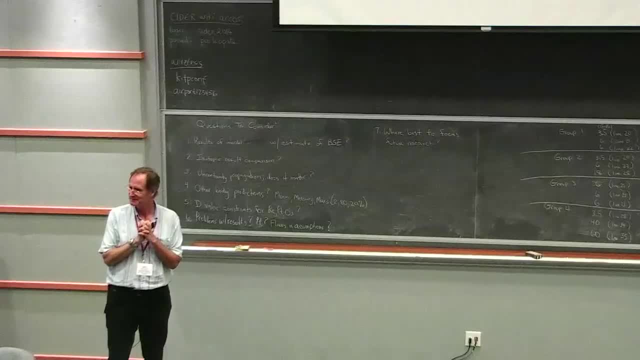 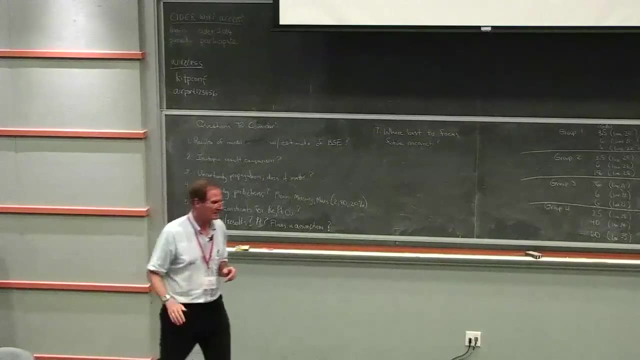 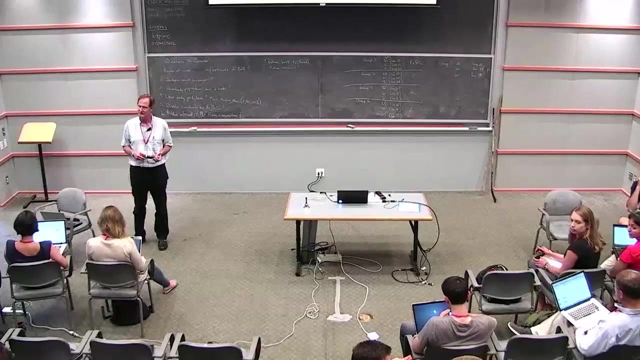 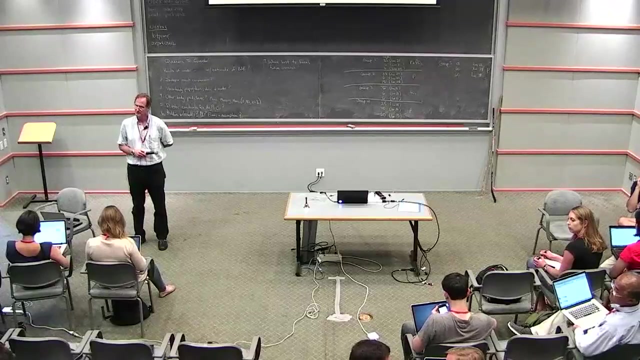 This is the shy group Here. where's the microphone Right here? Do we have one? Okay, yeah, so we didn't go as far along, but looking at the errors that were in the second spreadsheet, we could get the daughter ratios to be close. 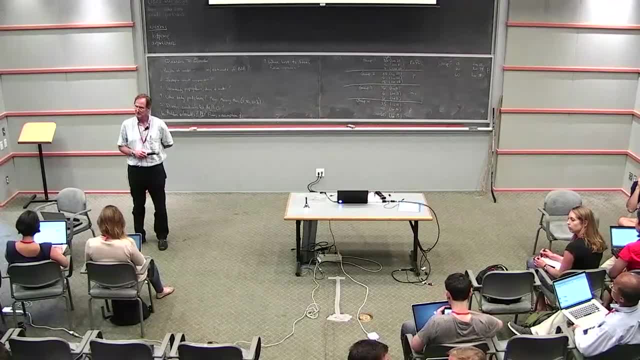 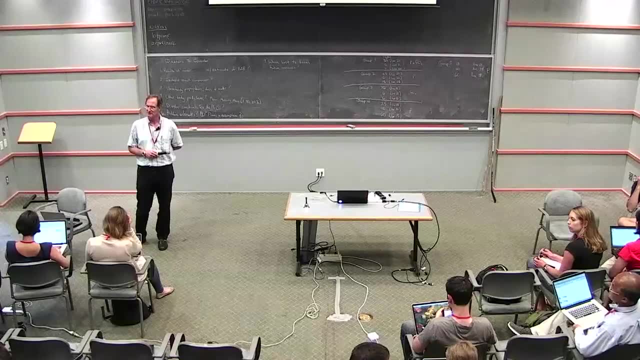 but that's just for osmium. We didn't look at the other ones quite as closely. So could you match the isotopes- Topic composition- but not the concentrations. Is that what you're saying, Right? Okay, Anybody else able to do that? 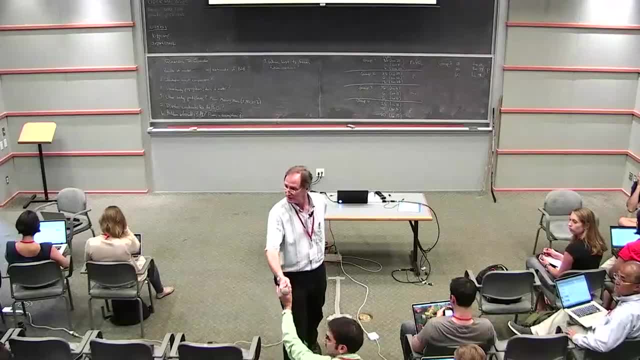 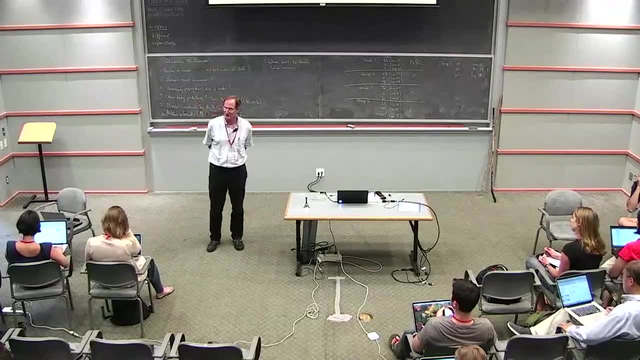 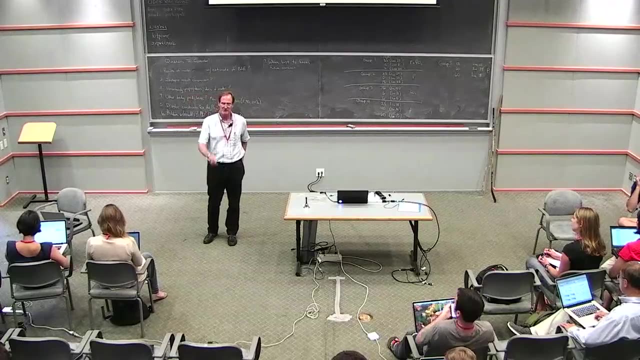 Here. Oh, and I'd like to use match loosely. What's that Match? Consider match to be loose, Loose match, But there were actual error bars in those ratios. Are you just ignoring those actual error bars? Which group are you? 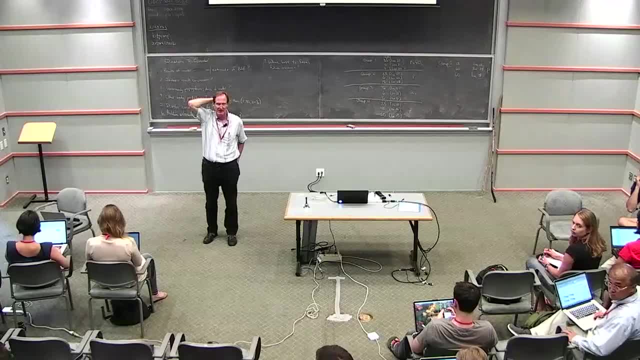 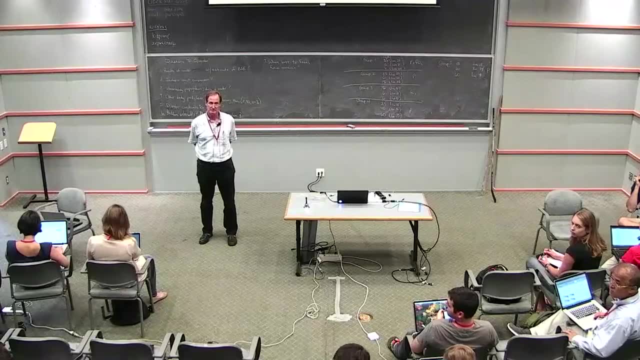 You're group three, No, still part of group two. So we were only varying pressure in ours, And so it was interesting to see that we were getting closer and closer to the bulk silicate earth with our by upping the pressure, but the platinum overshot. 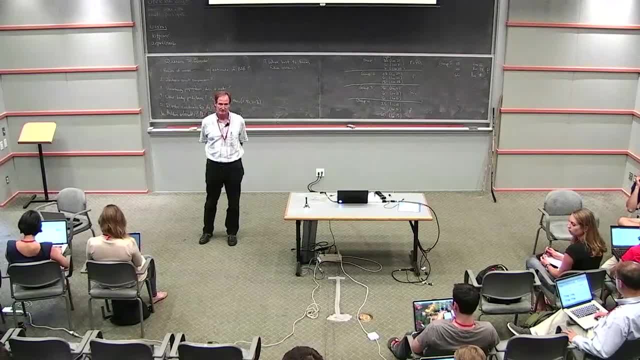 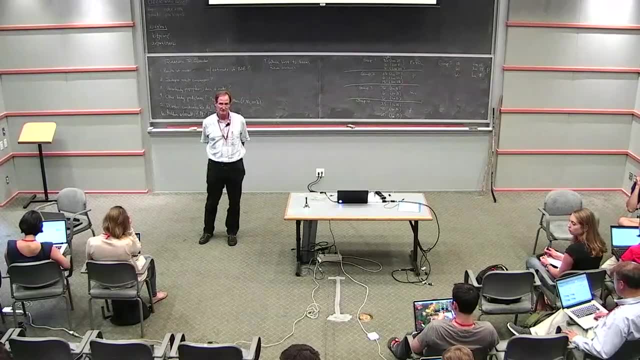 And so that was an interesting point that we discussed with you- was that, even though we are getting closer on many of the elements, because platinum overshoots what we're aiming for for the bulk, silicate, earth pressure isn't the only variable that we have. 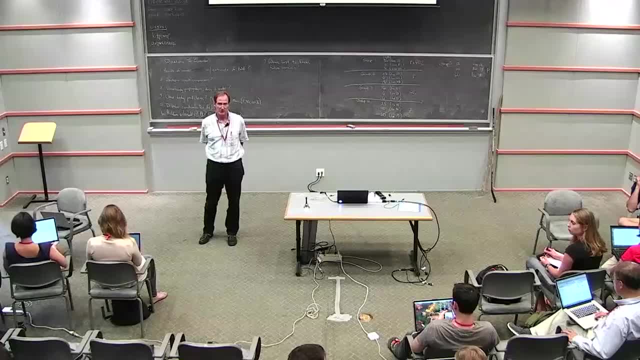 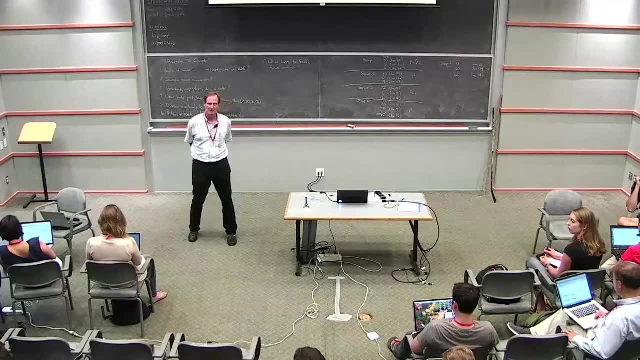 Okay To play with, And so I want to add that. So an overshoot is a problem. Sorry, palladium, not platinum. Palladium Platinum gets up there too, So but palladium is the most offensive of the ones in this. 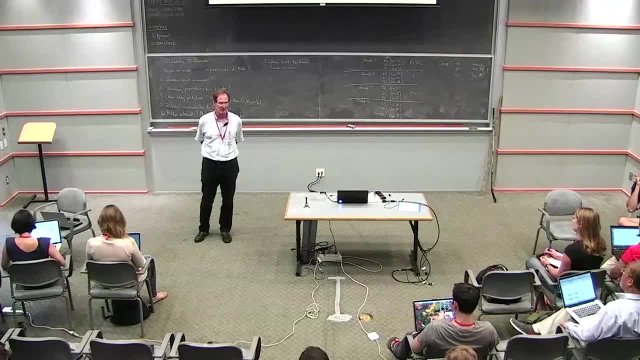 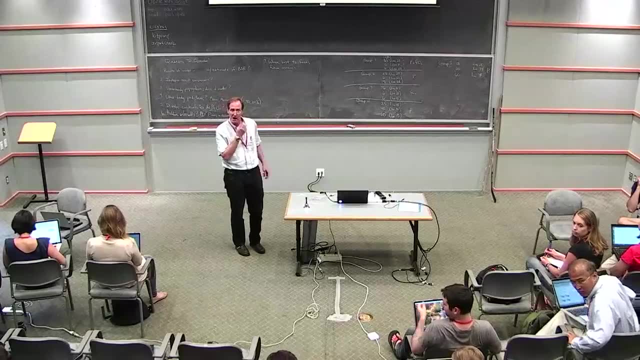 Yeah, in this set of distribution coefficients. How did group three do? Group three report please? We found that we didn't really get anywhere near it by varying the oxygen fugacity at 6 GPA. However, for the highest, 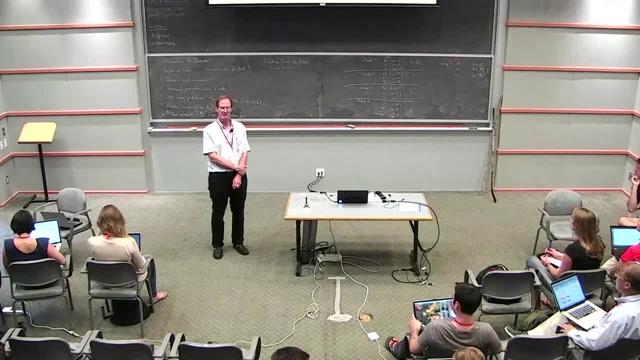 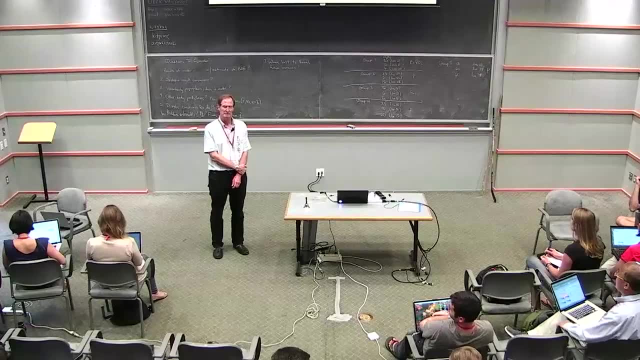 So is that saying? So you're saying oxygen fugacities. different oxygen fugacities didn't affect it much, or It did affect it, but none of the values that we were given were anywhere close to the bulk silicate earth or the osmium ratios. The best one was the highest oxygen fugacity of 0.56.. And we found that if you use the lower bounds of error you can make the osmium and iridium match. for the bulk silicate earth You can find a value within the error that does match, but none of the other ones are even close. 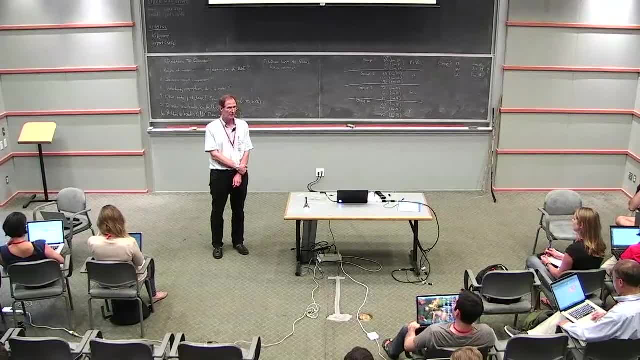 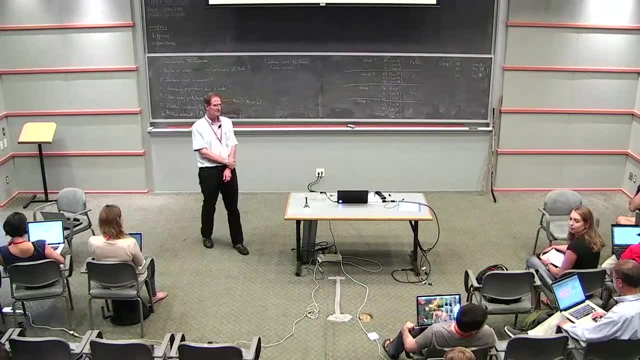 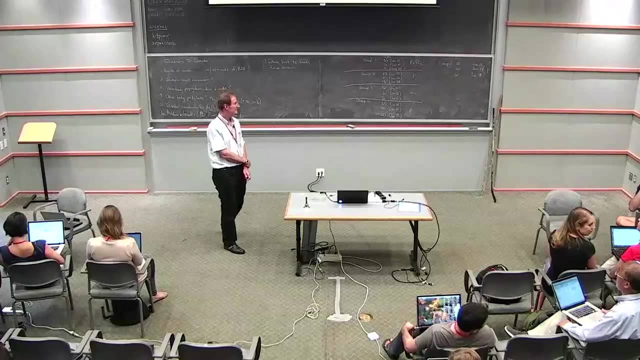 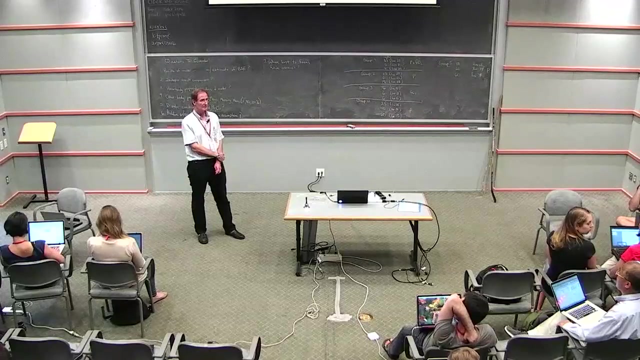 So that's the best we got. Okay, thanks, Group four. Yeah, same sort of thing. So we can fudge it to get it, but not by not anywhere near the orders of magnitude away from the partition coefficients that have been measured. So yeah, And you can play tricks like sort of varying, as you did. You can play tricks like sort of varying the sort of parent-daughter ratios, to try and match the isotopes, But you are playing. It's not necessarily based on any of the measurements we have. 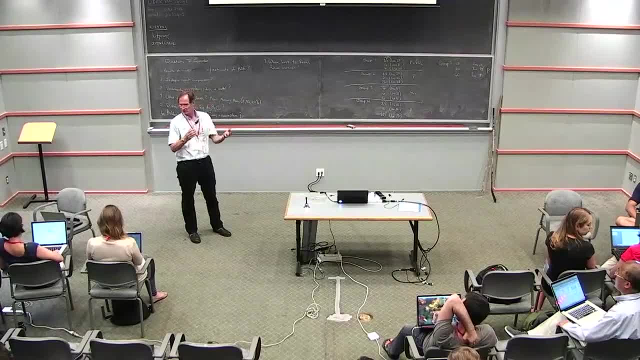 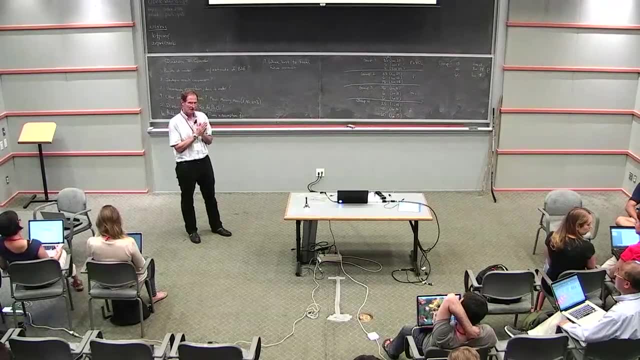 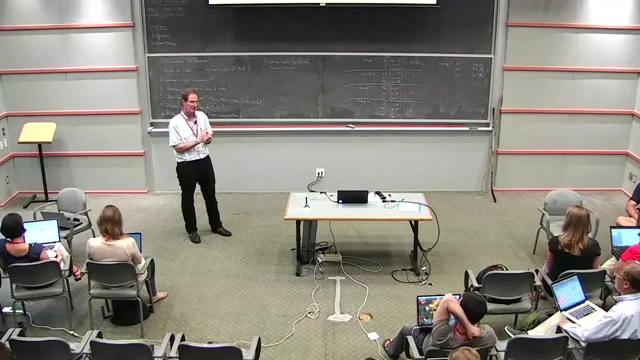 Yeah, but you can turn that around. And again, if you want to match the isotopic composition, you can see how much or how little you can change the distribution coefficients to match the observed data And you can come to conclusions on how much variance you can have in the distribution coefficients. They usually end up much tighter constraints than experimental systems can match. The uncertainties in most experimental measurements like that are usually much larger than would be allowed. from the variance in the data I have a kind of I don't know if this is a science or philosophical question, but why would it be that the Earth 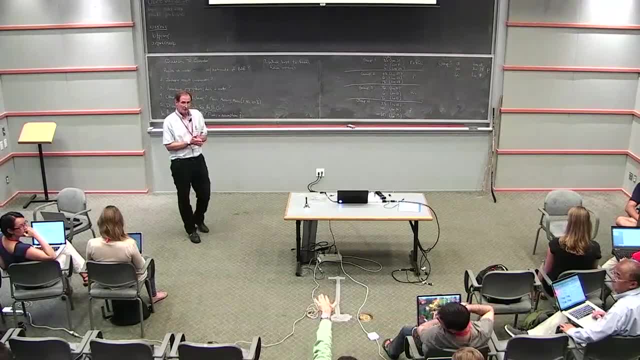 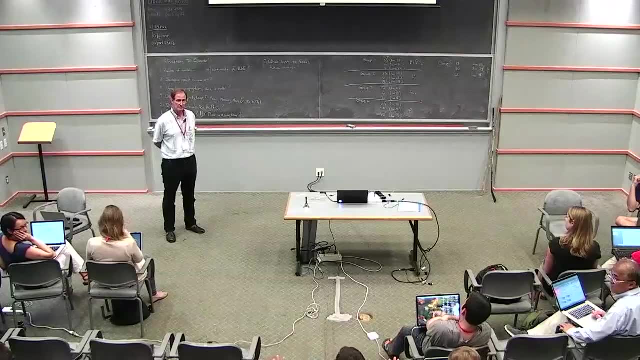 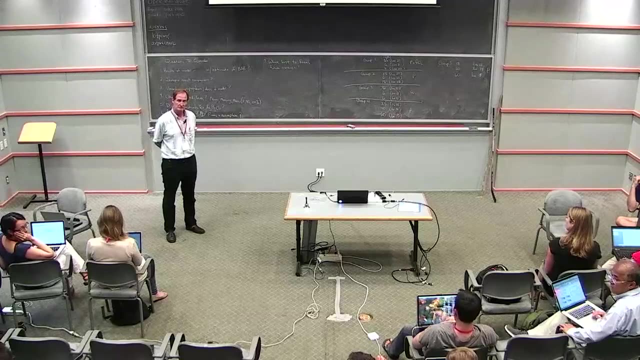 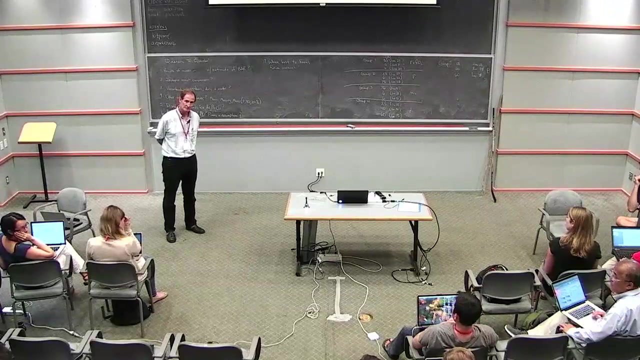 You know, you have these concentrations that are all the same, without a plot right, And then you fudge these partition coefficients to make this come out of something that doesn't look anything like that. Why would that coincidence take place? Is there any like ab initio reason to believe that these elements would actually partition in the way that's required to reproduce a constant concentration? 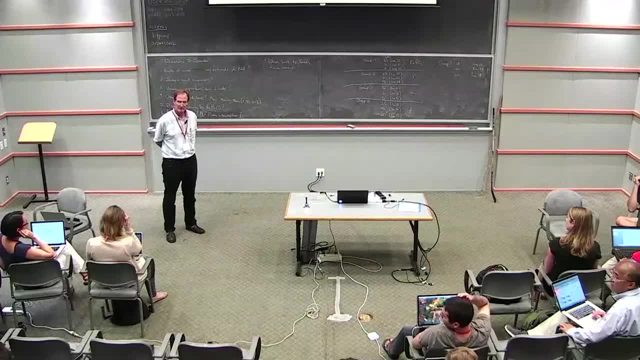 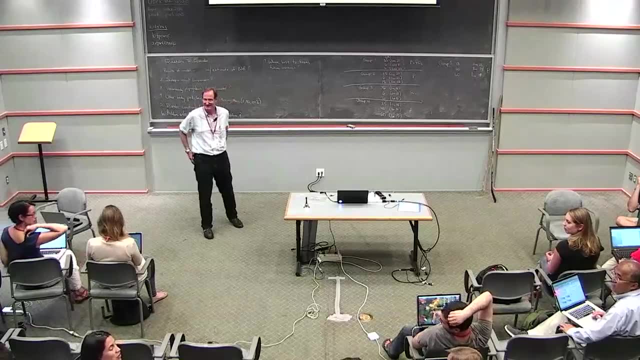 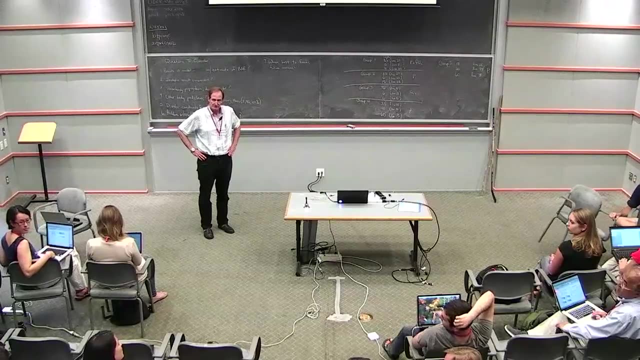 I'm not qualified to answer that question, Liz or Anant Preverse? I don't think that's the No. the reason, the initial motivation for a lot of the research was that this Murphy paper that was alluded to the idea that in a magma ocean, as things get really hot, 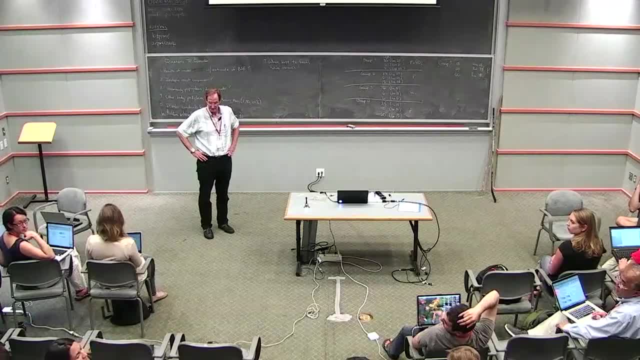 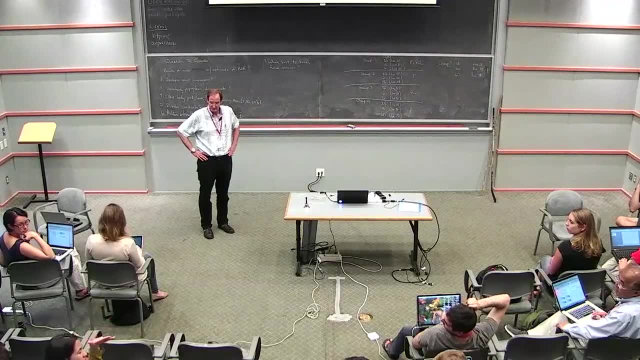 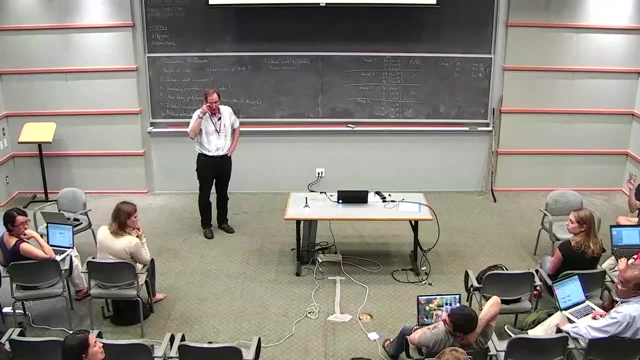 and the liquid metal and the liquid silicate approach super critical behavior. as the liquid silicate and the liquid metal become more and more similar, all Ds, all partition coefficients, will converge to one, And so the original ideas about why a magma ocean might satisfy the thermophile element problem. 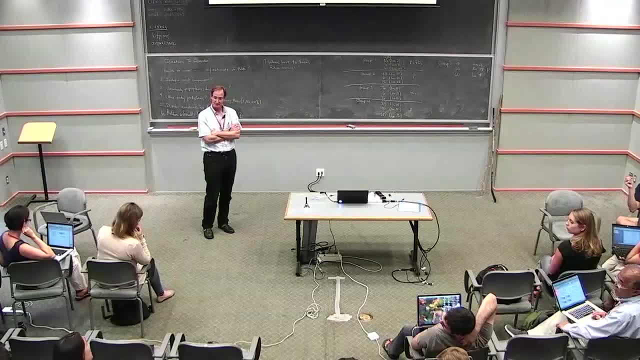 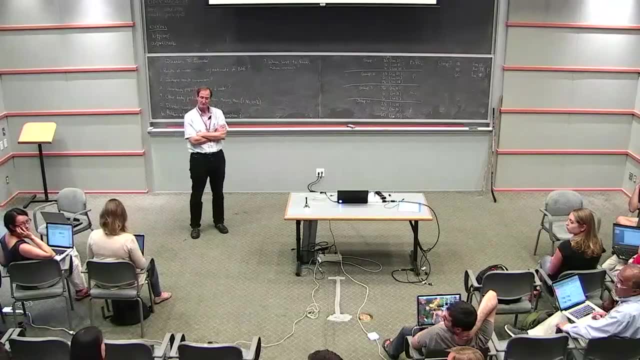 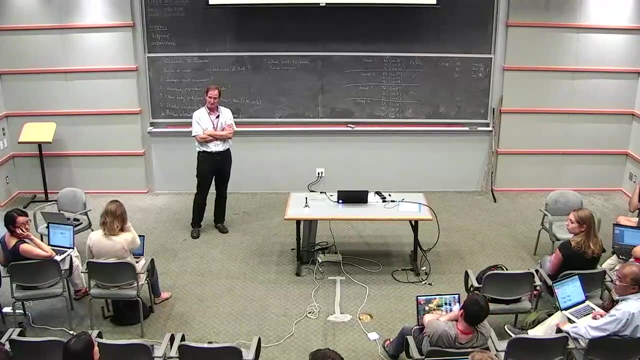 which, as originally formulated, wasn't so focused on the platinum elements or the highly thermophile elements, but focused on Ringwood's observation that the one atmosphere partition coefficients can reproduce the moderately thermophile element abundantly. And then this idea that you have a really hot planet and a hot magma ocean. causing the partition coefficients to become less and less similar, And so the original idea about why a magma ocean might satisfy the thermophile element problem which, as originally formulated, wasn't so focused on the platinum elements or the highly thermophile elements. 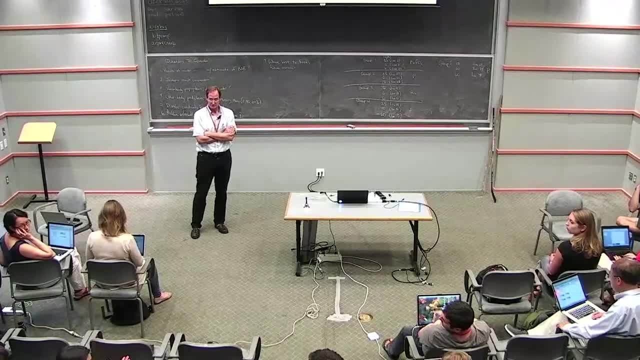 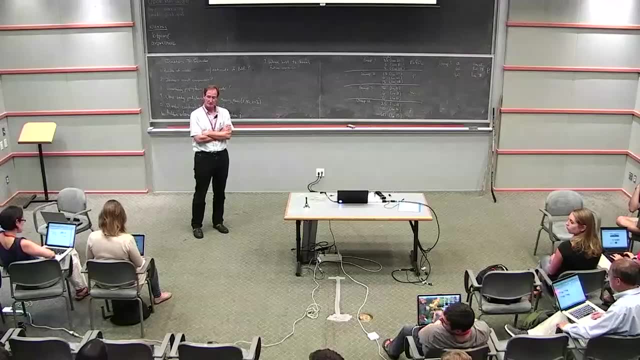 but focused on Ringwood's observation that the liquid silicate approach super critical behavior. as the liquid silicate approach super critical behavior, and then the fact that when this went to be investigated, if people looked at how these are valid and they do converge. 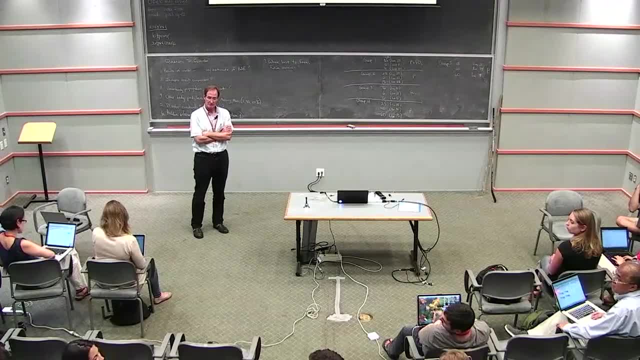 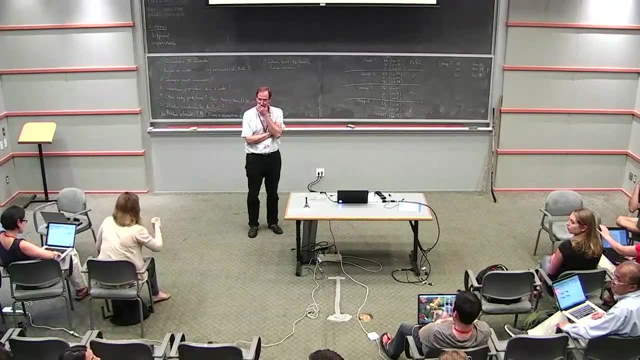 that's following the thermodynamic predictions you make. So that's the. I don't know if you said it's perverse. I don't know if it's perverse, but that was the idea I think of why people thought that magma ocean conditions. 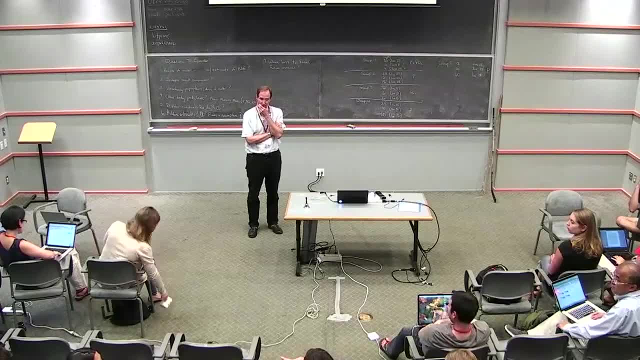 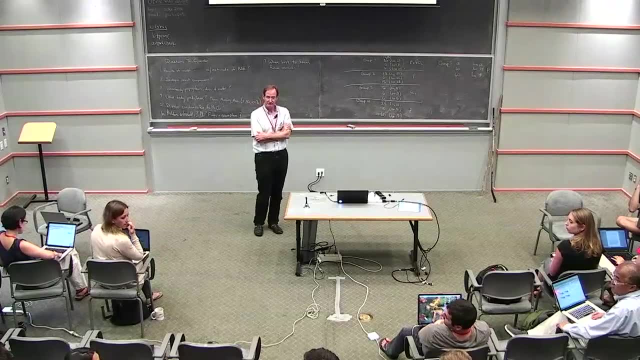 might cause the partition coefficients to converge. But if we had all the partition coefficients equal, we wouldn't reproduce. that would we. Yeah, you would get. Yeah, Yeah, Yeah, that's a requirement. So, group five: how did we do? 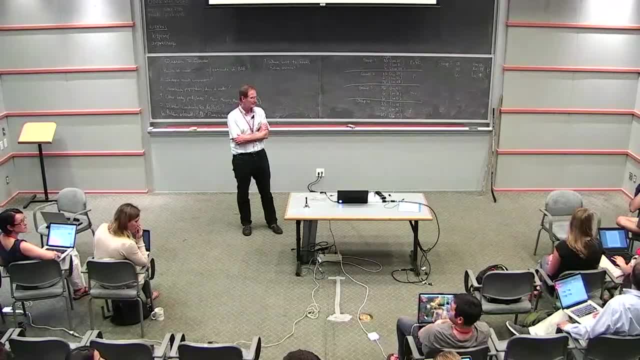 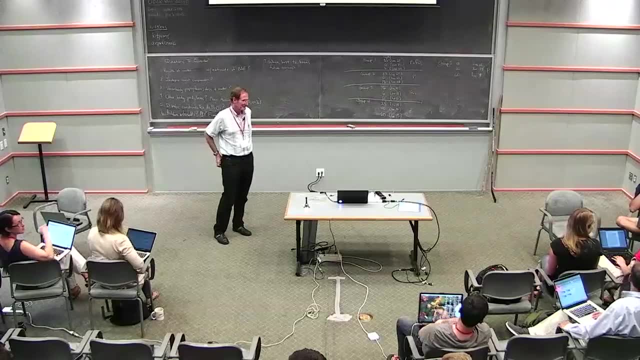 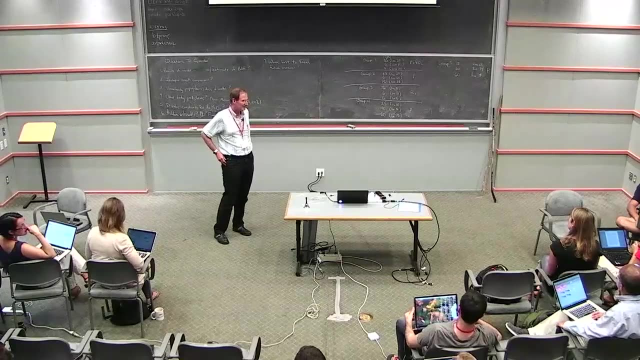 What did you learn? group five: Come on something new. Do you have something new to add? You had, on average, the highest pressures, so 18,, 40, and 60. So you certainly would have had the same outcome as group four for 60.. 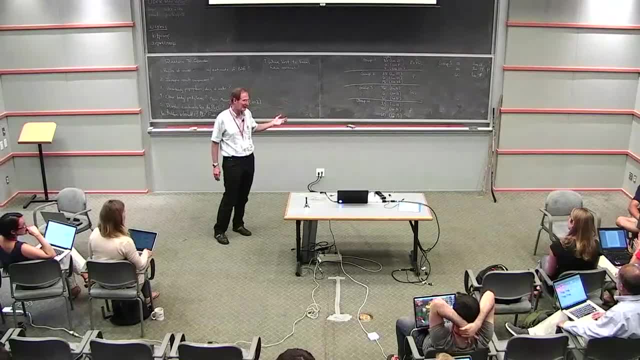 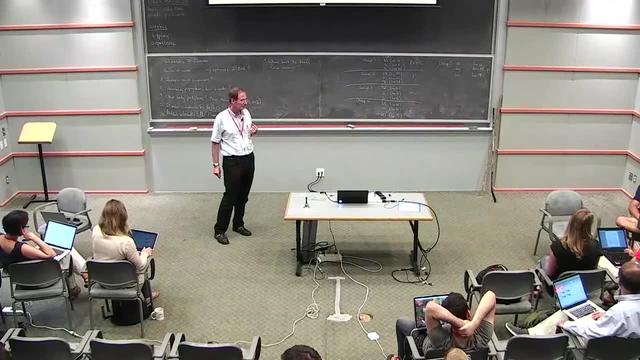 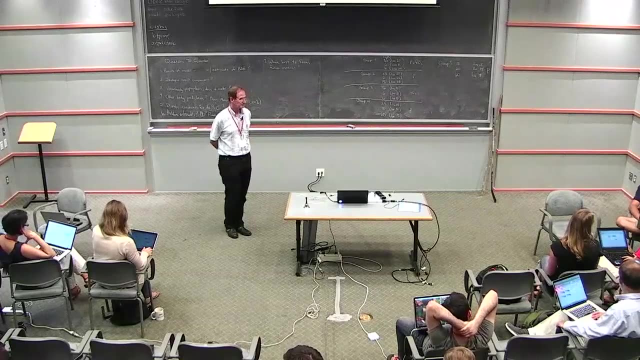 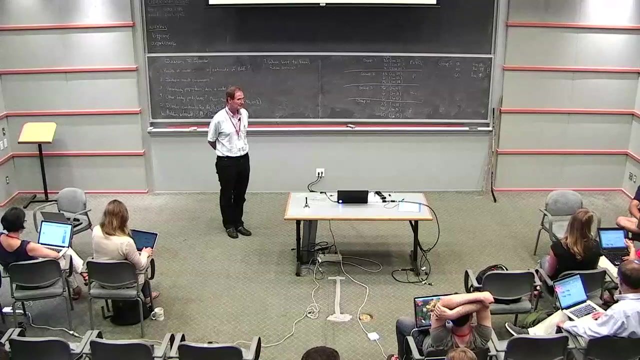 And presumably palladium, excess. Yes, Yes, palladium and excess. The result is pretty much the plot that we saw on the Excel figure. So we know that the all of that figure that they show they give a constant FO2 of iron, let's say minus three. 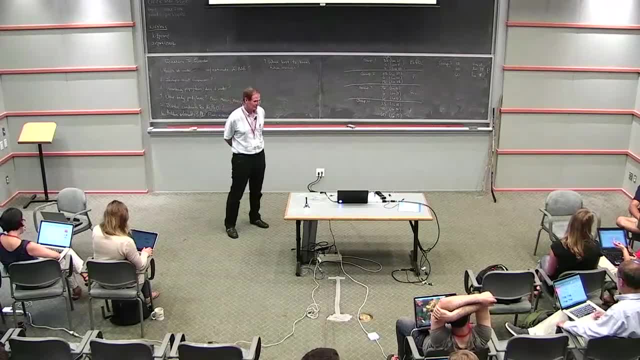 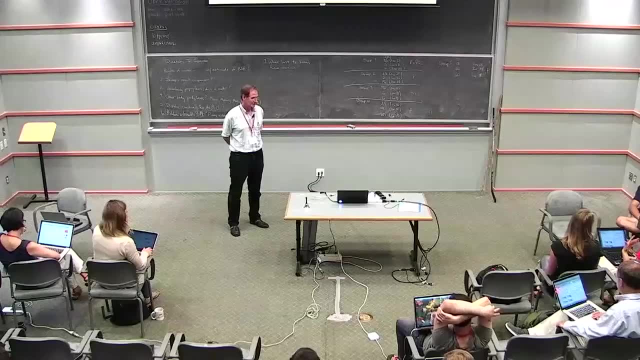 which is lower than anything- any of the data points that they have in spreadsheet at all. But FO2 goes in the wrong direction to help us with this problem, Mm-hmm, And you know we're in favor. 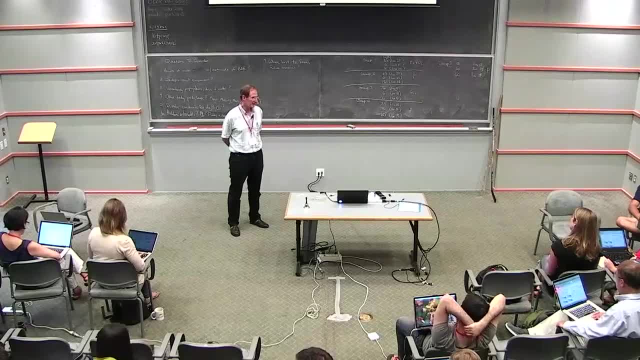 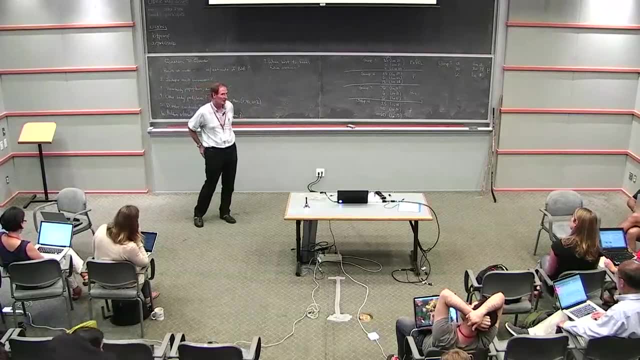 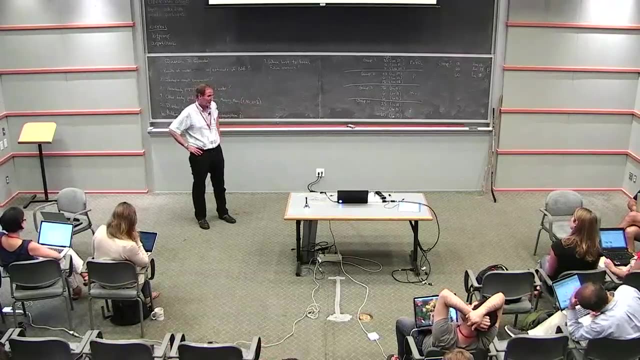 So does group five think that that's a problem? I mean, if we get to the final question, where to focus future research, if you, heaven forbid, decided you wanted to work on this problem, is that an area that would be appropriate? 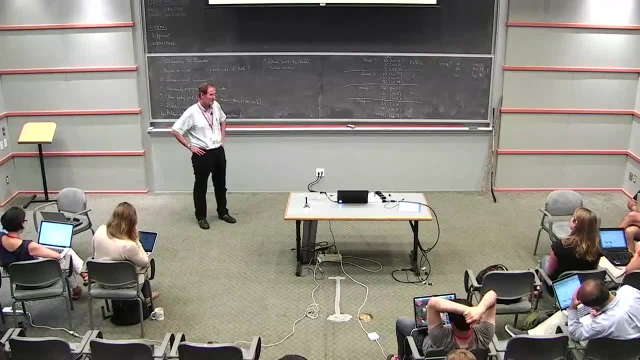 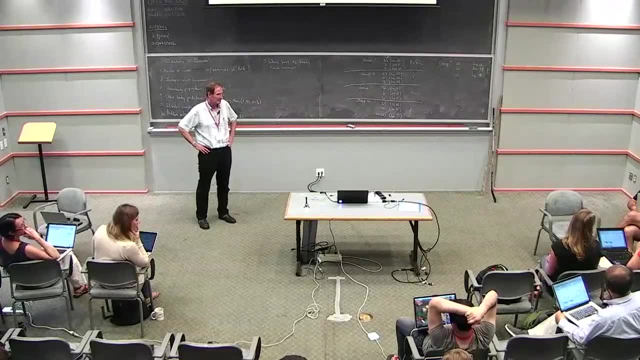 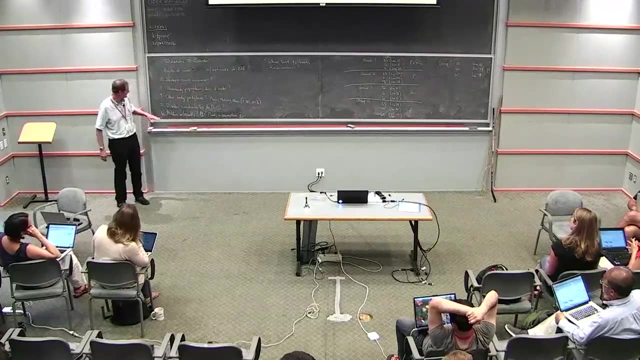 Is that trying to change FO2 conditions? It doesn't look like it's going to solve the problem. Okay, But it's true that it hasn't been tested, Okay. Okay, And I know we're running out of time, but I know a few groups. 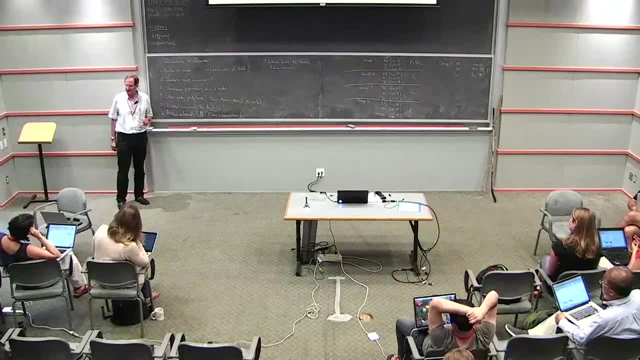 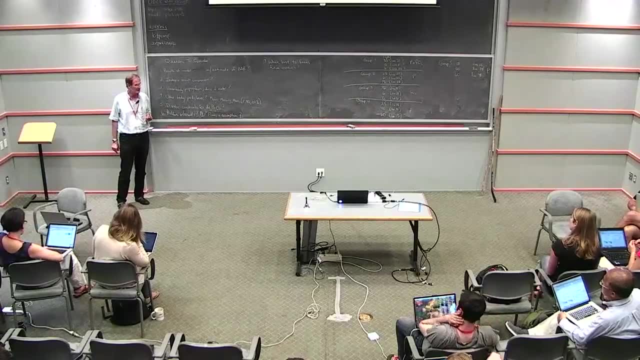 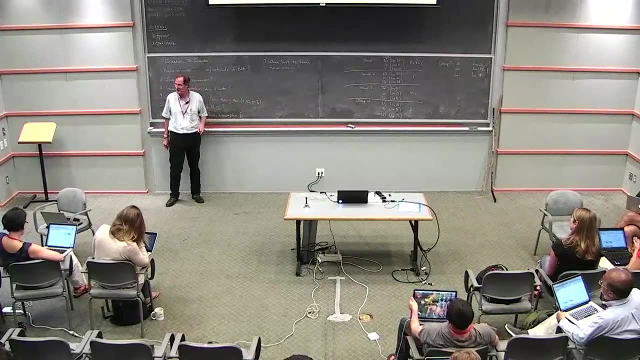 we talked a little bit about predictions for other planetary bodies. Anybody want to comment on that. They have different mantle-to-core size mantles, Very dramatically different from about 2 percent core for the moon, 80 percent for mercury. Would this have a major effect on highly siderophile element abundances? All things being equal, You of course would be partitioning at probably very different pressures for Earth and temperatures- probably different temperatures, And then you would have the proportional difference in the size of the silicate reservoir. but that would have a relatively mild effect on features. 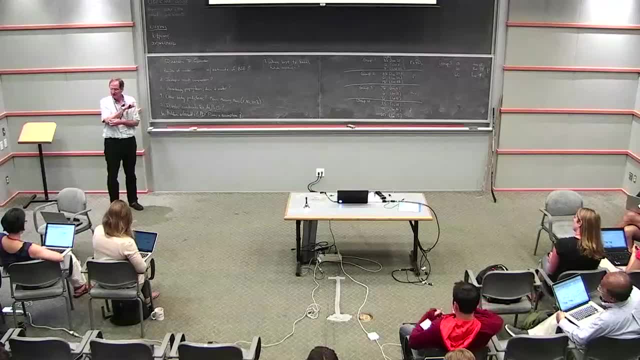 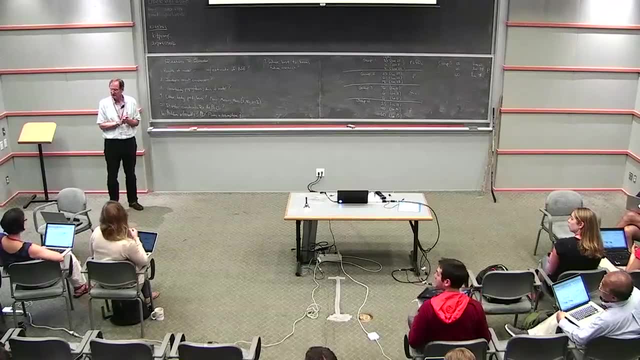 but not particularly radical ones. that is stable, modest impact on the final concentrations. I think if you plug different numbers in- You guys did that- What did you find? You plug in a low number, a high number, how much does that vary the concentration? 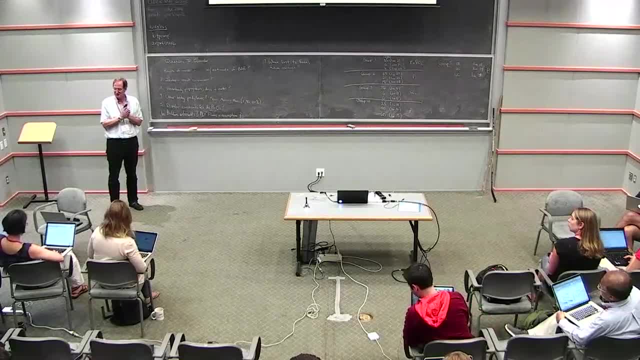 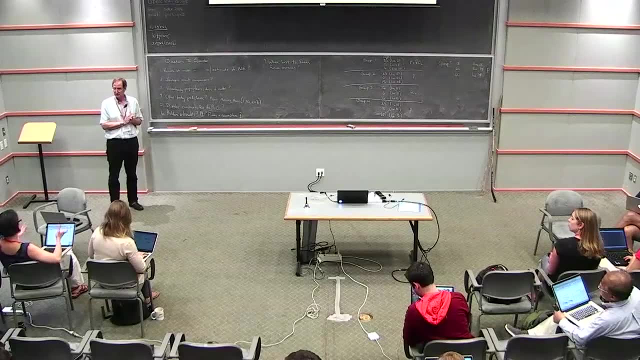 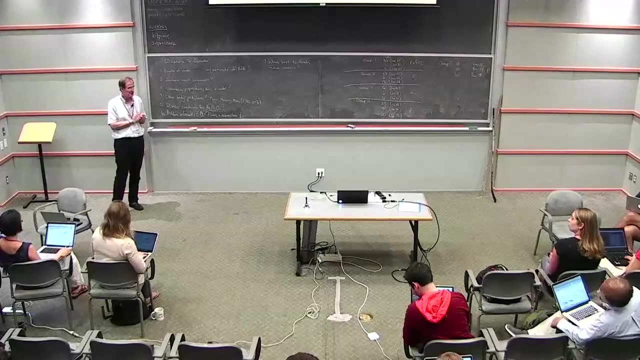 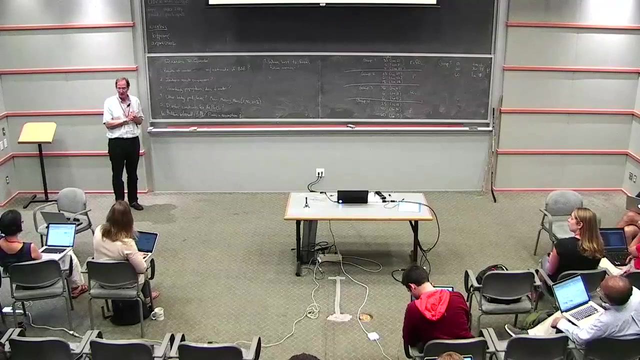 Well, I'm not asking if it's better or worse. How much does it change it? This would be a prediction, for It doesn't change the pattern shape, But that would maybe suggest if you went to Mars and you got some mantle samples. 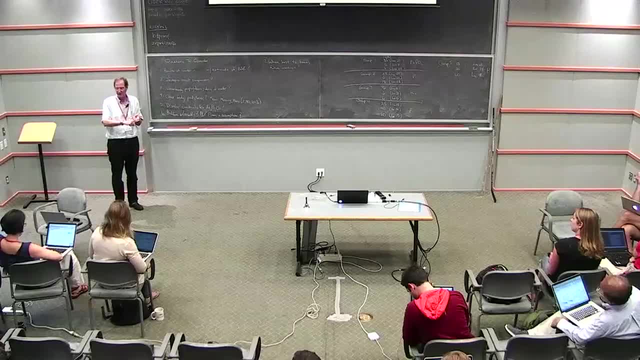 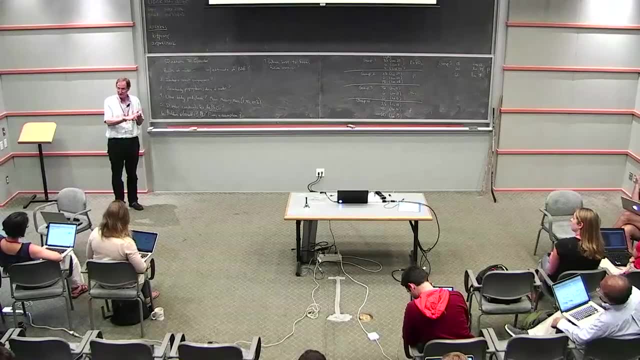 and you went to the Moon and got some mantle samples, and you went to Mercury and got some mantle samples. if this suite of elements were all set by the same type of process under different, under different conditions, you would expect different concentrations, correct. 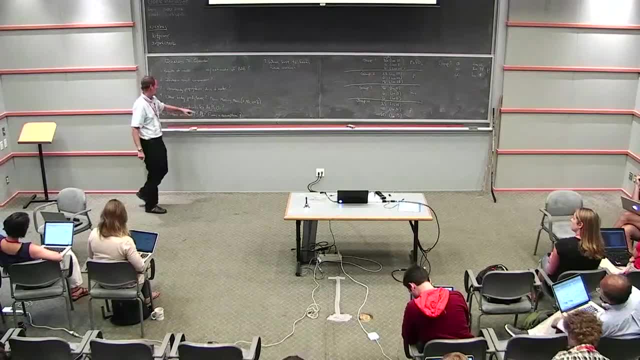 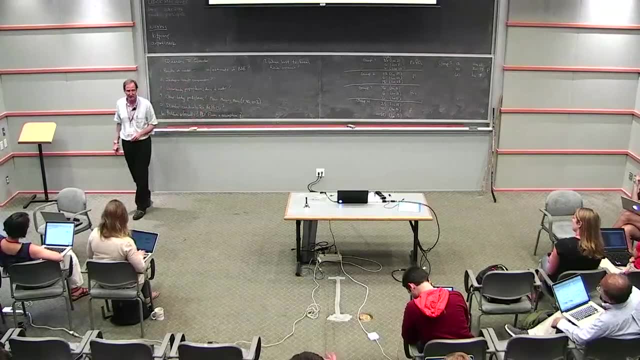 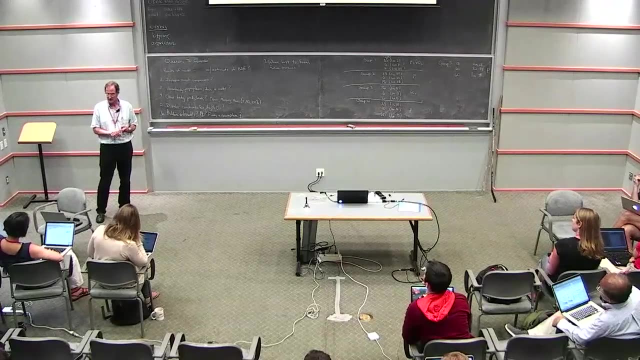 Probably, And what I told some of the groups is we actually think we know the highly siderophile element content of the lunar mantle and the Martian mantle And, amazingly enough, the Martian mantle looks frighteningly similar to the terrestrial mantle, which is a problem. 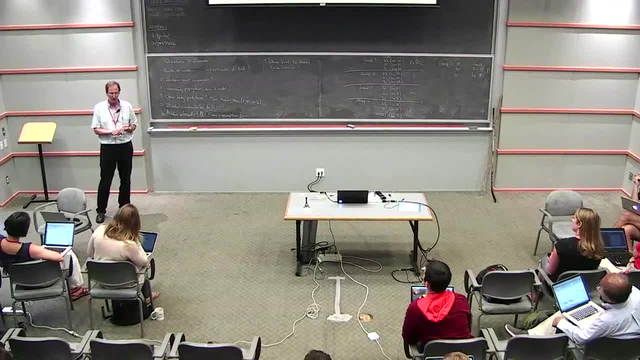 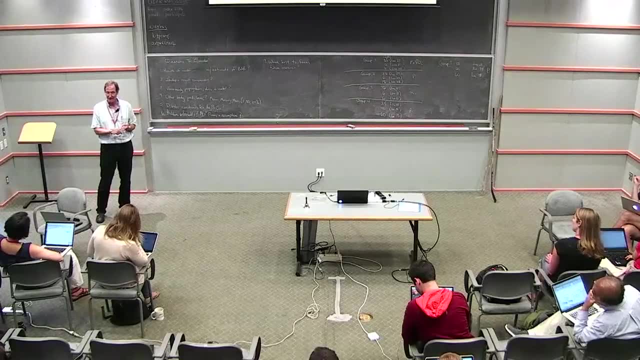 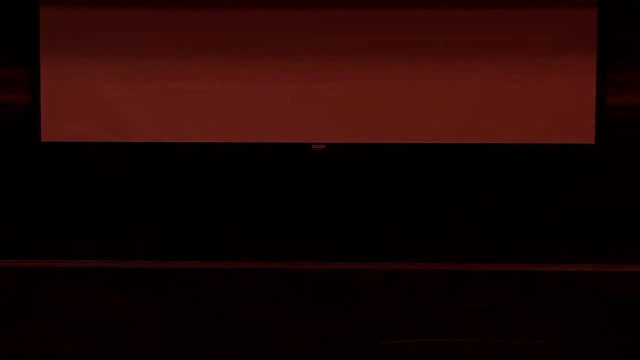 It's a problem for me- And the Moon looks quite different. In both planetary bodies it looks like The highly siderophile elements are in chondritic relative proportion, And that's based on the fact that both the Moon and Mars have probably chondritic osmium ice positions today. 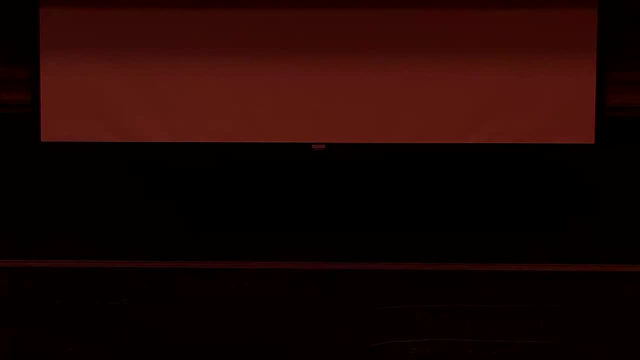 So that's an assumption, then, based on ratio of two elements over solar system history, The Moon has much lower highly siderophile element abundances in its mantle than the Earth, which is an interesting observation. Okay, So flaws in assumptions- I think we've talked about that in the different groups. 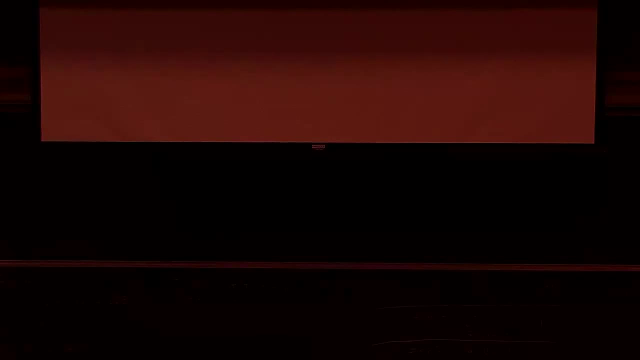 but there's lots of problems, one of which we're using fictive osmium partitioning data. That's a bit of a problem. So if we were to redo this and we had an unlimited budget, we might want to somehow work really hard. 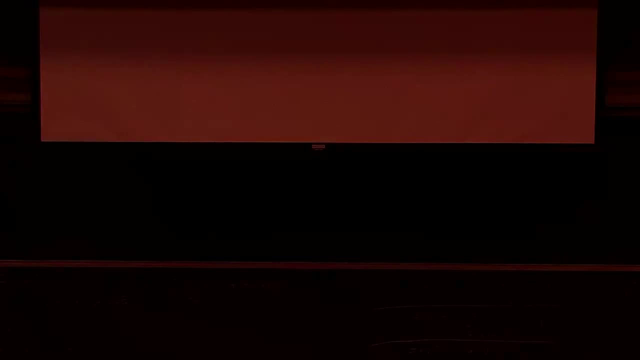 to get osmium into the experiment because it's very important as an isotopic constraint, but it's very difficult. It's a very complex element experimentally. What else would we want to do if we had an unlimited research budget, and we're really interested in this? 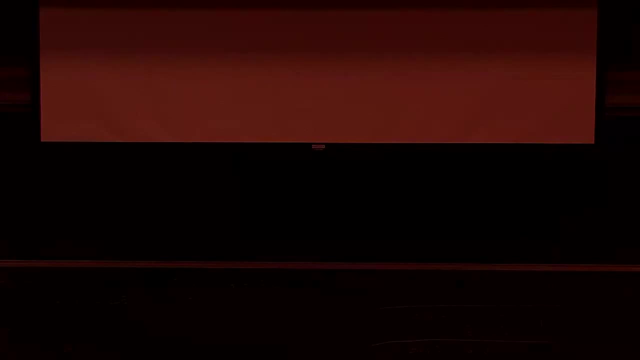 Liz, you practically have an unlimited research budget and you are interested in this problem. I think that a lot of effort should be invested in doing experiments at pressures relevant for magma oceans. The, The data up to 25 GPA seems moderately to converge or make predictions about magma ocean conditions. 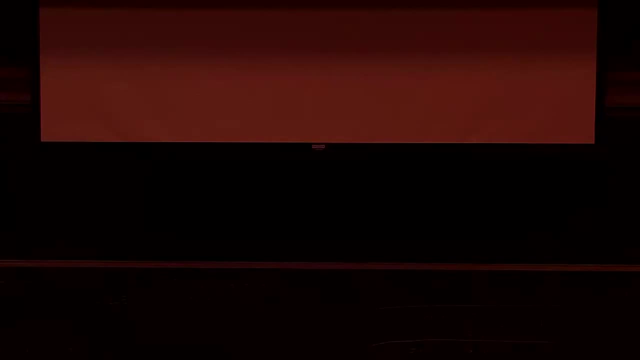 but everything at 60 GPA is an extrapolation. I was just talking, We were just talking about papers that have come out showing a big kink in the partitioning, the effect of pressure on partitioning. that would say that you know. 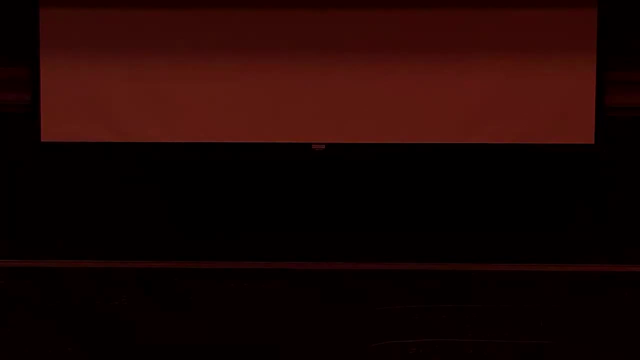 you can't extrapolate from below 25 GigaPascal up to say 60 GigaPascal, But what I point out is the big break in slope occurred where you have a change in the type of apparatus the experimenter got in. 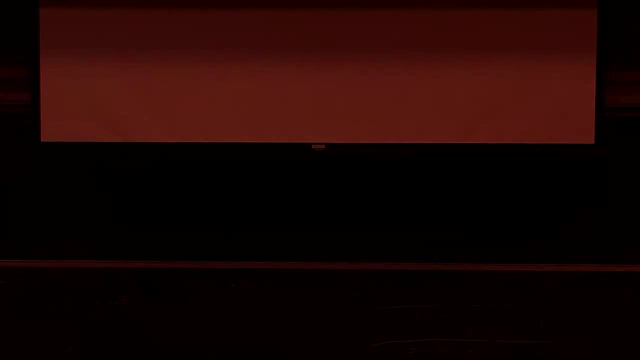 That's just coincidence And this is also- This is also true- The two big Two, GigaPascal. the break in slope happens going from 50 millimeters multi-handle and then, at 25 GPA, you go from multi-handle to diamond cell. 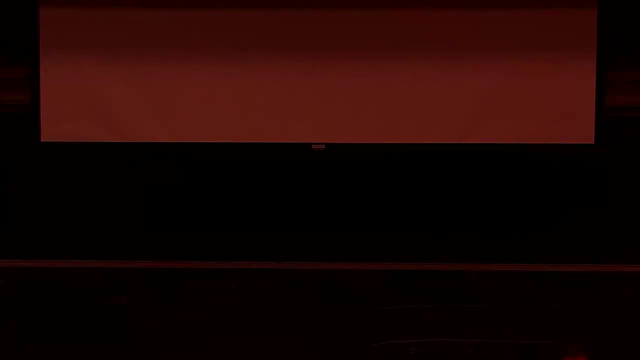 And so I think we should be very suspicious that these large changes in the function, the function for pressure, which is a key variable, a very key variable- we don't have an apparatus that spans, for example, a really critical range like 20 to 30,. 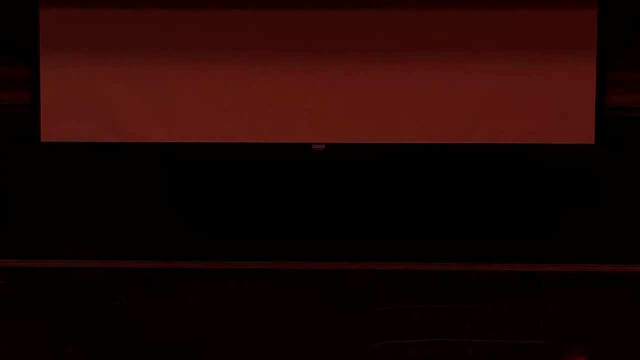 or 20 to 40 GigaPascal. If I had an unlimited research budget, I would try to have such an apparatus. Yep Right, I would like to live in Japan. Just speak loudly, So do you know where these elements sit? 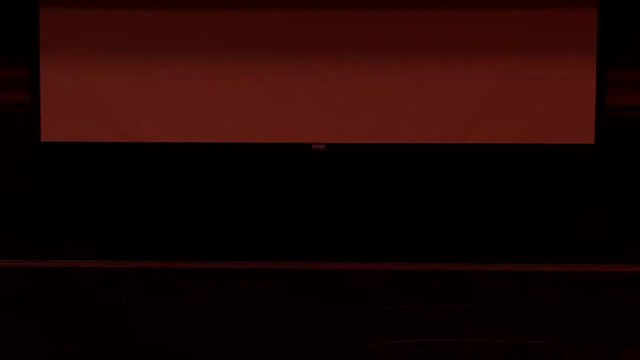 inside a polycrystal material. Are they on grain boundaries? Yes, Do you want to know? Yeah, The osmium iridium ruthenium group in the mantle tend to sit in alloys and Osmorygoy. Yeah, And a mineral like laurite sulfide certainly. So they're mostly in alloys and sulfides. They're usually divided into two groups based on what types of sulfides they like to go into. So platinum and palladium tend to go into base metal sulfides. 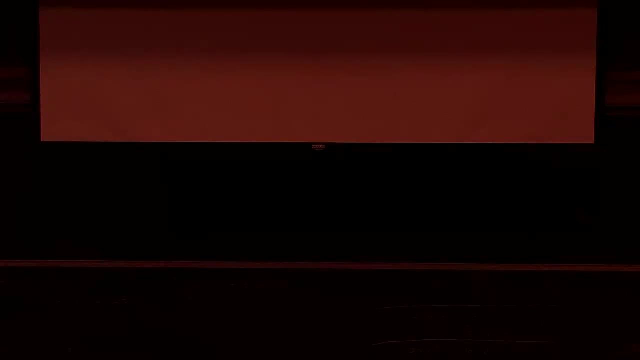 And that's why they behave so differently during mantle melting conditions. So osmium, iridium and ruthenium are typically really compatible during the production of basalts. So they are highly fractionated in crustal production But they're really trace phases. 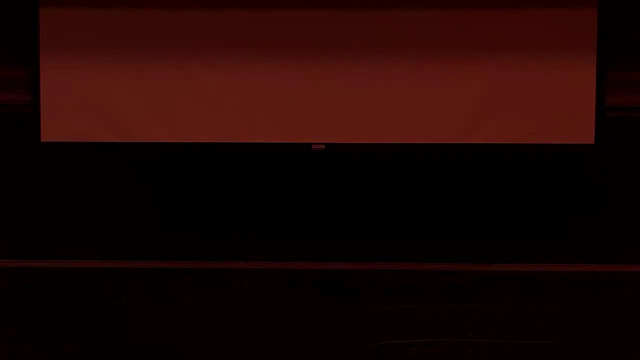 so it's hard to locate them and hard to document them. Yep, So to put the question differently, I guess one way to ask is: doing this type of experiment, is it even on the right track? Yes. Next question: What do you mean on the right track? 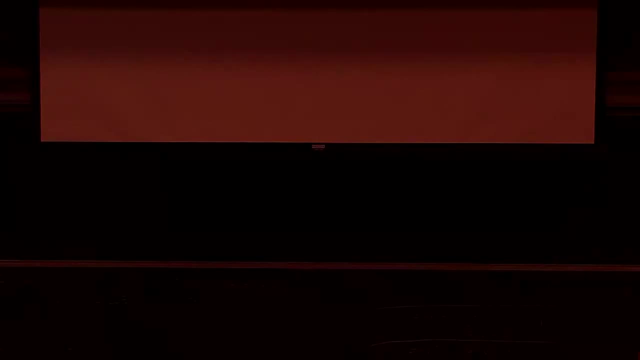 So, you know, is it in the nature really, For what? Later accretion materials, through that kind of thing, that additional experiment become irrelevant? Well, I Explain by later accretion. Yeah, I think the answer to that is. 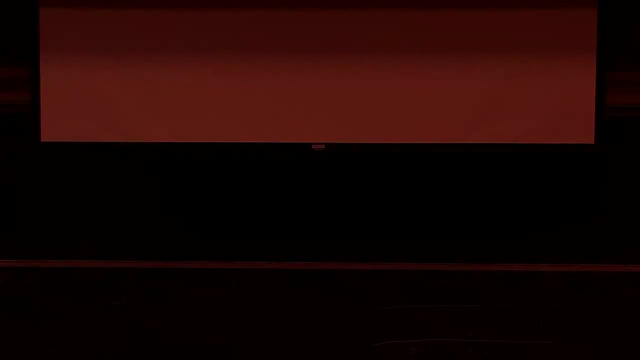 it is relevant. And I think it's relevant because of what I've been saying, which is if you can explain If moderately siderophile elements were set by that process and therefore there was metal, silicate partitioning of all the siderophile elements under those conditions? 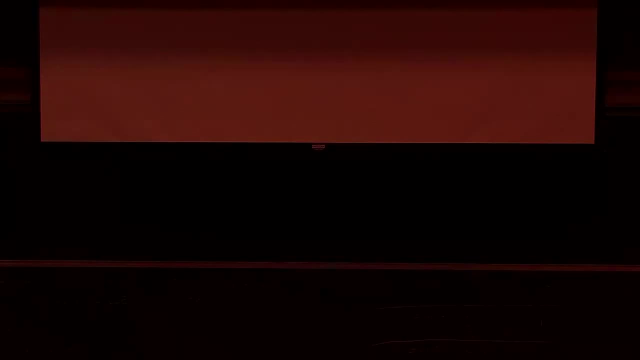 and if the partitioning of elements like palladium is accurately defined by the experiments, then we're missing something, because you can't have later accretion yet an excess of palladium resulting from magma ocean processes For later accretion to really work. 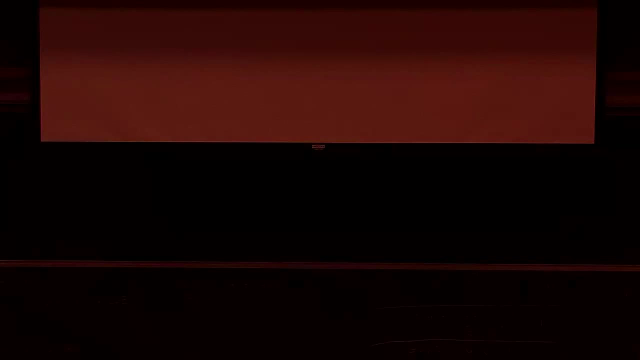 without a perturbance of the chondritium chondritic relative abundances, you have to end up with a mantle with sufficiently sub-primitive mantle abundances that adding material on from a chondritic source just buffers the concentrations up. 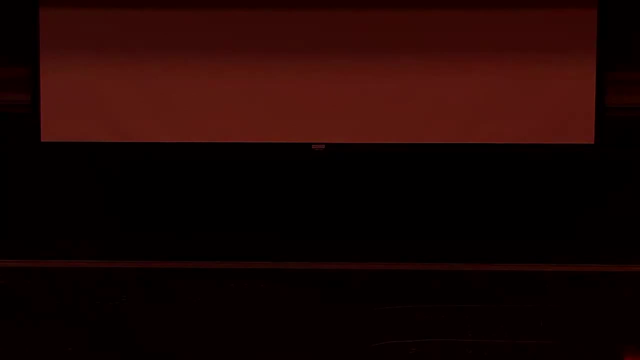 So I think we genuinely do have a problem and it's telling us something. I just don't know what it's telling us at this point. Okay, we're going to have to end shortly, but go ahead. Okay, so you said: 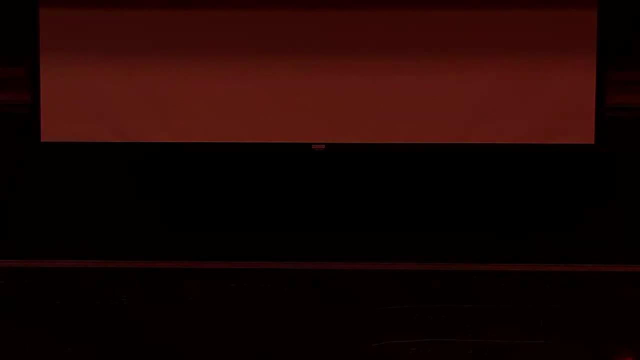 it was surprisingly close to Earth, but the pressures would be much lower. presumably the temperatures would as well. What does that tell you about this? Well, it's a problem from any of the model standpoints. It's a problem from a magma ocean standpoint. but it's also a problem from a later accretion standpoint. In the same proportions. Yeah, What's the assumption about the mantle that's below the magma ocean? What does that hold? Yeah, well, that's, I agree. That's a good answer. I think the assumption is that that would start off with very low abundances and ultimately get mixed back in and therefore diluted. the perhaps somewhat higher abundances that you may have had result from the magma ocean process, But Does it affect the choices of the path? 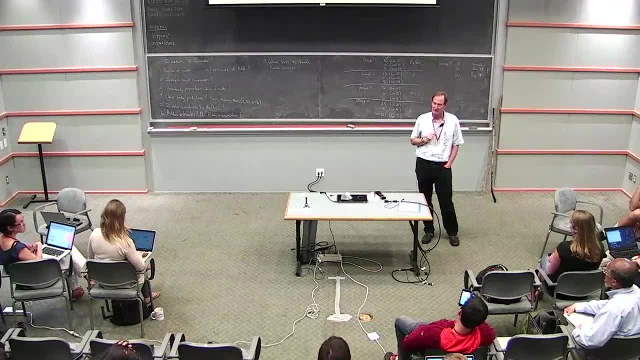 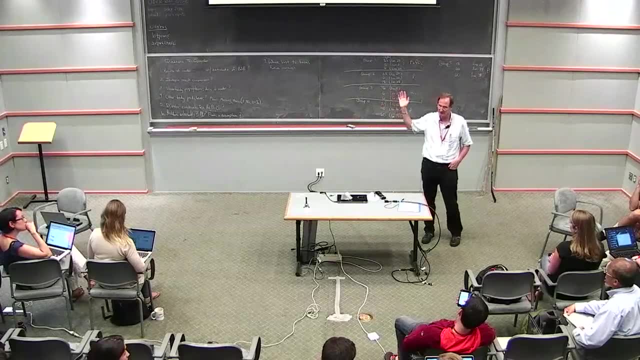 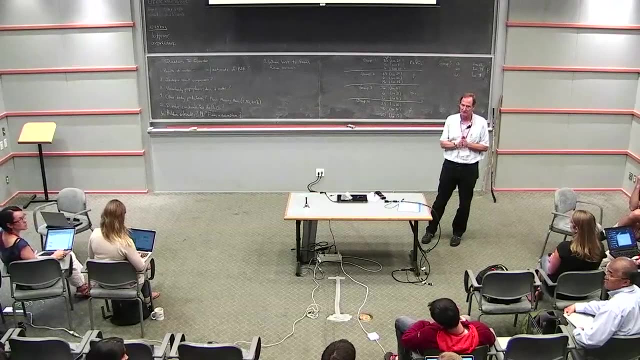 It would, It would. I think it has a bigger problem on absolute abundances, though, than relative abundances, And I personally favor the relative abundance arguments over the absolute, because we have two isotopic tracers. for that, I think we should end the tutorial. 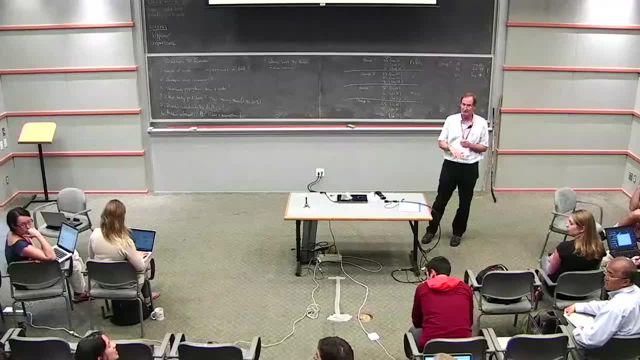 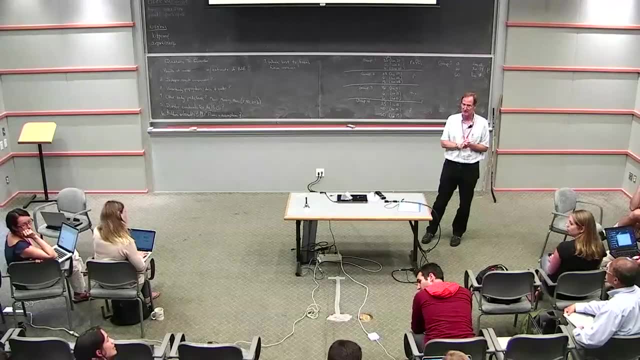 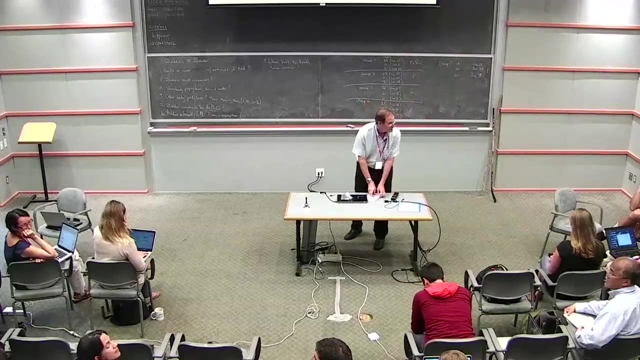 and move on. I have one more question. What about the possibility that the third-file elements are still being exchanged between the core and the mantle today? That's another story. Just something to think about. That's another tutorial. Okay, Who's? 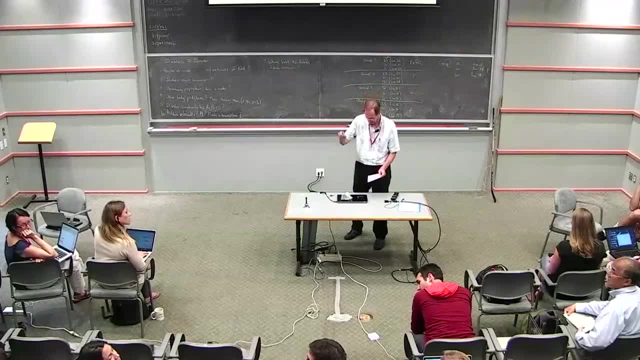 Who's got the follow-up talk? We have a talk, huh, Alan Thanks. 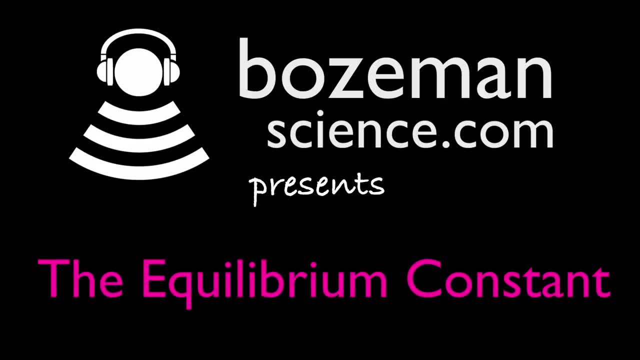 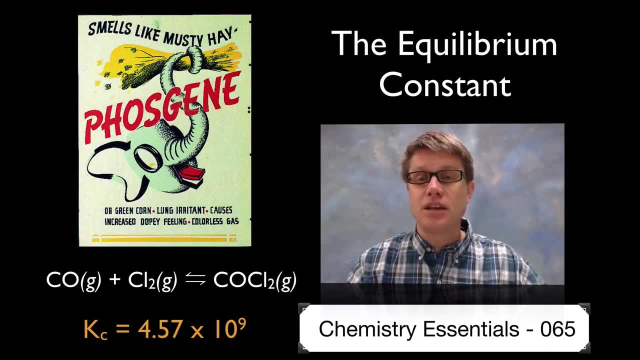 Hi, It's Mr Andersen, and this is Chemistry Essentials, video 65.. It's on the equilibrium constant. A chemical weapon that was used in World War I and killed a number of people is phosgene. Phosgene is created through a reversible reaction where you take carbon.